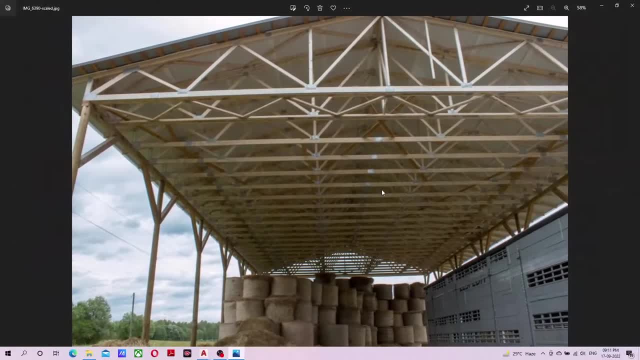 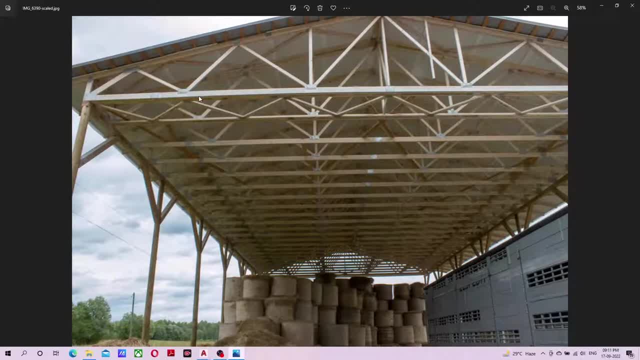 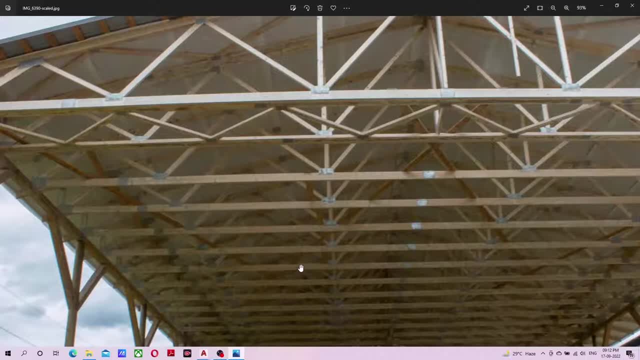 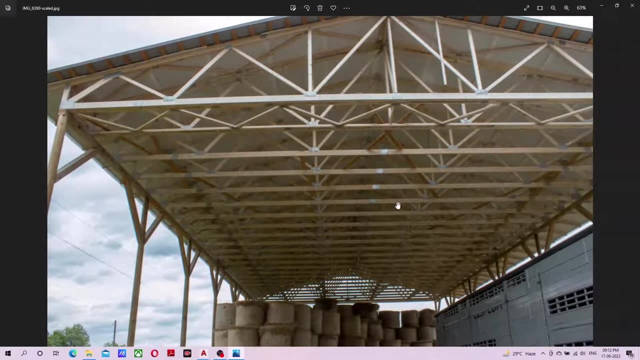 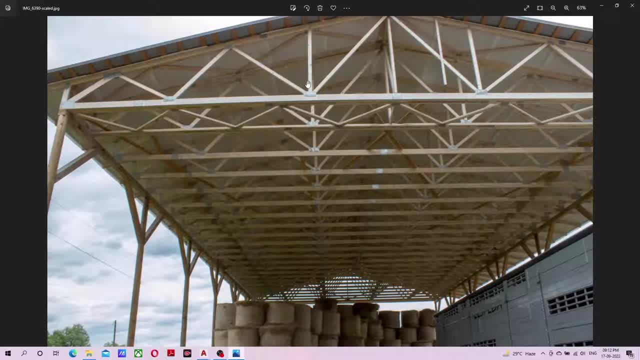 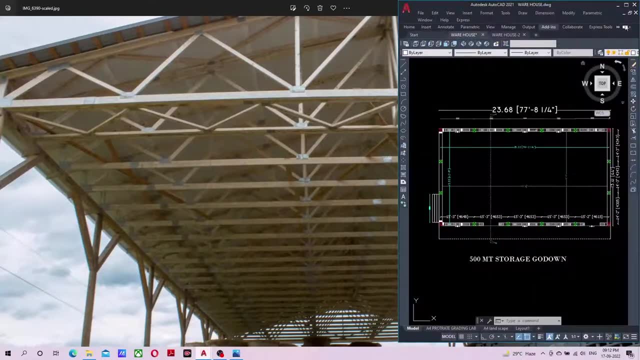 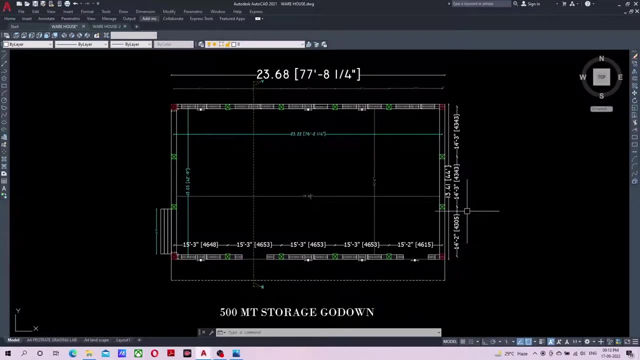 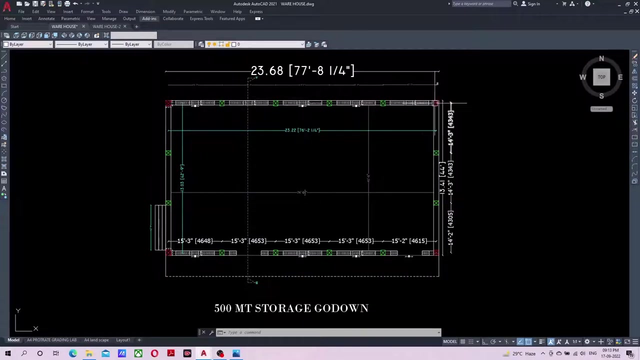 and your tie beam. so this one is your secondary member, so we will design it completely. so I have a plan. this is also a real project, which is: my size is 77 feet and here is your 44 feet. inside it is your one, two, three, four, five, six, six. number of layer of your column. 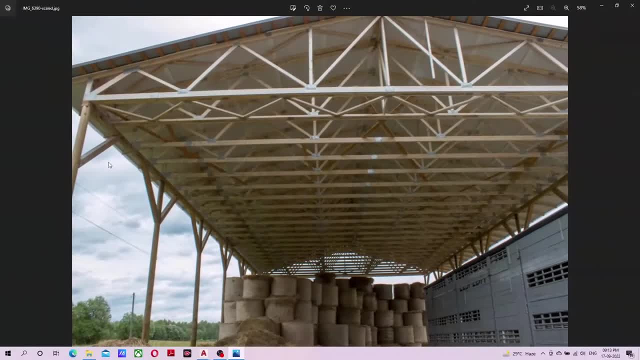 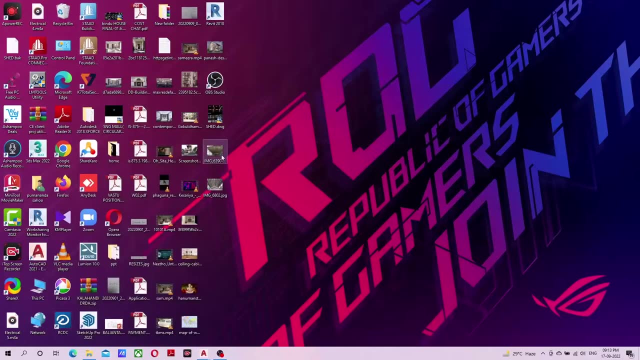 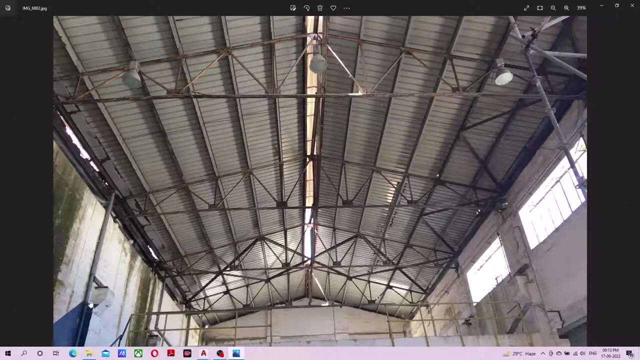 means six number of your trusses will be here like this one truss is done. after that, here is a truss like this here. if I show one more picture here, then see: this one truss is done. this one truss is done. this one truss will be done. and after that, this is its column below: 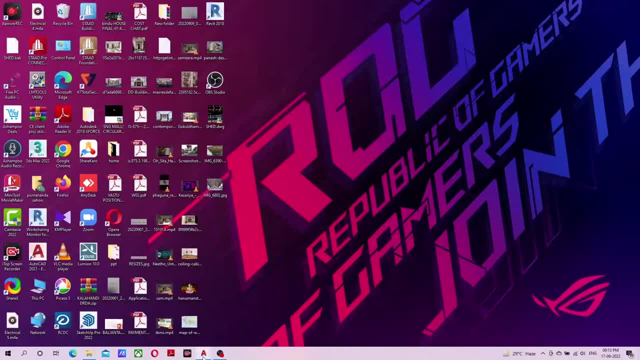 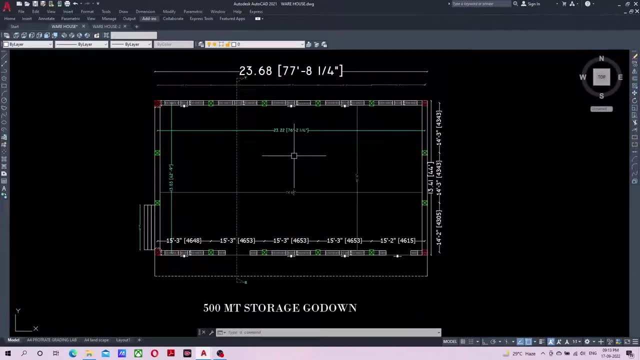 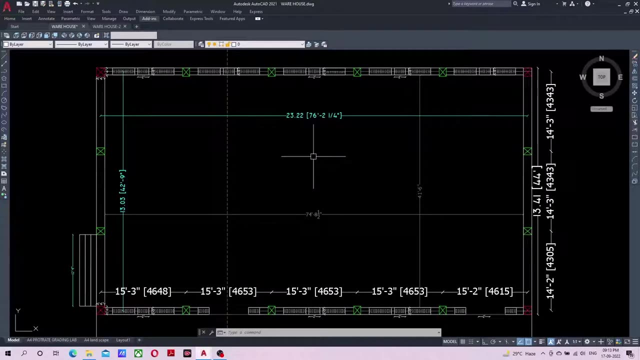 so of the same type. here is a total six number of layer of column, so six number of trusses will be here. so we will draw it at the start. and one more thing I am telling you here: whenever, whatever structure, you will do anything in StartPro or AutoDCard, please do it in millimeter. so I am going to consider. one column will be ISMB 300. it means 300 mm, so if you do in millimeter it will be better. now I will directly startPro software. eft 엄청 often do that, so I have a startPro software. I am going to startPro with the name ofσω новiowikми doku 100, also once in a row. 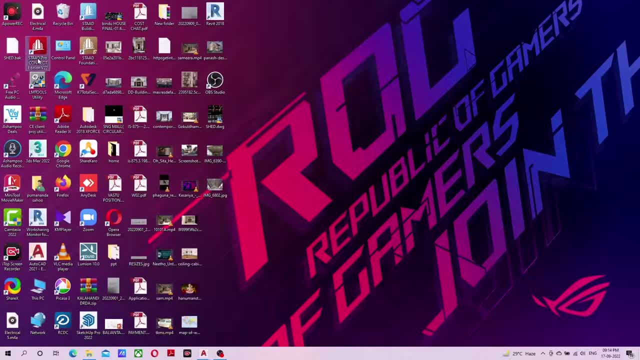 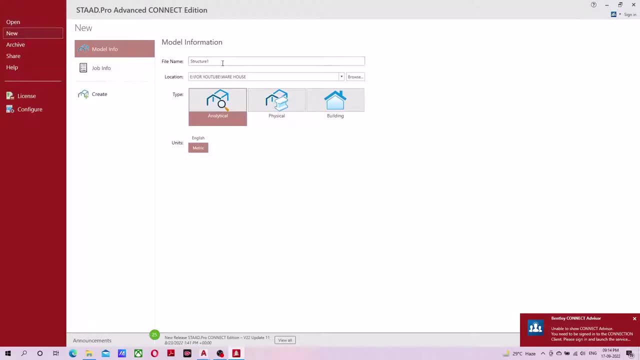 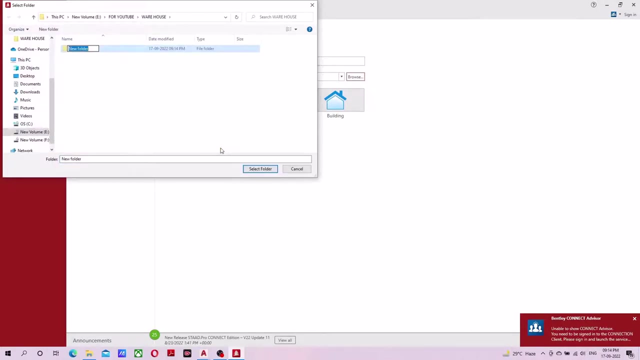 pad pro connect edition version. so here I open it. I continue it after this: here I will click the new option. here I will provide its name, which is still structure. here I will get still structure. after that: here I will browse and create another folder in the warehouse. here I will create a new folder, one folder one only. after that, here I will select the folder. after that you can. 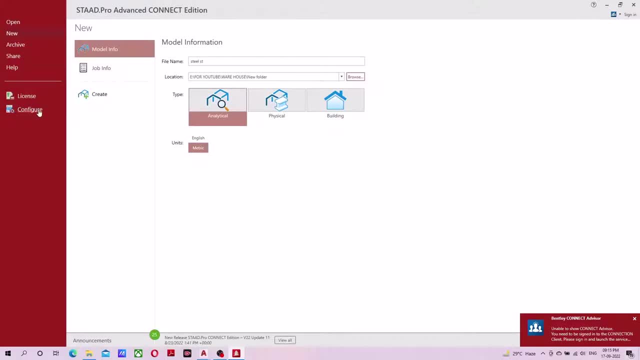 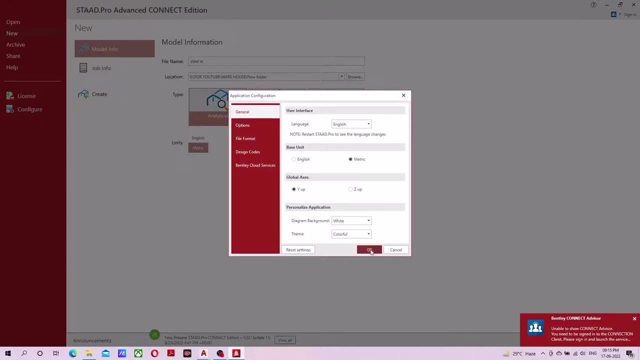 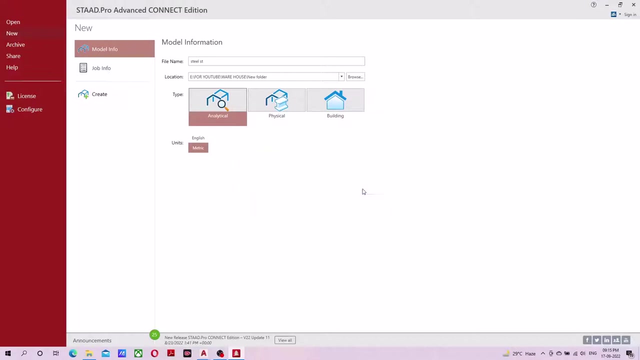 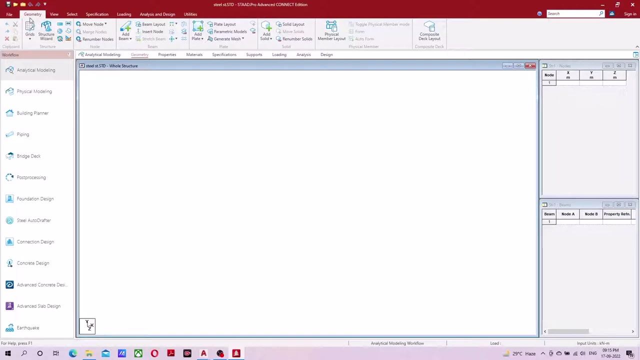 put it in the matrix after the matrix. go to the configuration here and check that matrix should be selected. matrix means your meter, millimeter. ok after ok. here you simply click the create option. after that, here you will do yes after yes. see this, it comes in meter, but I want it in millimeter. so here you go to geometry, select this unit option. here you select Newton with millimeter. 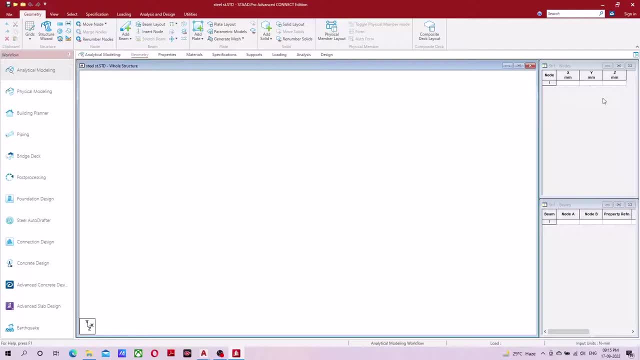 flat. One video is enough forü all types of steel structure. So this process will also happen. Only your model can be changed. So see how do you do that. So now we can minimize the working safe of u withleion is now not necessary to me. later, when it will be necessary, then I will be on it will do it After that. here I make it a. 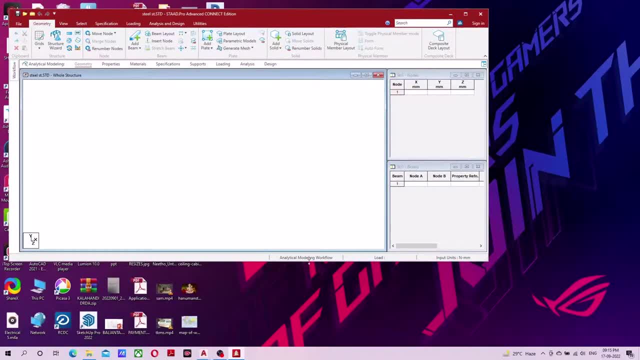 little smaller. I make it in a total video. I divide it into two parts because in one part I divide the sideはい. I take the size of the lifetime auto card and such is got. but now I am dividing it in two parts. I will lengthen this to the maximum of the start. dev интер less. respect the tears i. 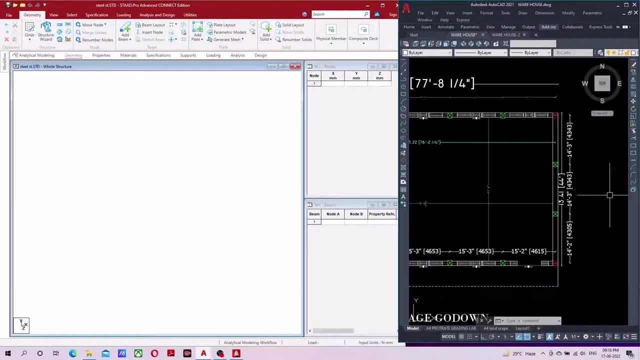 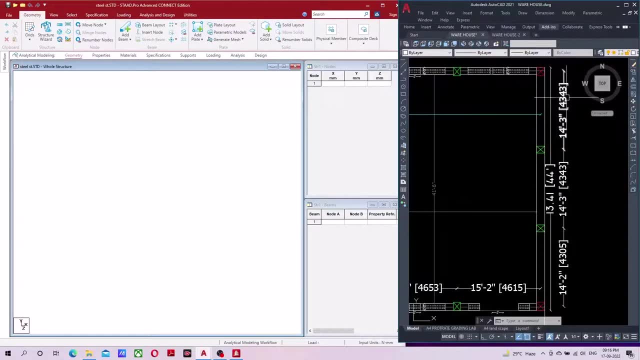 I have to check here, like here: I have to make one truss, this one, after making. I can copy it later, so I will make it so here. dimension is 4343, 4343, 4305, so I take all of them same for now: 4343. 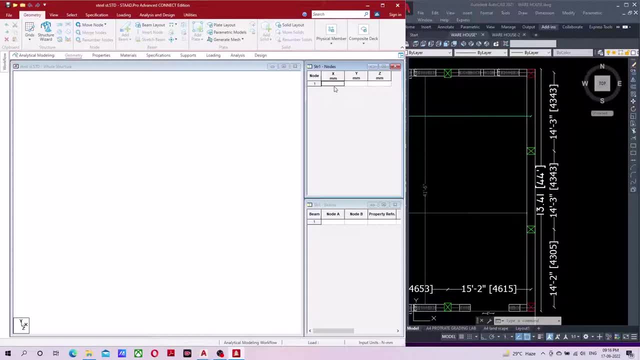 now what I will do. first, after selecting node point, I will enter 0. so this is the first point. now I will copy it in x axis: how much number? 1, 2, 3, 4. I need 4 number here, so how I will select it. 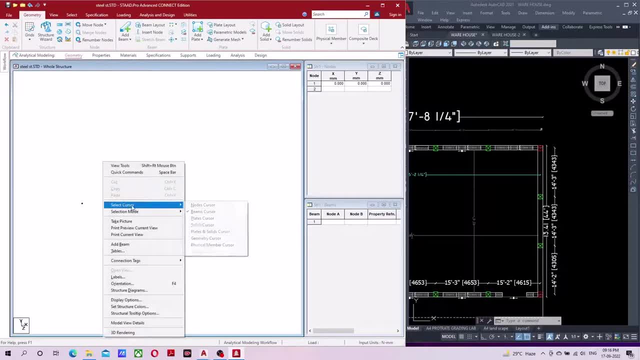 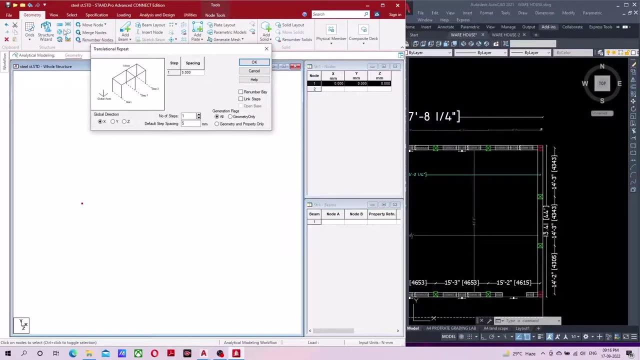 to select, simply right click, select cursor to node cursor, select at a time. I have to copy 3 times, so what I will do directly, I can do transitional repeat copy: see upgrade version. after doing transitional repeat. this was the option here in which direction you will copy. 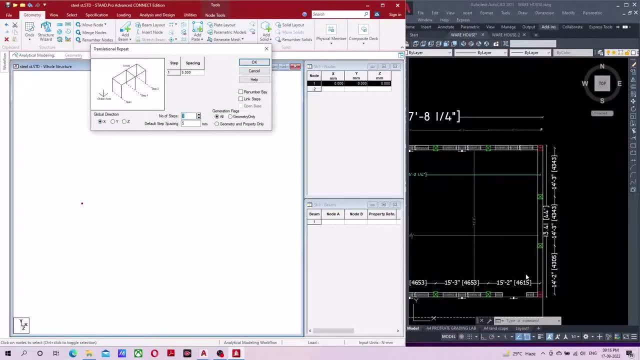 I want in x number of step. how much you will give? 1, 2, 3. so number of step will be 3. now you will give the dimension dimension. here I give 4343. if you want different, then you can change it, but I keep all same. 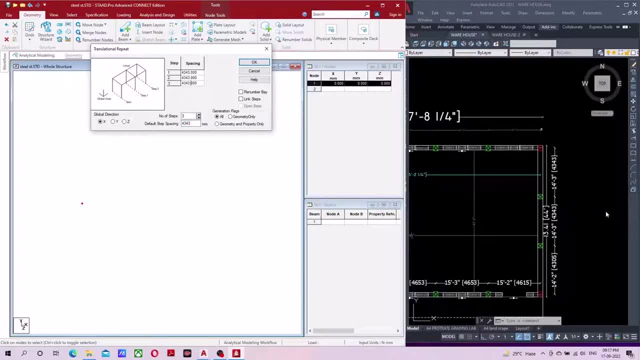 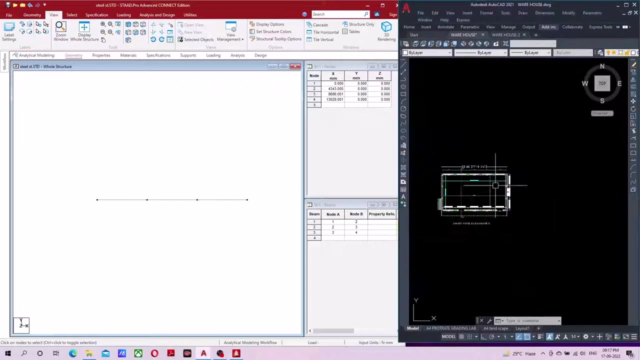 4343. this much keep equal. so it will be better. both sides will be equal after 4343. simply, I will do link step so link will be created in between this connection. so keep it in front view so see my bottom part is done here. after that, this go down. 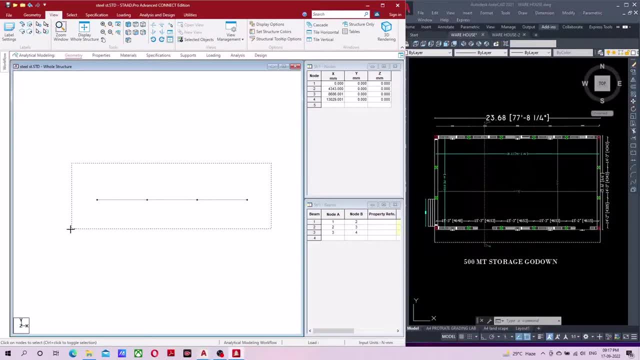 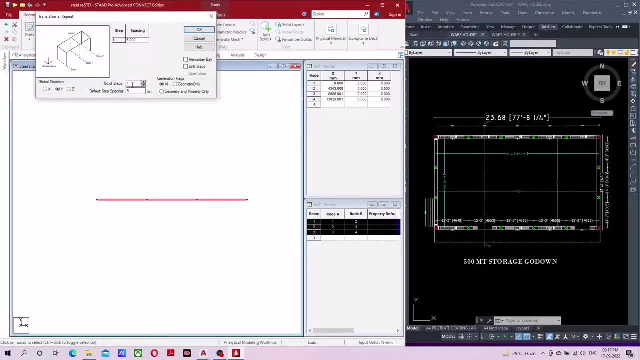 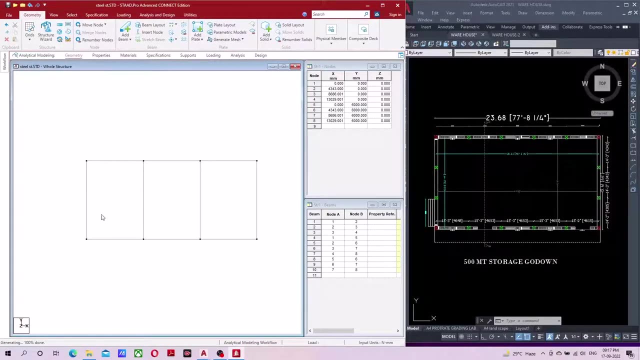 its height is 6 meter, so now I will copy it 6 meter. what will be better, I will directly do transitional repeat. and y axis, number of step 1. and this 6 meter means mm. 6000 mm after that link step after that: ok. 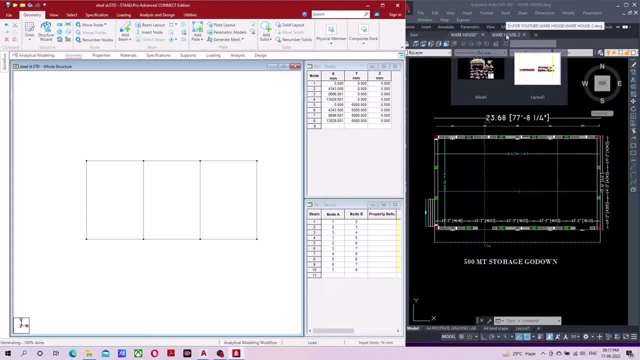 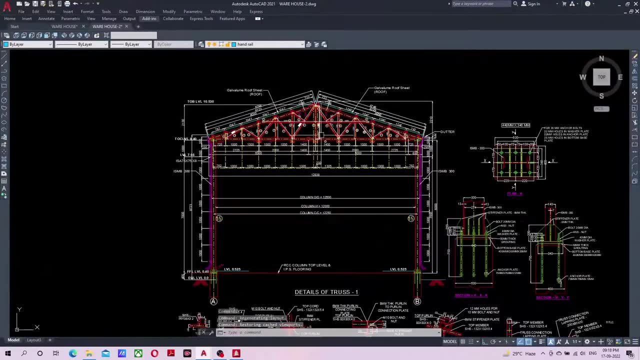 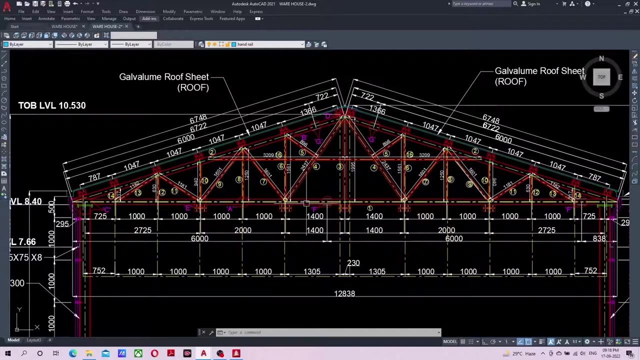 now I am done with this part. if we see one drawing, if we see one drawing in previous I did, if we see its reference. so this truss, I will draw truss of this type which this line was drawn. now I will provide this height and angle. 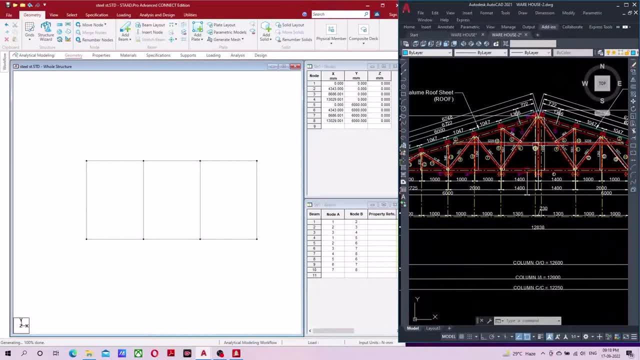 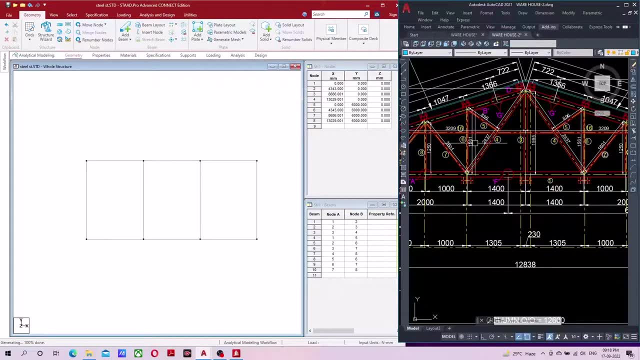 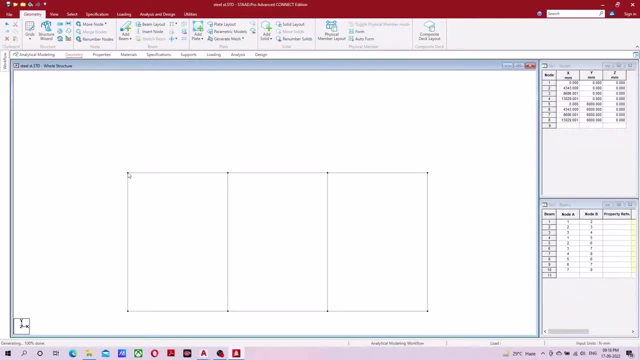 so I am going to provide something like this. so see, if draw something like this, then I have to provide this height. this height will be provided. so the height, how to provide this height, the concept of providing height. the calculation is total length of the span divided by 6. 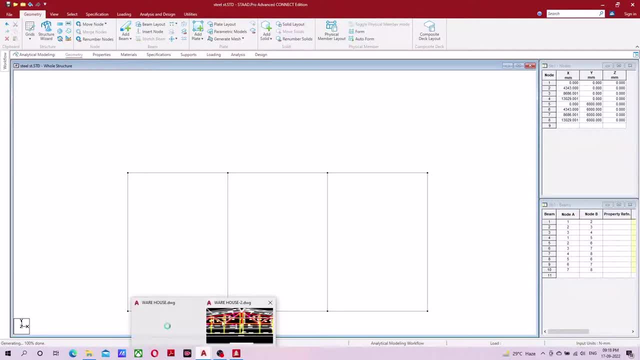 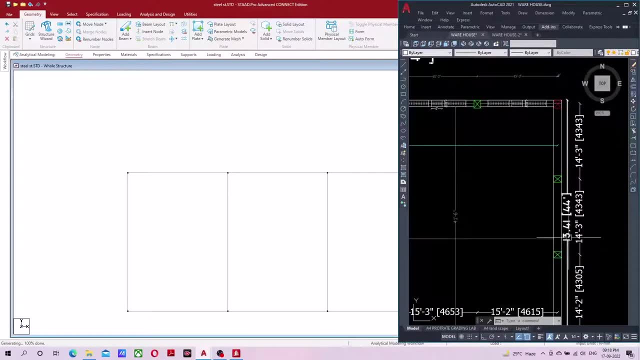 so its total length we can check in autocad. total length is this length: 13 meter, approximately 13.41, 13.41 meter. I will turn on the calculator calculator. I will take round figure 13. so 13 divided by 6. so here: 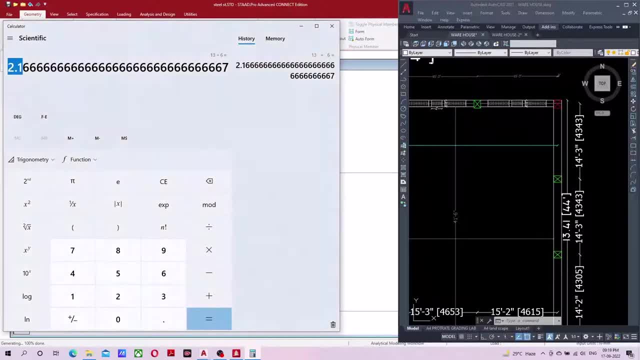 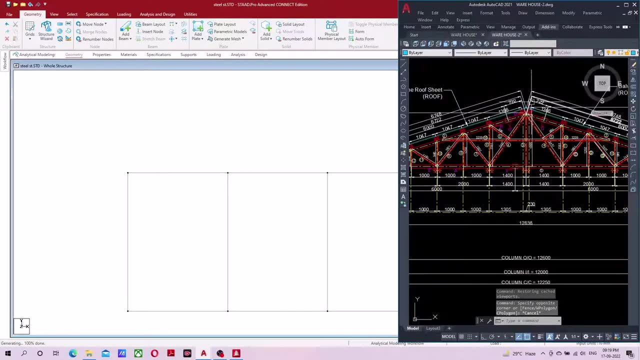 your 2.166 means 2.1. the height of riser will be 2.1. this height, this is called rise. its height will be 2.1. so from here I will copy 2.1. so I need a node point. 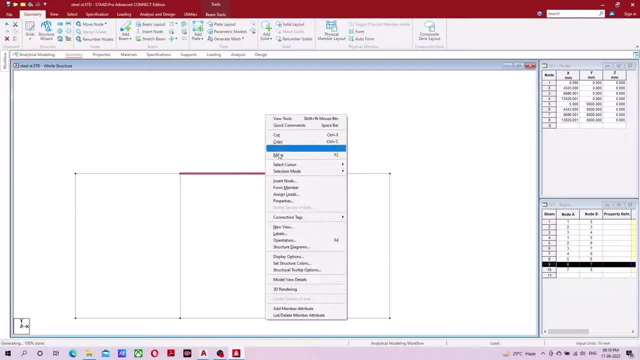 I need a joint point to bring it. select it: right click on mouse button. then meet point. then ok, now I will copy it. select cursor right click. select cursor node cursor ctrl c for copy, ctrl v for paste. give the dimension 2.1.0.0. 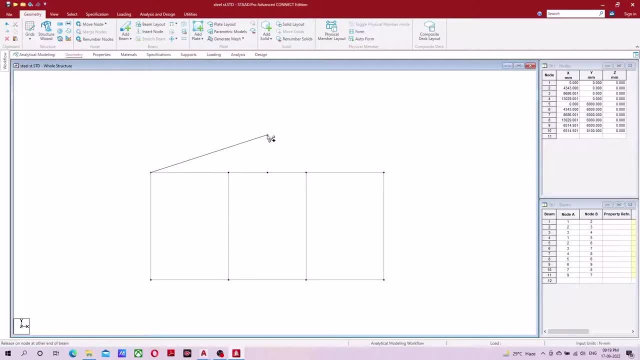 which I have calculated. now join it like this: after joining, we delete one side. why I am deleting: after completing one side, we will mirror it like this after that, what I will do now: I will extend this member, which is called apes. as you can see here it is extended. 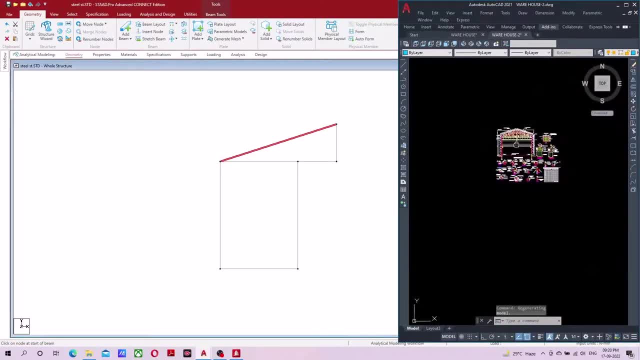 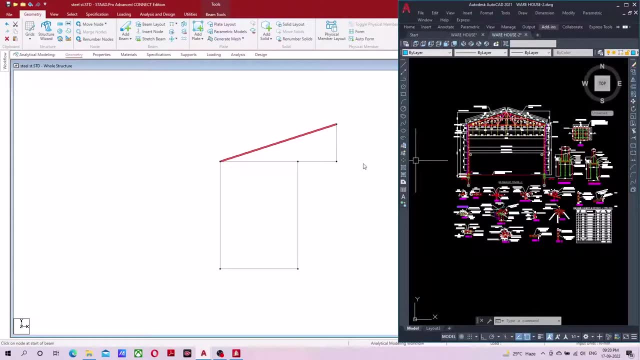 after extending here it provides gutter. this is a drawing, total drawing and start profile. I can download it from description with minimum price. I will show the drawing if you want, and in start profile format. you can go to description and download it for the practice purpose. ok, so now. 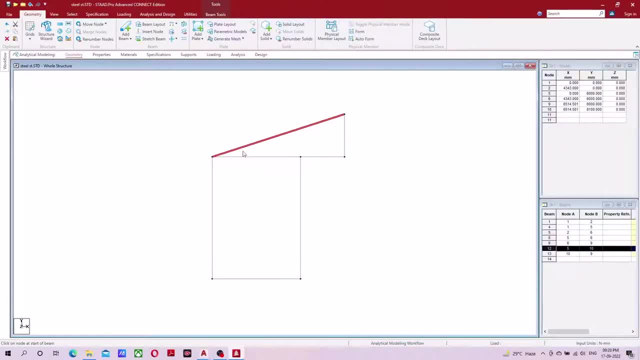 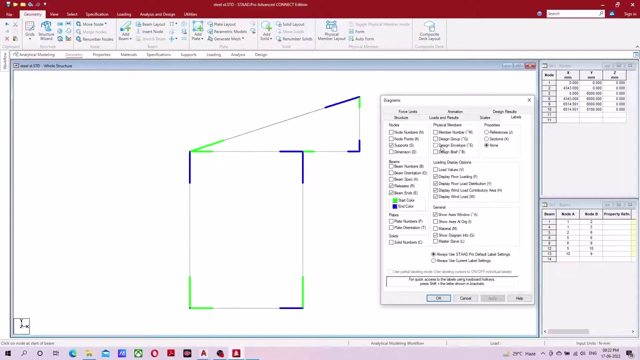 this apes, I will keep it 500, I will extend it to 500. so how will I do? simply shift e, shift plus e e for egg. press shift e it will show some color. now right click on mouse button. here we will select level. here you can see: 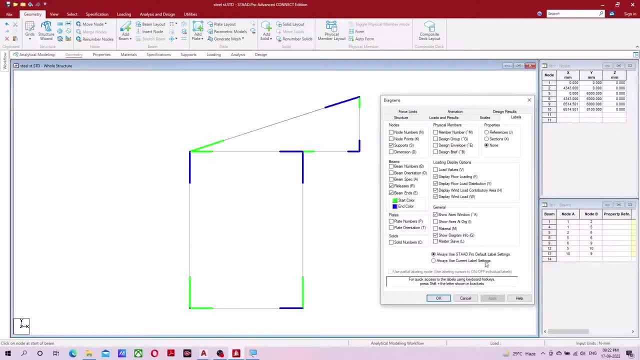 two colors. I will zoom it here. you can see two colors. one is your start color, green color- and blue color is your end color. here it will extend in start color means it will extend in starting color. so you can check it. after checking I will cancel it. 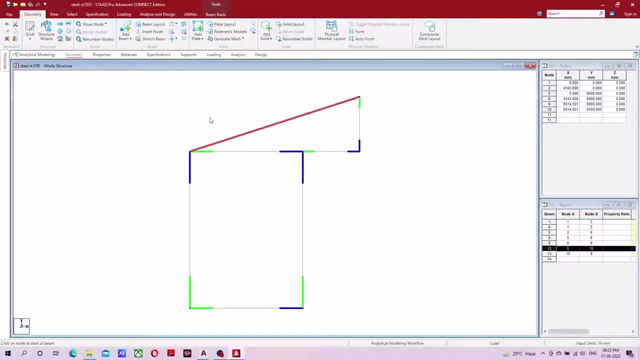 by default. green is your starting color and blue is your ending color. now I will select this member. right click in the mouse button. there will be an option. after selecting, there is an option. go to geometry. there is an option of stretch beam. click on it after that. 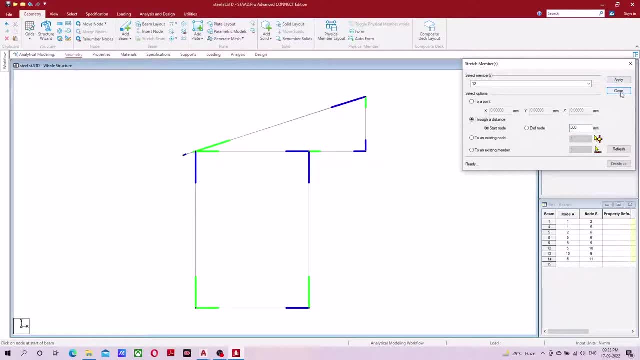 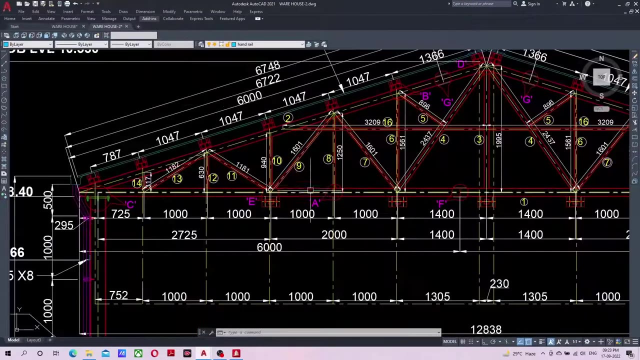 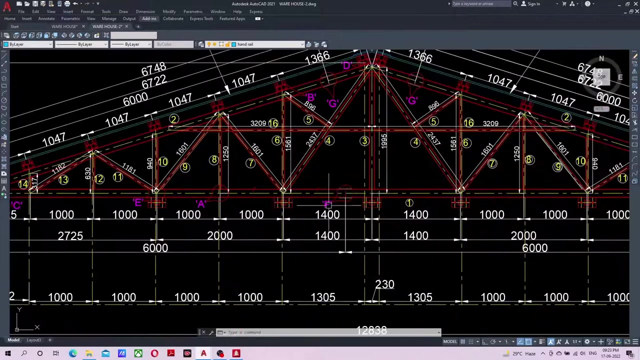 provide dimension, I want 500. after that simply apply: ok, see it extended in starting color again. shift e color is removed. after removing, what will we do? if I check, see here one perlin to second perlin: dimension is 1 meter and starting one is 1400. 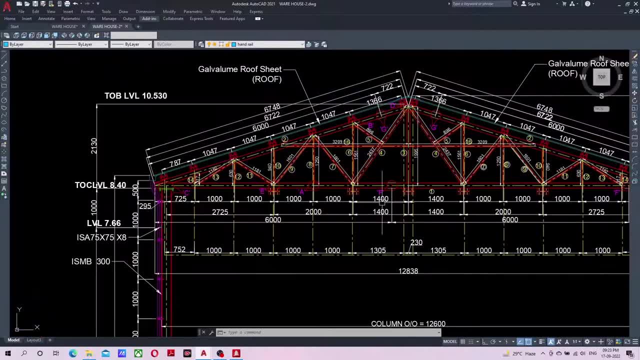 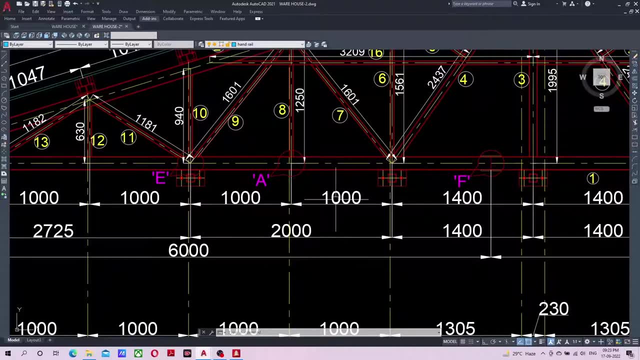 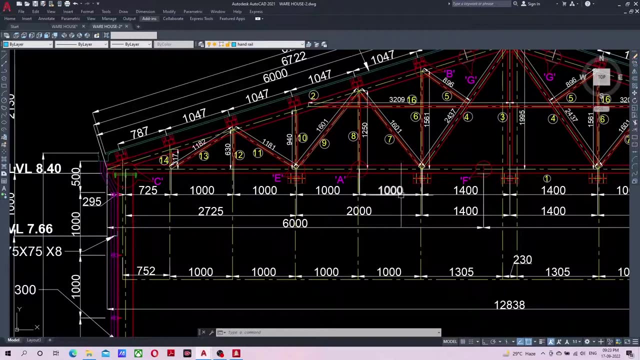 this is a standard. you can follow it, and dimension can be different, like this: 100,600,500,700. you can take it. it is not necessary. it depends on the length of the span. if the span is more, then reduce the distance. here it is not more. 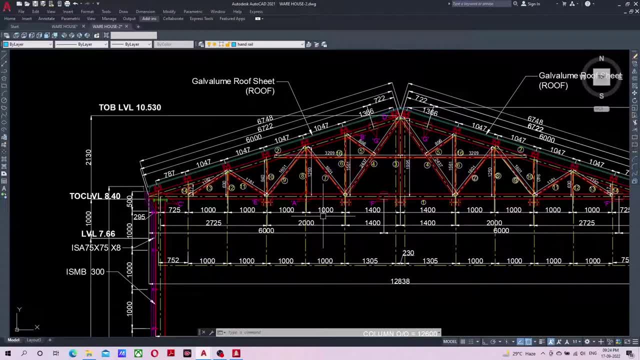 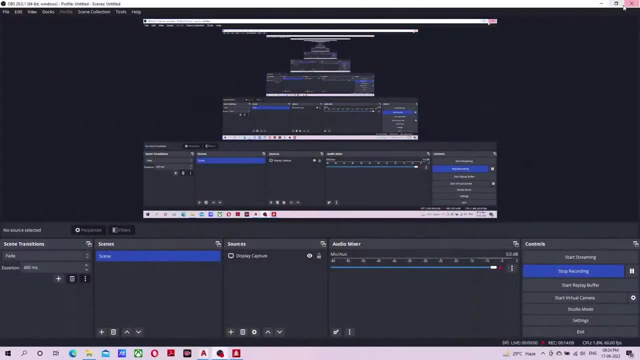 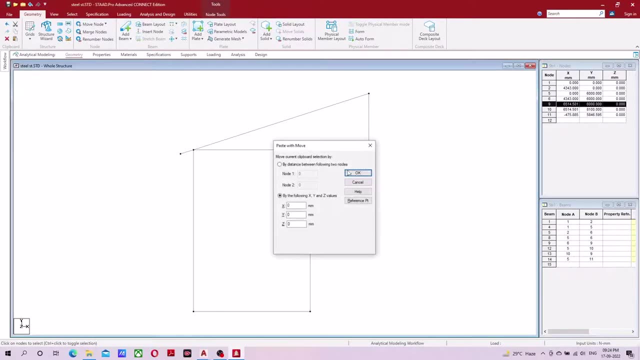 it is 13 meter only, so I have taken 1 meter. that is enough. it is not necessary. it is enough. I will make a copy. right click, select cursor. after select ctrl C, ctrl V in x axis: see in reverse direction. copy will be minus after that, ok. 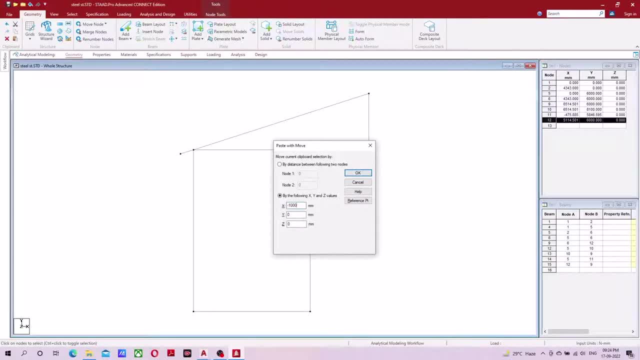 now. I will copy it: ctrl C, ctrl V. I will copy it: Ctrl-C, Ctrl-V, X, again minus 1000. Copy it like this. You can also do transitional repeat, but I copied it here. No problem, if it happens again here, it will probably happen. 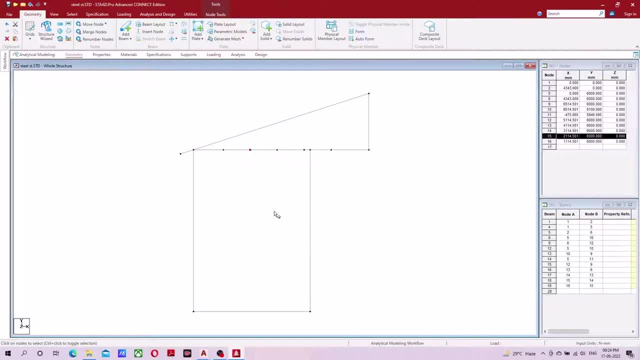 See, this is your 1000 Rest where it happened here. we will check it. So the rest one came here: 1114. That is okay, no problem. so this is my part here, Completed here. after completing this part, if we 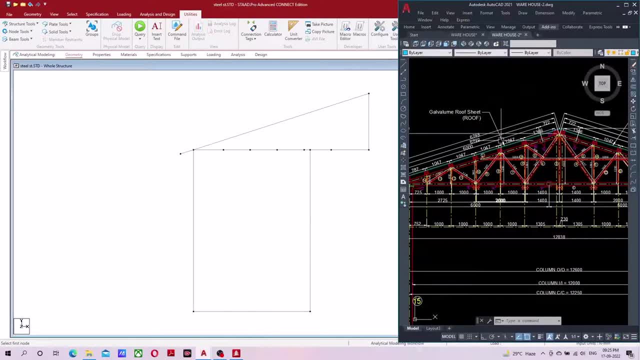 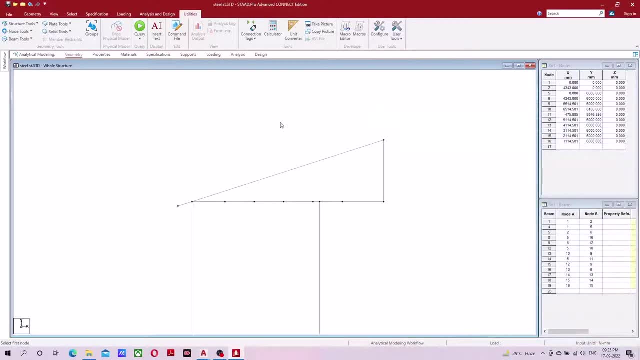 If we check, then what is here? it has to join vertically upwards. It has to join vertically upwards. So what will I do to join it vertically upwards? now I will do select cursor. right click. select cursor to node cursor. I will select this node. 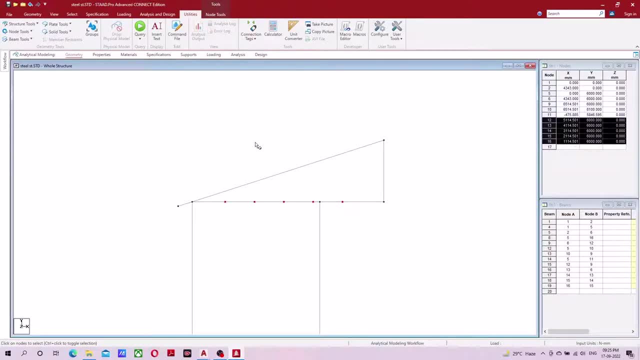 Which I have to join, I will repeat it: transitional, I will copy it upwards. which should be drawn above it, Which I had provided in this dimension, 2100, so more than that I will take 2500. I am doing it. geometry, transitional, repeat. now you see. 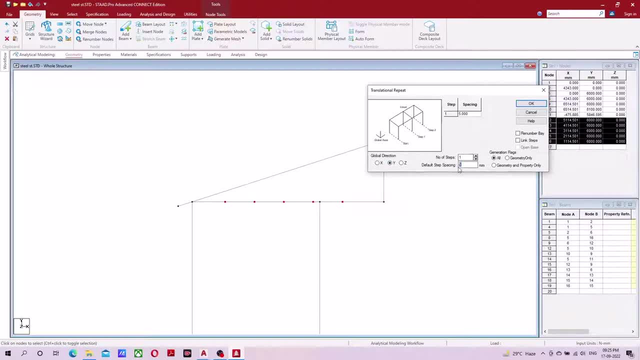 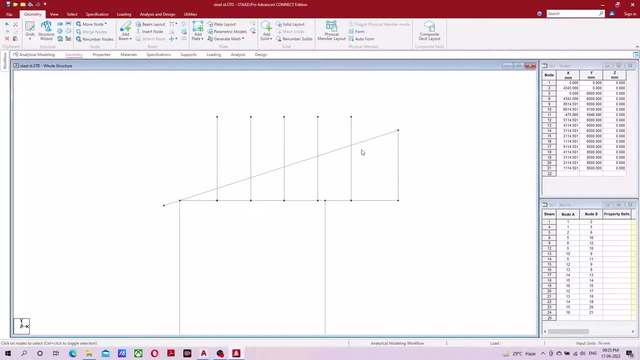 Y axis, number of step 1,. this will be your 2500 Give link step. after that click ok, this is some line here Now, in between this line and this line which is your Connection, see here if I insert a node point, if I intersect it. 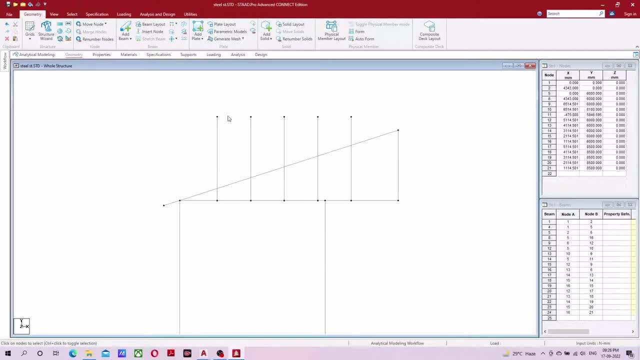 So the node point will be inserted in between it. it will be divided into two parts Later. if you want, you can delete it so as we have selected it. Press control. I don't want this one. I want this much. after pressing control. 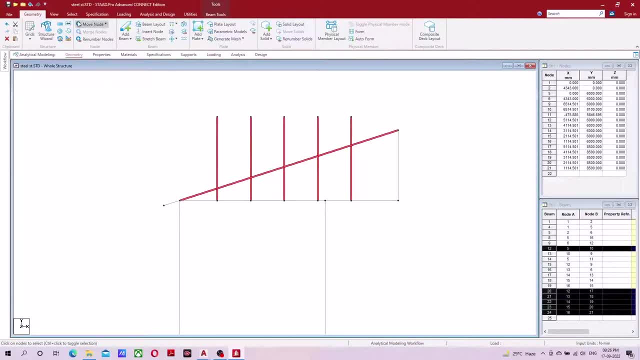 After that you go to geometry. after that This option is visible here. see this option properly. This option is visible. this option is called Intersecting option, so you select this option. after selecting Here, click on intersect. selected beam, after that here. 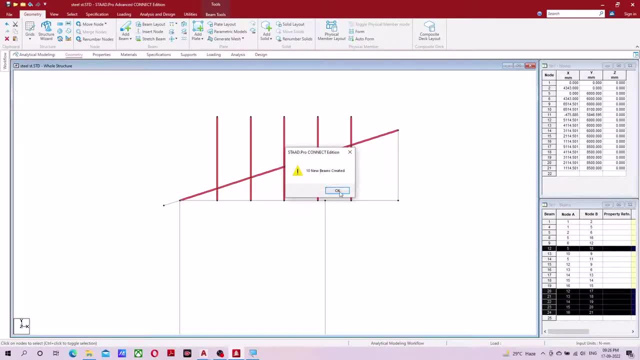 You do ok. after doing ok, 10 new beam created. ok After that. if you want it, you can do it From here. If you want it, you can do it like this and delete it. See no node. you delete it, delete, enter. enter. 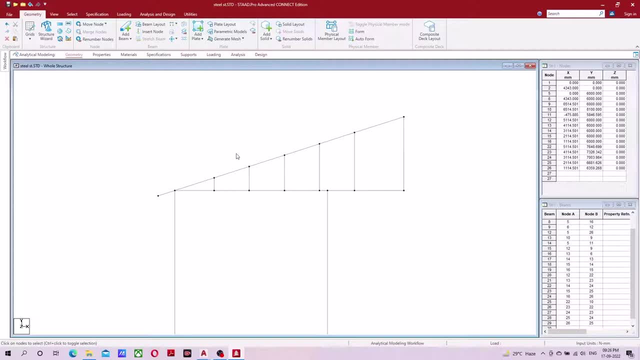 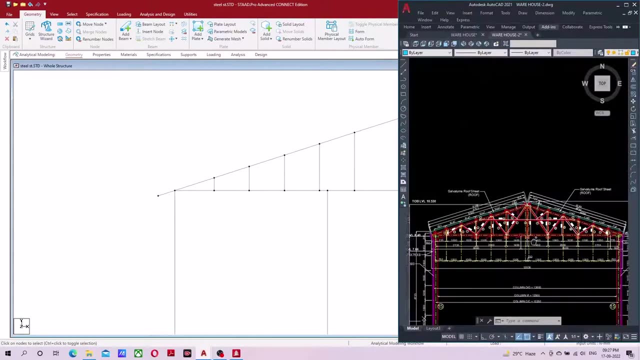 You do it. so this is my delete now What I will do after deleting. I will check the drawing. So see here. now there is such a connection, this type of connection. There is such a connection, so I will draw this connection. 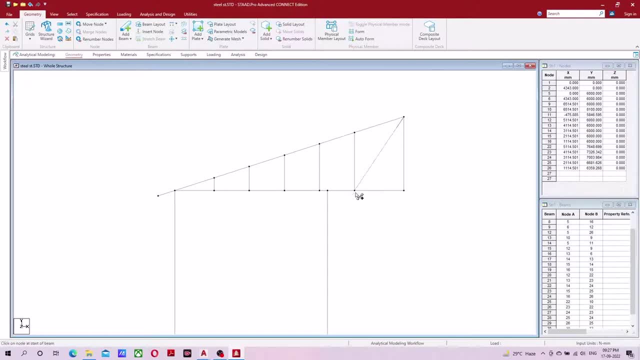 So here I took the argon icon first, I joined from here. after that I give such a connection here. this is called secondary member. Ok, this is not fixed. there are different types of secondary members Which you can follow from the book. which type of? 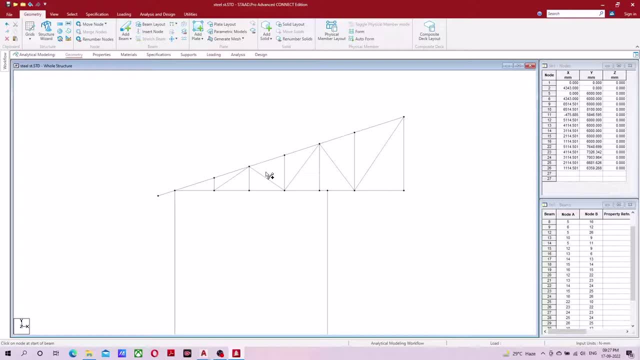 How it is provided in the angle. but basically you can take this, this is no problem. This is called how we trust, so you can take it accordingly. What is the type of trust? if you want to know that, Then you comment. then definitely I will make another video on it. theoretically, 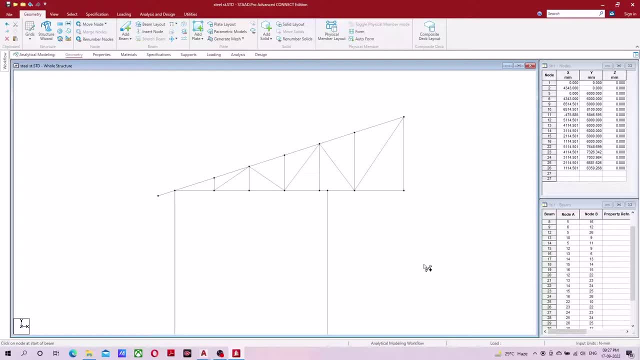 What is the trust, what is needed in it, and How much trust is there? I will explain that then. please Comment, if you want it. so that's it after that. Now, what will I do? there was a connection here. if we look at the drawing. 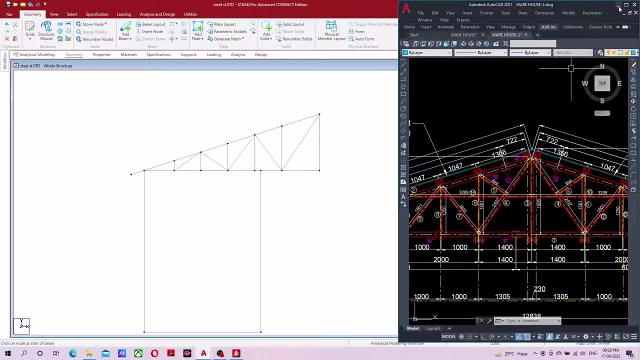 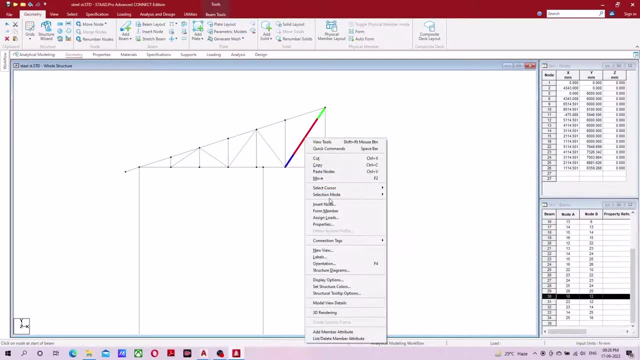 So here I need another connection, because this span, The length, is too much. so what will I do? simply, I will right click on it by inserting a note. By inserting a note, I will insert a note point at the midpoint. I will join it with the argon icon. so see, my part is complete here. 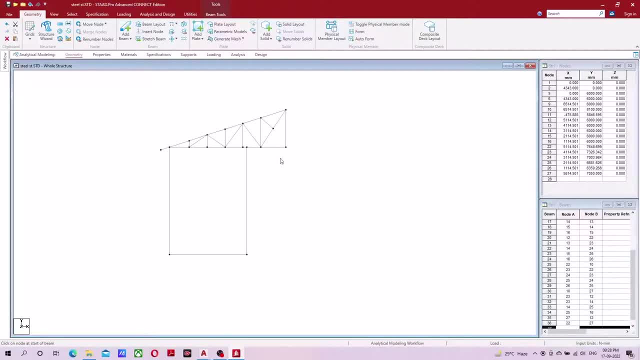 After completion. what will I do now? I will mirror it to mirror. I have selected so many, after selecting which axis It will be mirrored. see here: mirror will be mirrored on the x axis on this side. So here you click on the mirror. this is the mirror option if it is copied in x. 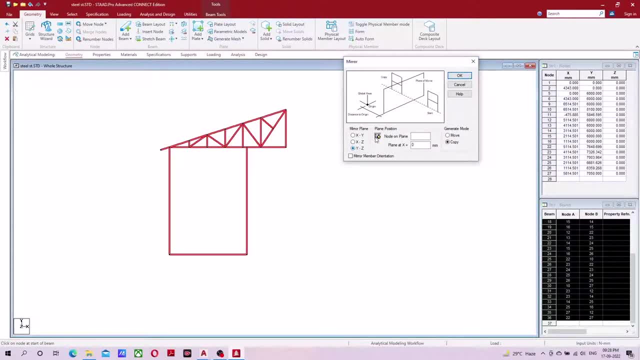 If it is mirrored, then select it as yz- its opposite. after that, This point is the peak point, which is selected by the center point. select it After that. you can take this too. you can take this too. click on any point. 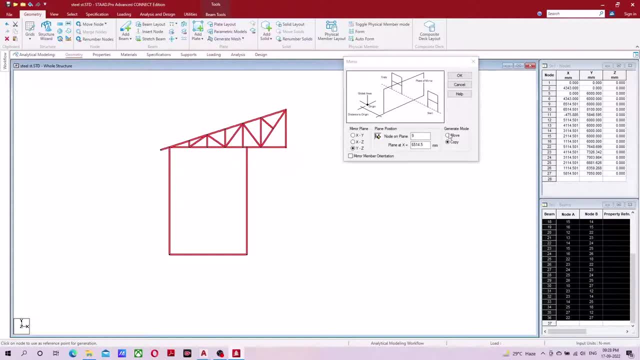 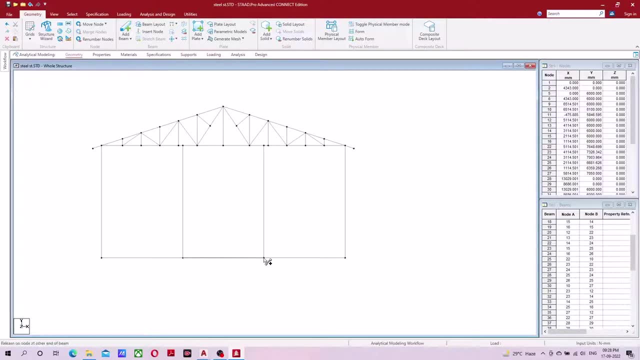 Because this is the center. based on this, it will be mirrored on this side copy. Ok, see, your mirror is done. after that, I will join this lower beam, Which will be my plinth beam- plinth beam. So this much part is completed. after completion: 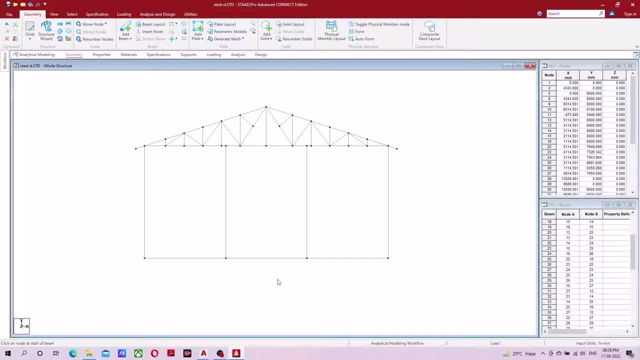 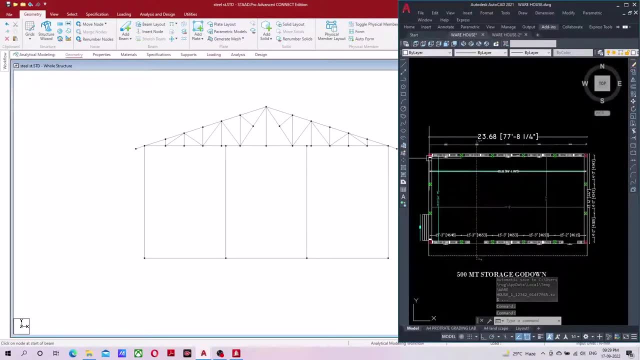 What will I do now? this one truss is completed. so if I, If I look at the drawing, then how many number of trusses are here? I had counted 1,, 2,, 3,, 4,, 5,, 6,, 6 number of trusses are there and its 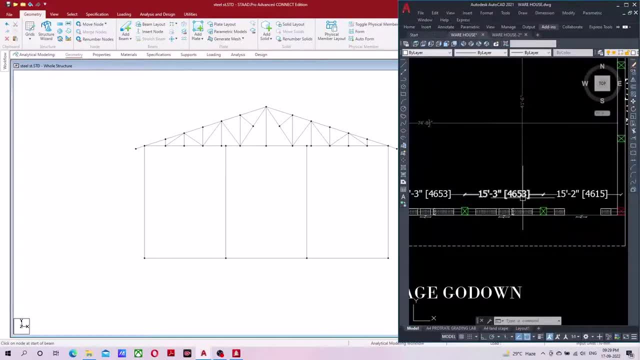 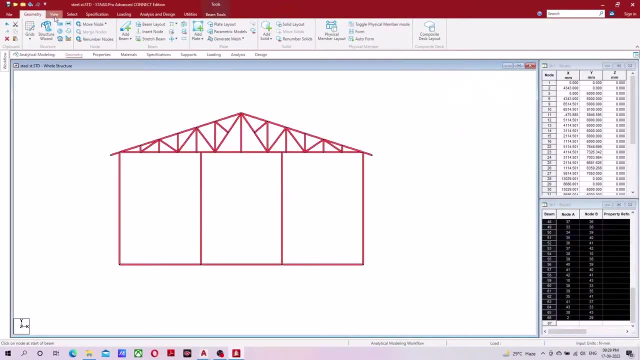 Dimension is given your 4,, 6,, 5, 3, 4, 6,, 5, 3, And the first one is a little different, so I take all of them the same. Now I selected it, I go to the isometric view view isometric. 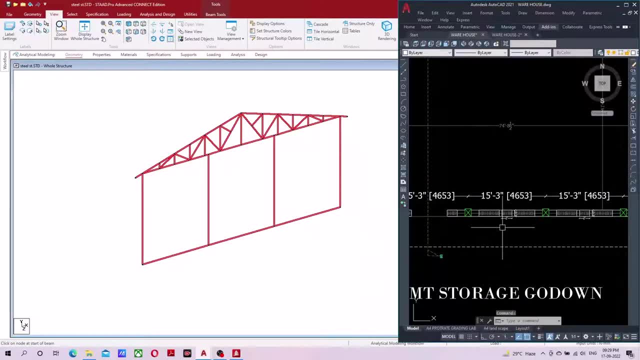 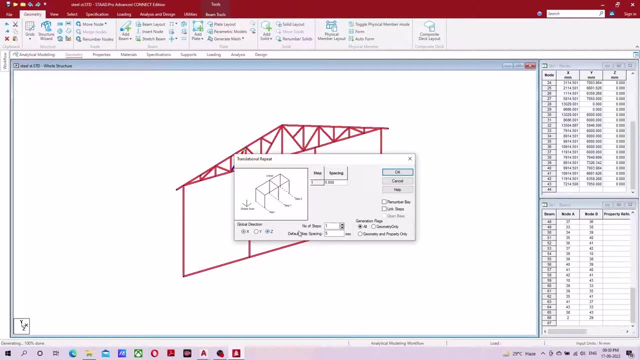 Yes, 4, 6,, 5, 3, 4, 6, 5, 3. So to select this, I go to geometry. Transitional repeat z-axis. number of steps will be here. how many number of steps? 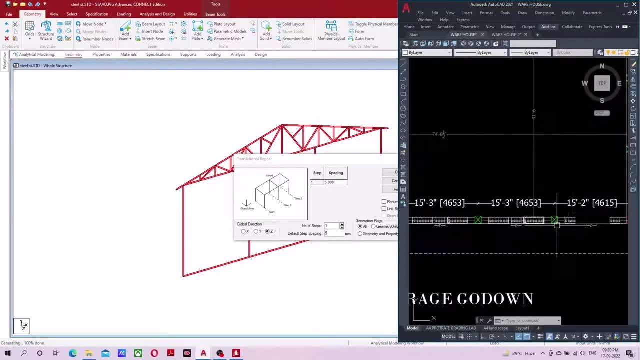 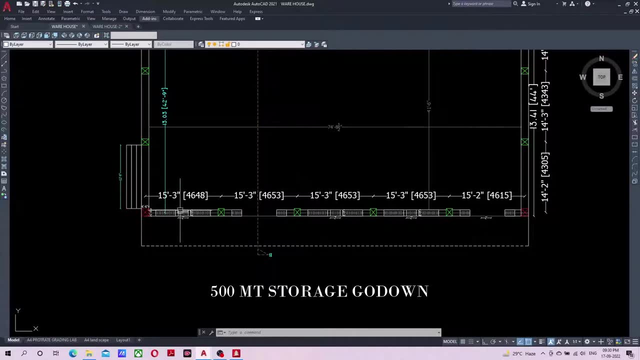 Will be there. here you count number of steps means spacing, As if I see here, then the number of steps will be 1, 2, 3, 4, 5, in between spacing I want 5 spacing, 4,, 6,, 5, 3, so here the number of steps will be 5. 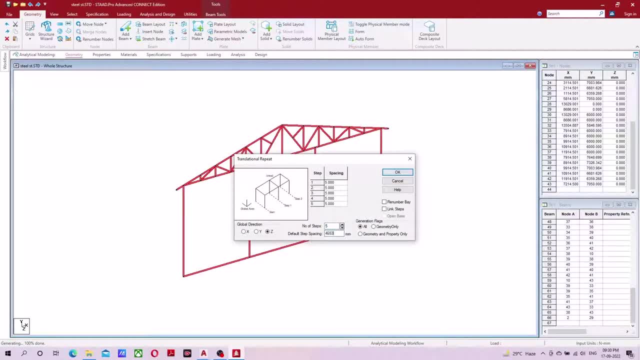 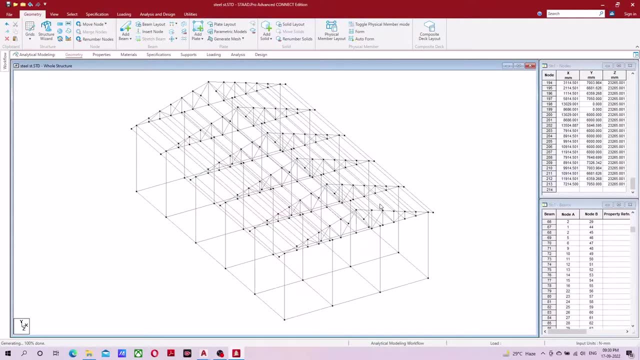 Here 4,, 6,, 5,, 3,. after providing Here all the changes have been made, your 5, link step after that. simply I have done here, so see this much is completed here. After that, if we check here, then see: 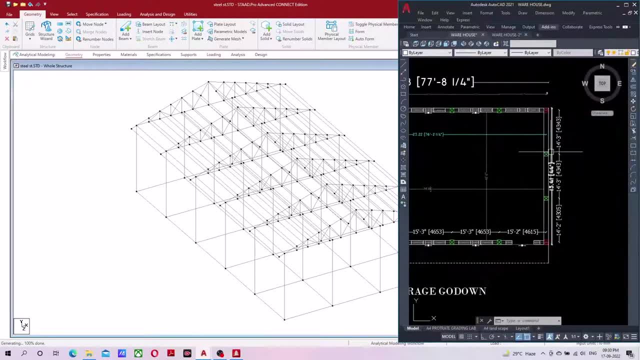 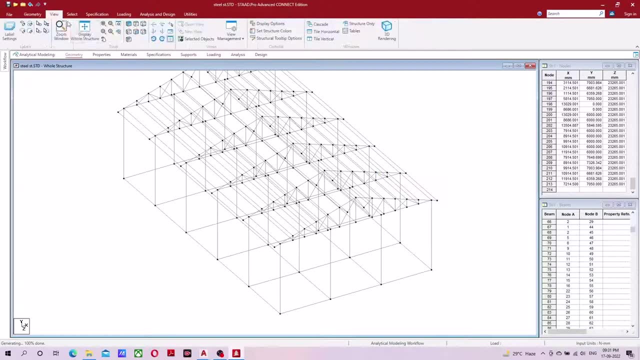 In between, you do not have any column. there are 2 extra columns in the starting. There are 2 columns in the ending. there is no column in the middle, so I have to remove it. How will I remove it? first, you go to the front view. after coming to the front view, 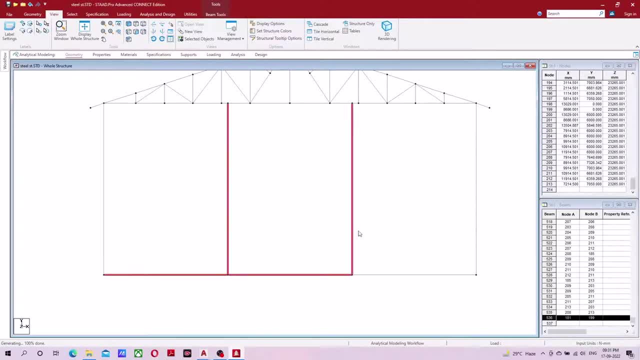 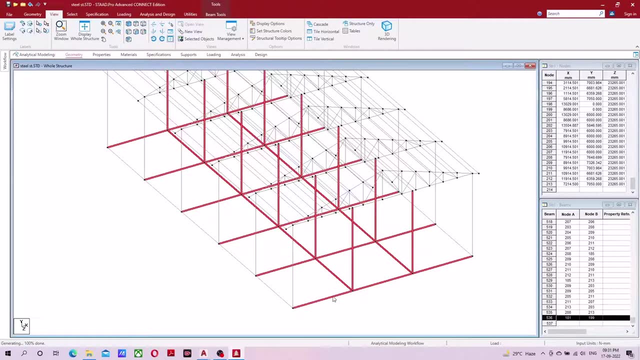 After that, select all this, what is visible to you. select it like this By dragging. now come to the isometric view. Unselect the first one, press control and select the first one again. So see, this is selected. similarly the last one too. 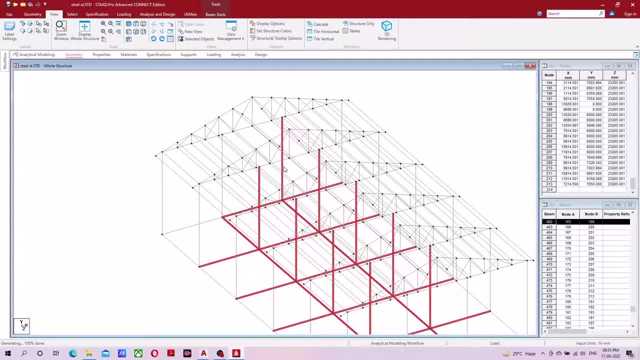 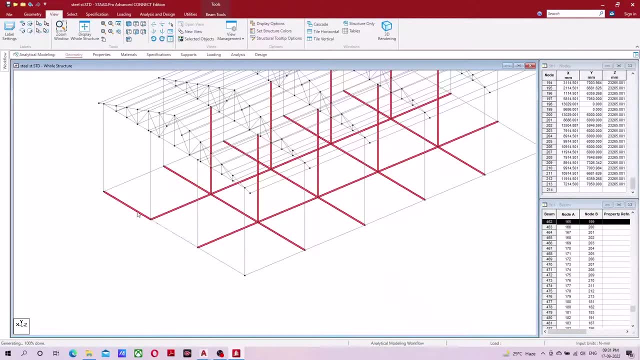 Press control, select the last one, like this. so what will happen? It will be unselected. let's rotate it a little. if there is a problem, then See this. we can rotate it with the navigation key. See, the middle one is only selected. I have to delete it, simply delete from the keyboard. 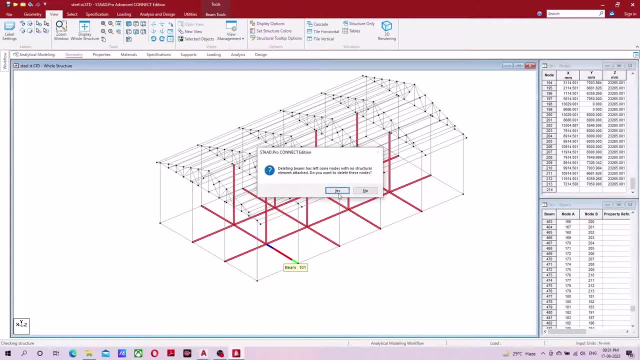 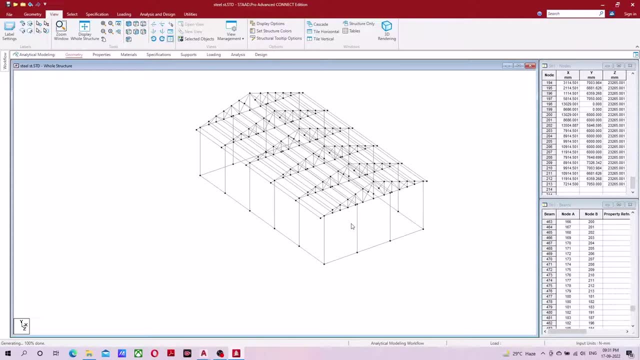 Yes, this part will be deleted here. See, this is deleted. look at This. much part is completely done. so my model is complete here. After completing the model, what will we do next on it? We will provide support. so, to provide support here. 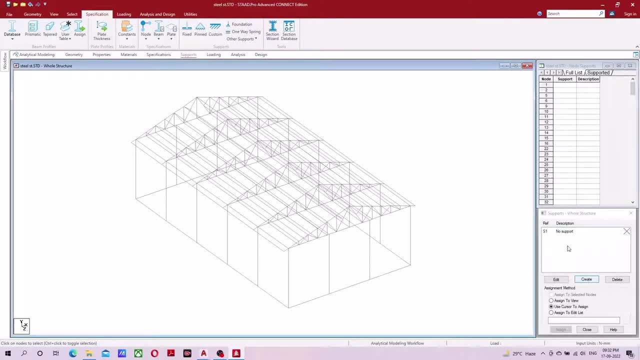 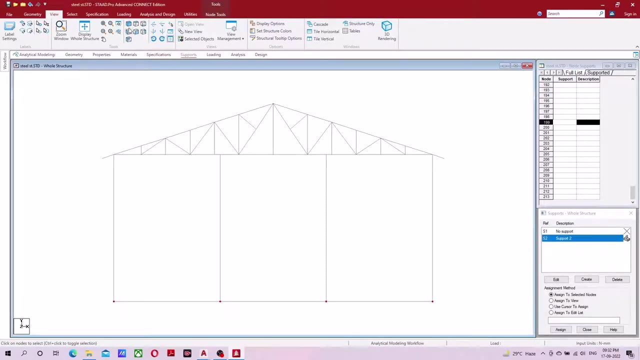 Go to support. after that here by default, Click on create, then add. After that, select fix. to go to view menu, click on front view And select all the nodes below. Look at the isometric view. this is properly your support part. Selection was done or not. after selection, simply here. 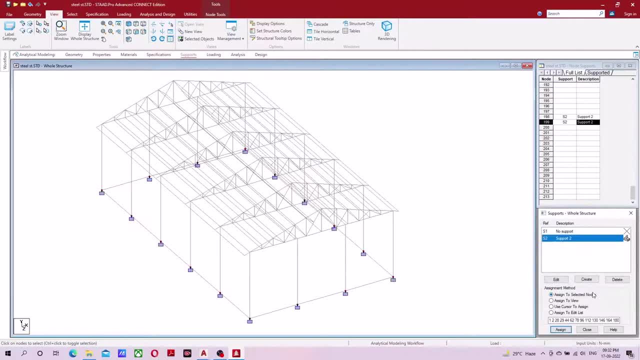 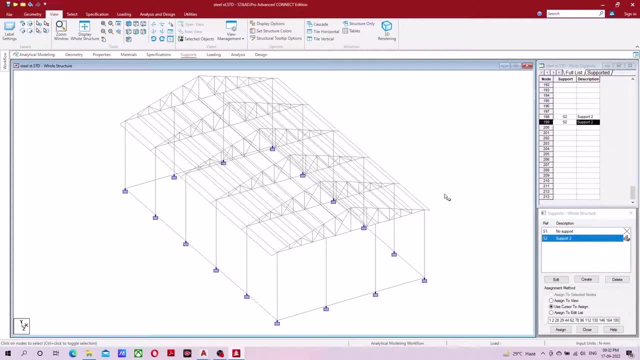 Assign. yes, so see, this is my support. Fix support has been assigned here. after that, What will we do on it? we will provide property. what will we provide property? According to my client requirement, all these columns will be RCC column and this beam will be RCC beam. 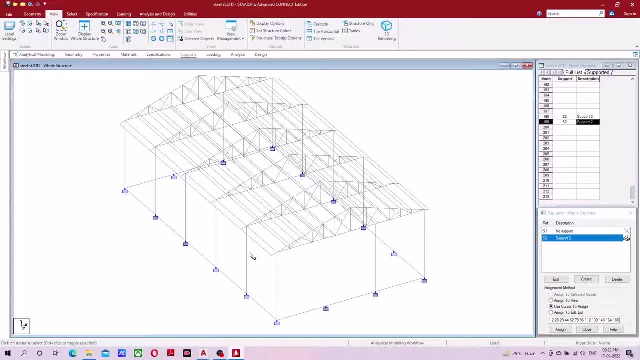 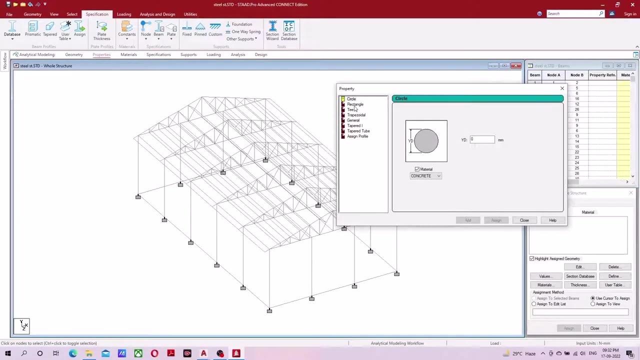 On it. this frame will be a total steel. so first I provide RCC property, I provide this material. For that I will have to go to the property page. after that, here I will select on define option. now what I will do. Here I will select on rectangular. here I will provide sizes. 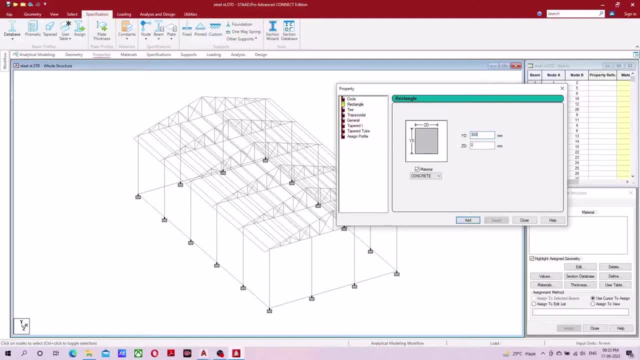 Column size. for now I assume 300 by 300. Later we will check. if this size is not ok then we will increase it later. But minimum: here we keep 300 by 300. After that: here the material will be concrete art. after that: 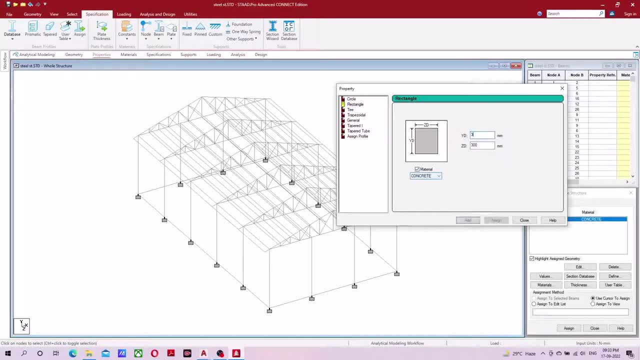 I take the size of the plinth beam: 350. Depth is 250 mm, the depth of 350. This depth will be of 350 and the width will be of 250. I take this for the plinth beam, I simply add it, then close. 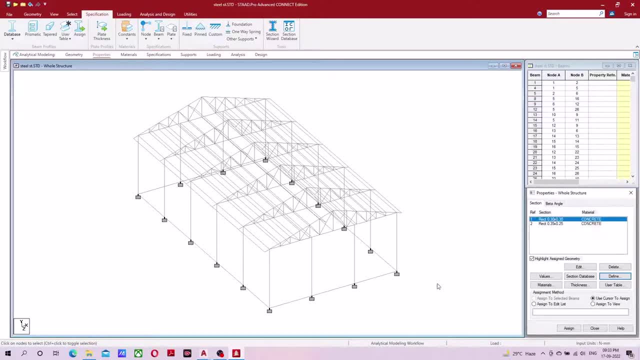 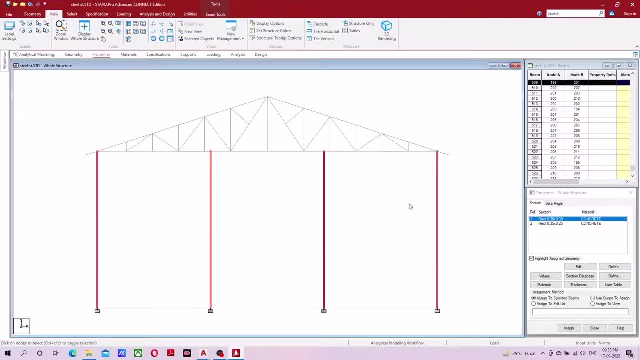 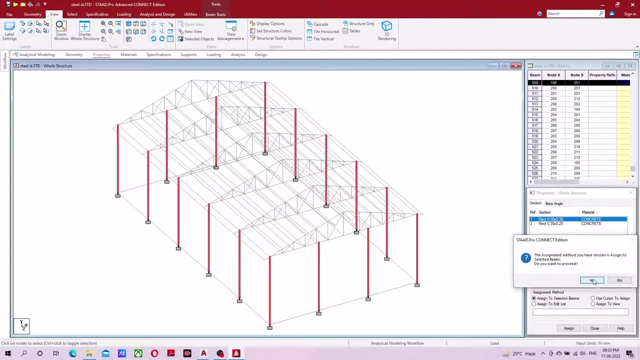 Now, after selecting the first one, I will apply all the columns above. Simply go to the front view after pressing control. Here you can drag and select a column like this. Check on the isometric, then here: assign Assign to selected beam. assign: yes, this column has been assigned. click on the mouse. 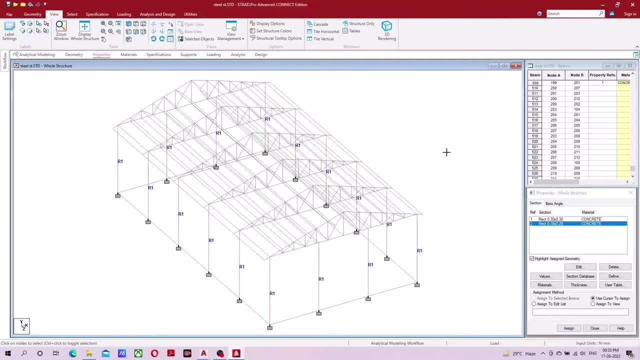 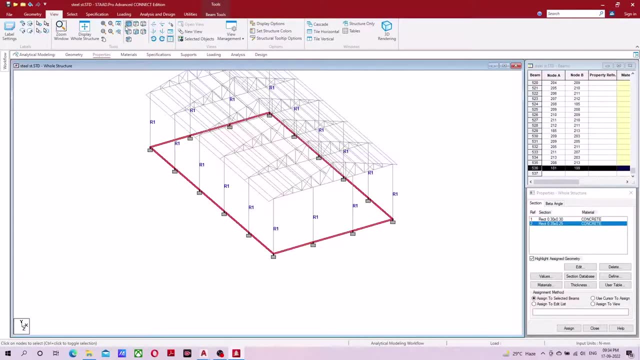 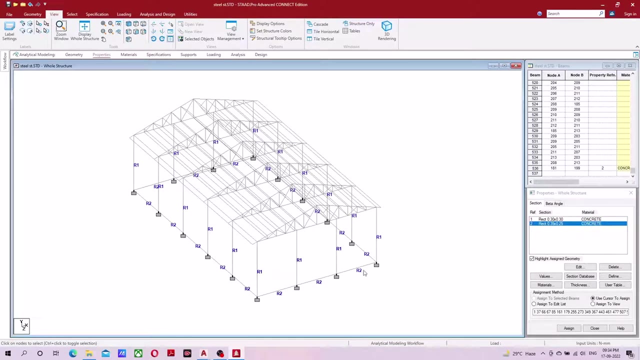 After that, select the beam option. sorry, select the beam option. Go to the front view and drag this lower beam Select. see this selection is done. then assign. Click on. yes, I check this, then click here one time. Click on select all, then right click here. 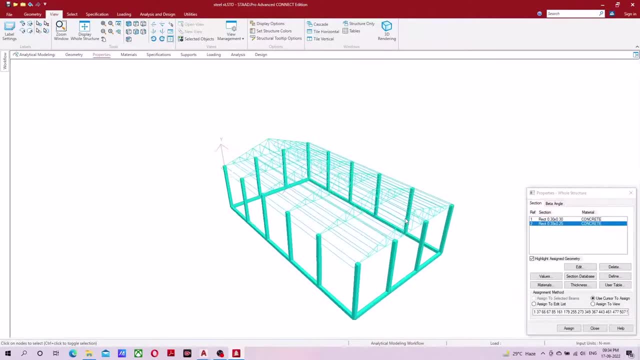 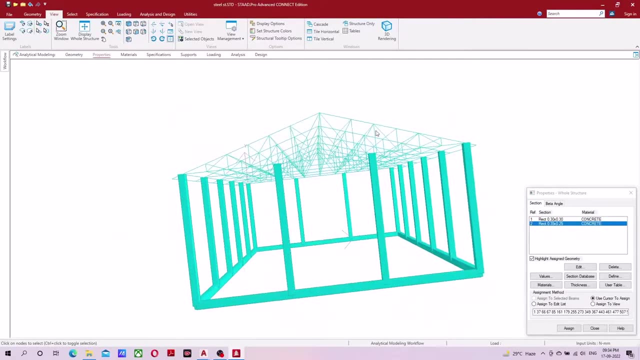 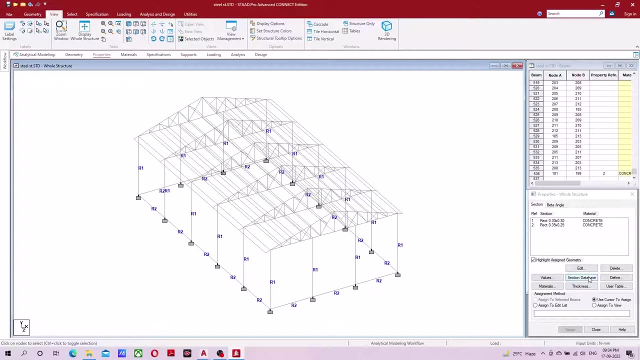 Click on the coloring, see here your column and here Your plinth beam has been completed. here now I am. The upper part is the part of steel I will apply here. So what will we do here for this steel You have to go to the section database. steel property is not available in your define. 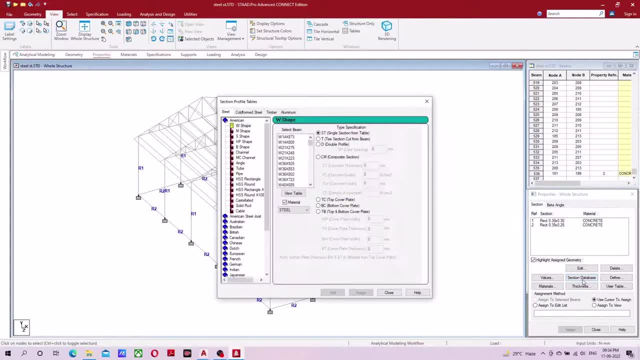 Click on the section database. after clicking, After 4 to 5 seconds, this window will open. On top of this, your variety country is available here for America And here Australia. different countries are available here, see here. There is also Indian. if I click on Indian, then here variety Indian property. 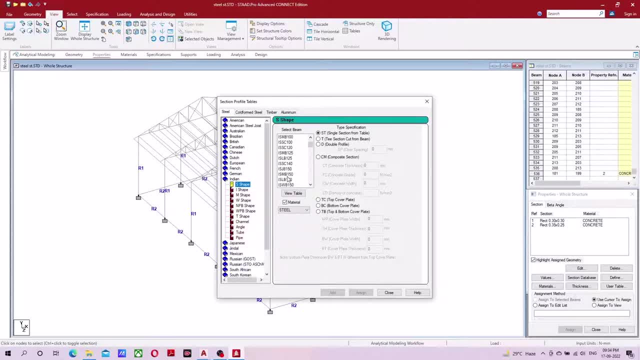 Available like this inside SF. see here ISM Will also be here. so here I have taken the column of RCC, so here I will not provide the column of steel. if you want, You can add it from here, whatever size you want. if you want a channel, then click on the channel. 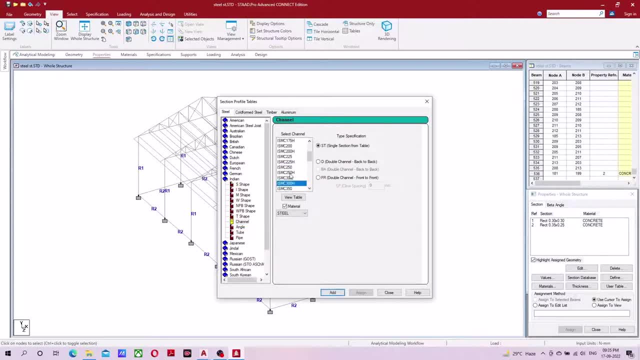 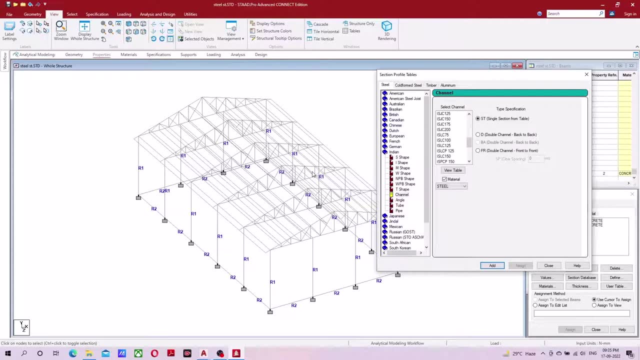 Click on it. here you can take different properties, but According to my client, whatever will happen here depends on your client: Which size to give, which shape to give. ok, If he wants a channel shape, then you can take a channel, but which channel? 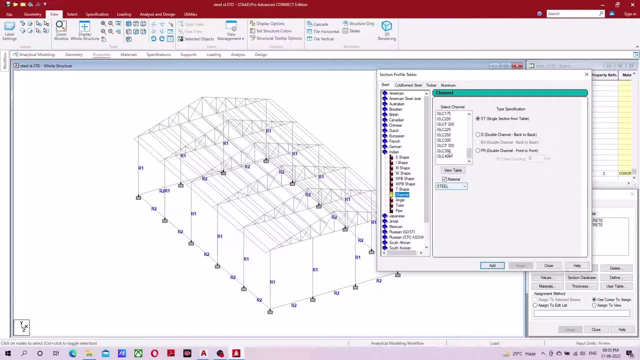 Which size will pass here. it depends on the design. So here you have to take the member of which shape. it depends on the client. If the client is telling you, then according to the availability of the market, Here you are, What type of member will you take? you will decide that. but basically the column. 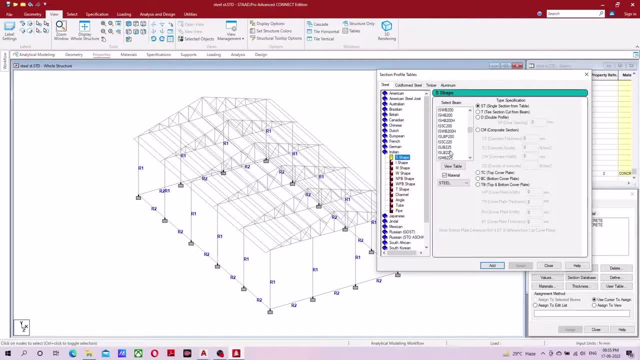 If there is a column of steel, then here I take ISMB. I take the difference size of ISMB, but here I do not have a column of steel, So I don't take the column. the rest of the upper part is according to my client. 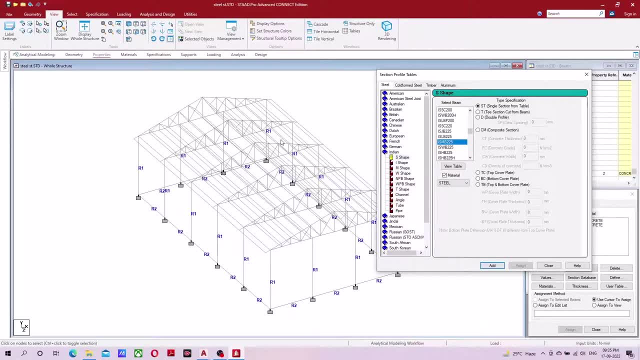 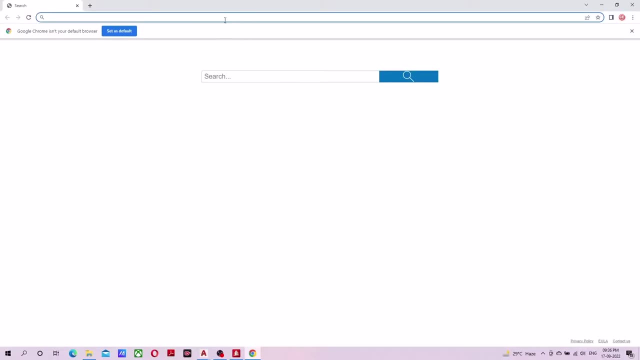 He wants tube section, which is like a square. He wants tube section. so I will take the tube section: tube section. How does it look if I show it to you? How is the section of the tube Here? I simply searched on the net. here I wrote: 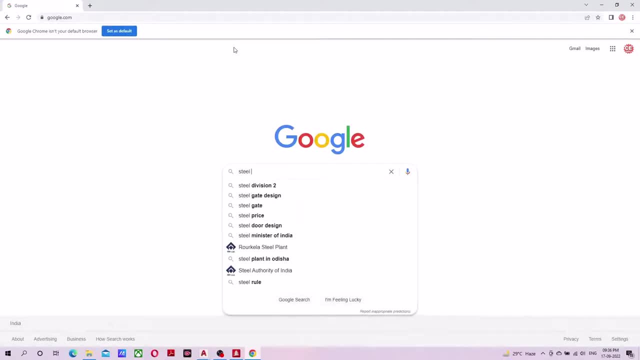 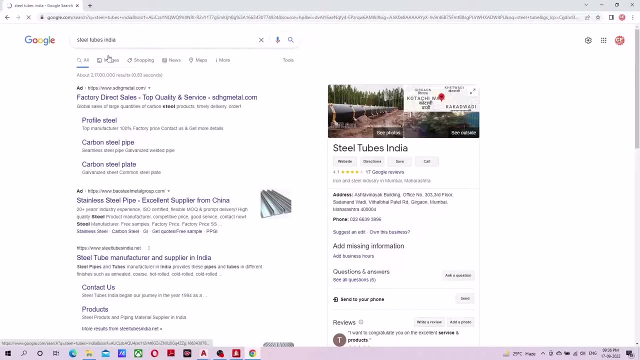 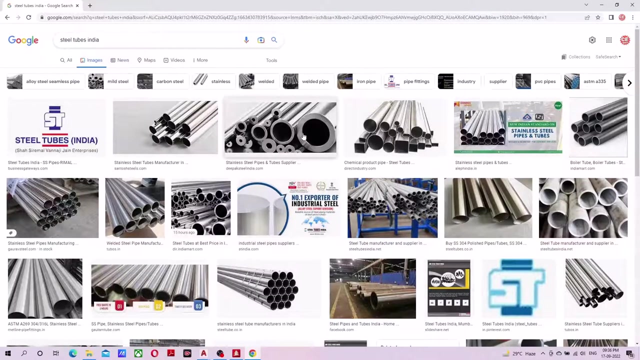 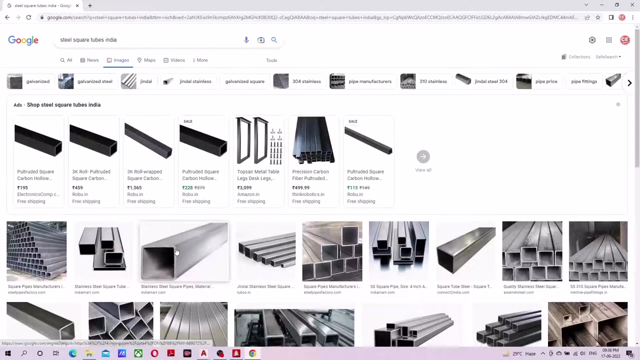 Tube, steel tube, Indian. Let's go to the image. This is a circular pipe. ok, circular. If you want a circular, then this is a circular tube. if I want a square, Here, it will be. Here I write: square Steel, square tube. See this. there is such a section. 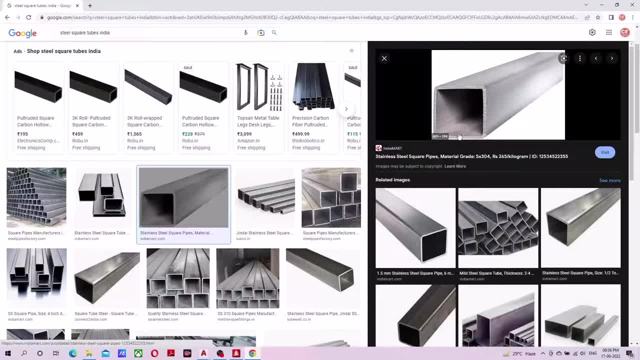 This is the section of the steel tube. If you want rectangular, then this is a rectangular section. If you want a square, then this is a square. If it is rectangular, then it can also be a rectangular section. And if there is a pipe section, then you can take a pipe section here. 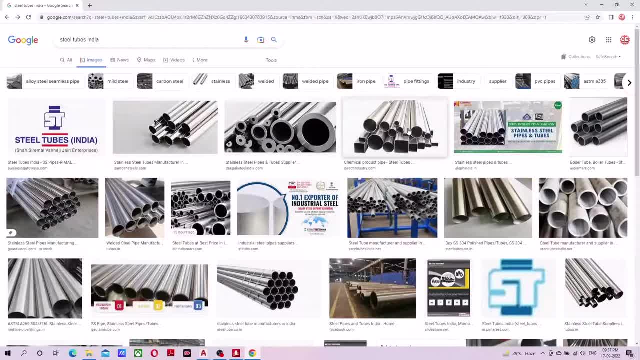 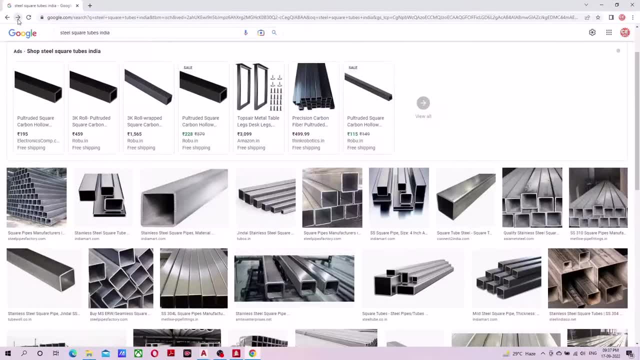 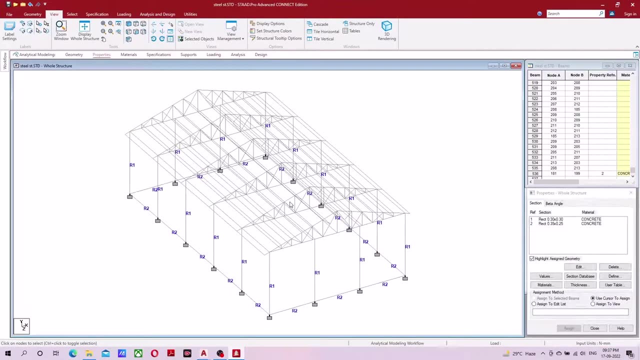 This is the pipe of the steel tube. It has some thickness And it has some direction. This is a diameter. So whatever section I take here, I will take the shape of rectangular and square. So I have to provide this section. So how will I provide that here? So here I have different members. 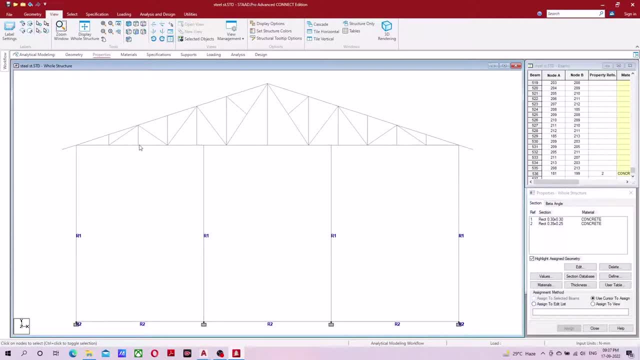 If I go to the front view. So this is the lower member. This is the lower member I have already told you This is the tie beam and this one is the raptor Which carries more load. So I will provide a little bigger section to both these sections. 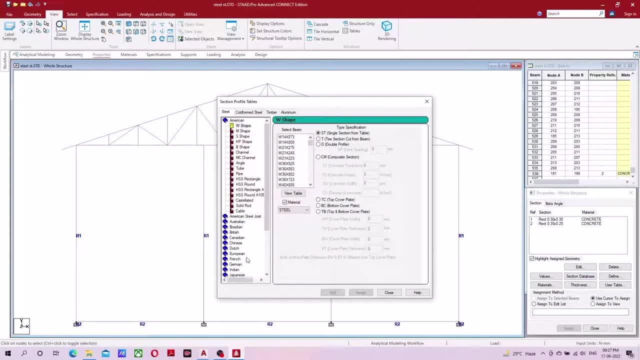 So here I go to the section database. Here I come to Indian. This will not be available in Indian. You come here On the tata structure. This is available in the tata structure, So tata also imports you to India. So no problem, After coming to tata. 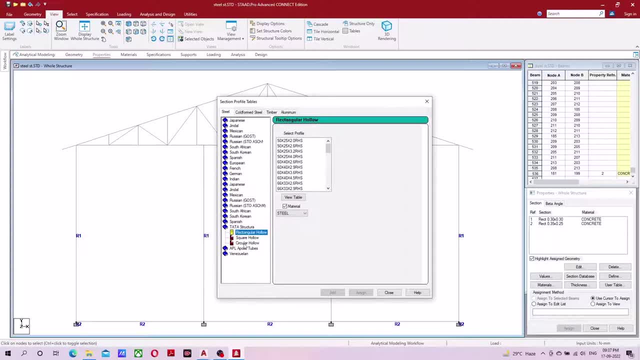 Which square, or rectangular or circular do you want? So you can choose from there. So suppose I want a square. So for this lower member and the inclined member I will take the square section And suppose I take here Which size will pass here? I will take it accurately after the tile. 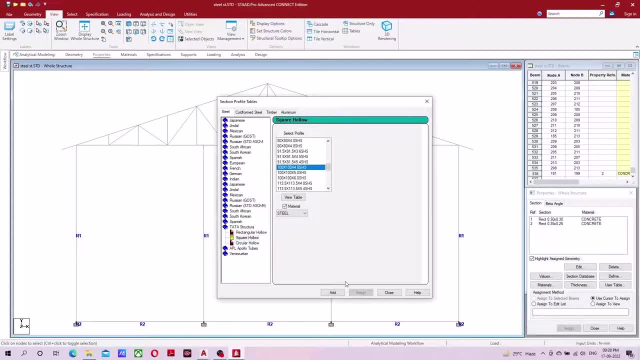 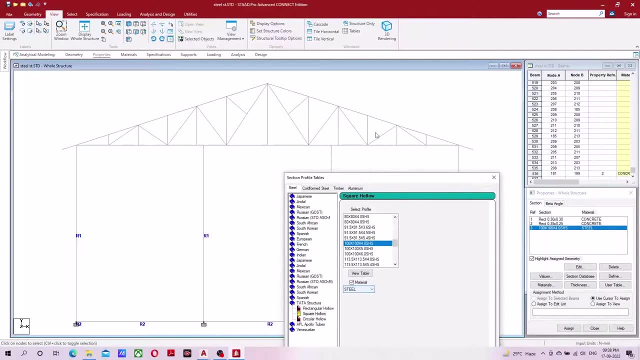 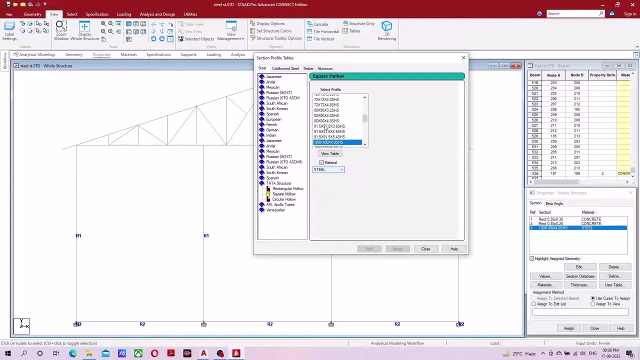 For now, I assume and provide 104 here. This will be of steel, Directly added After that. This is the secondary member in the middle. All these secondary members, For all these secondary members, I take a little small size. I take a little small size of that square. 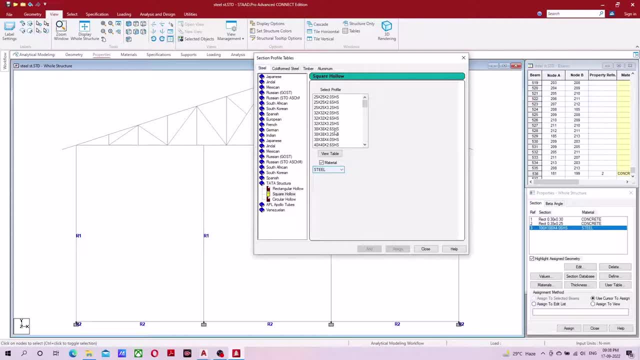 Because this is a secondary member, It will pass in a small size. I take this, for example. I take the member of 38-38-2.6, Steel will be added. This is a small section. After that, next will be your perlin member. I said in the perlin member. 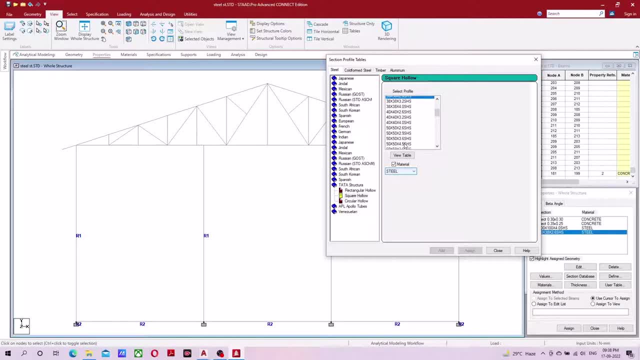 And after adding this I will show it again For perlin suppose I take. I take 60-64 of same square And 3.2, 60-60-3.2. And one more thing: Which size will be available It has to be seen in the market. 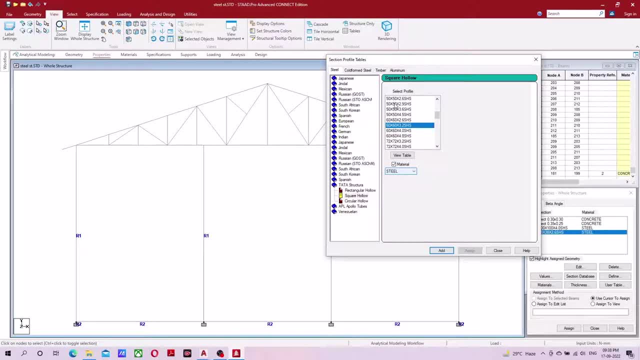 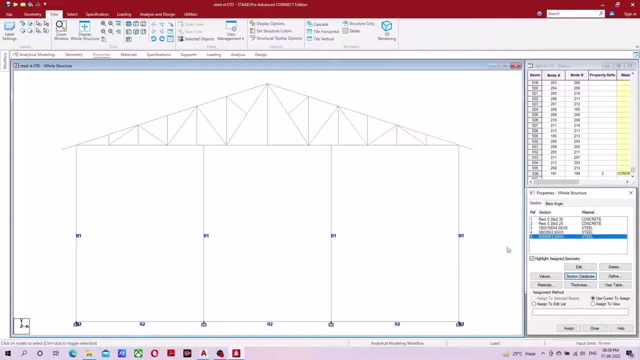 Because it is different from 60-60, It is 72. So it will also have to be seen in the market Which availability is there in the market. After that I added it here, I closed it. So first we will provide Which one we will provide. 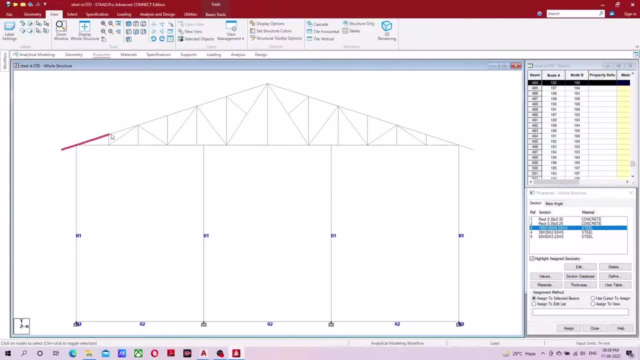 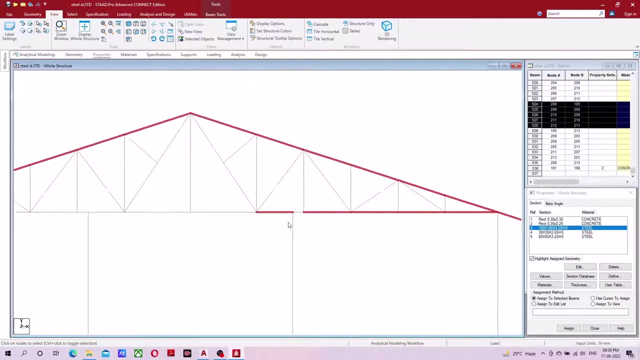 To provide this. Press the control And select it one by one. Select in the middle. There should be no selection in any joint point. So press the control. I selected it one by one, After that this middle one. So there should be no selection on any joint. If there is any problem, then zoom a little. 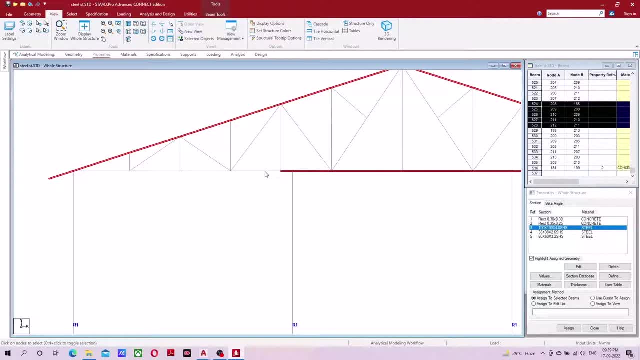 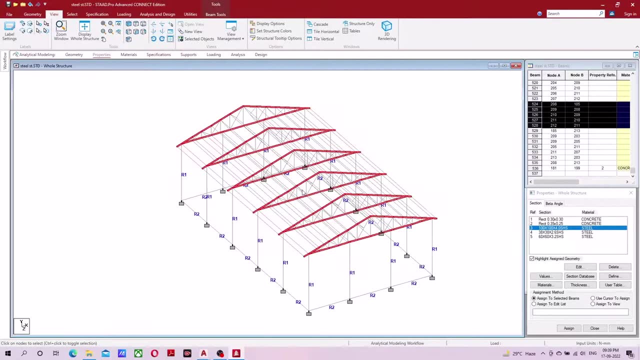 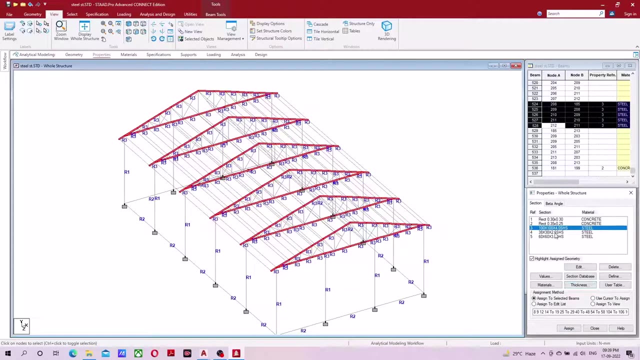 Click in the center. After that you do it like this: After selecting. After selecting, Select, ensure isometric view. After that, see if it is properly selected. After that, Assign to selected beam. After that I will provide the second. On the secondary member, Go to front view. Press the control. 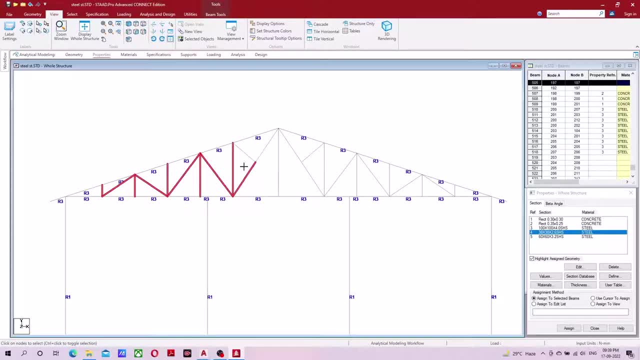 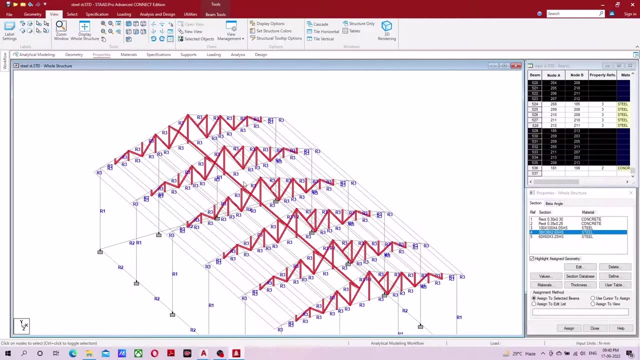 Now I take it Like this: I can drag it Here. I select it like this. I select it like this: Carefully select it And after selecting You will see it on isometric That it is not properly selected. There is a mistake here. Press the control. Press the control and select it. 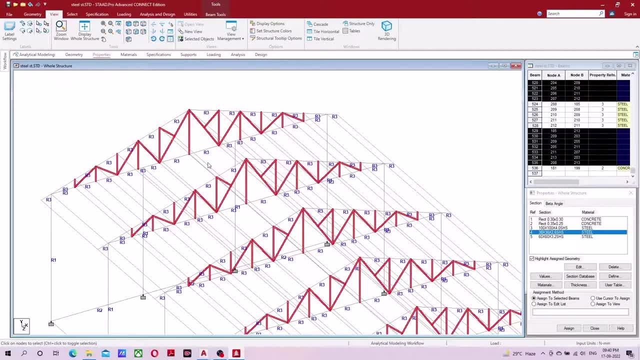 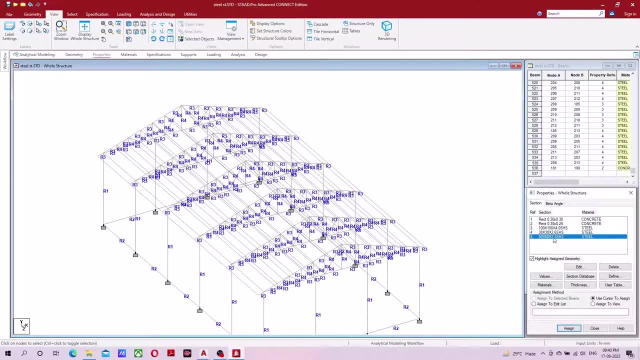 That's why, Whatever you will select, You check it on isometric view. After that assign it. After that, this member- I am going to provide it in perlin. What is perlin? This is the member. This member is called perlin, So it will be automatically assigned. 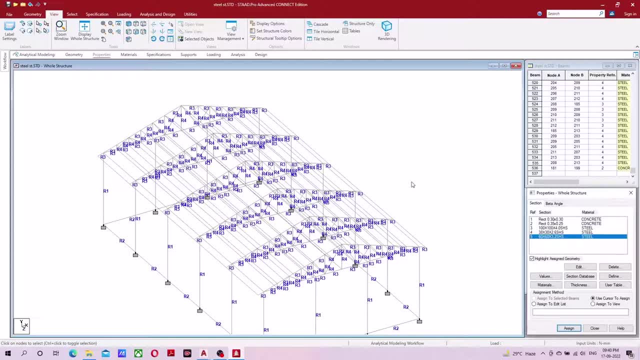 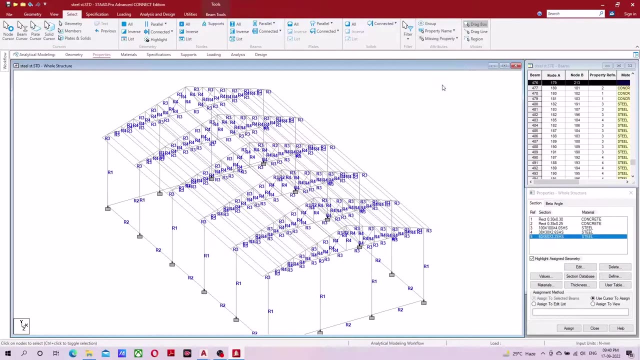 Because all the properties have been done except perlin. So how is the automatic selection Select it After going to the select menu bar. Click on the missing property. After that, again missing property. Where there is no property, It will automatically highlight for property And once here, property, Missing property. 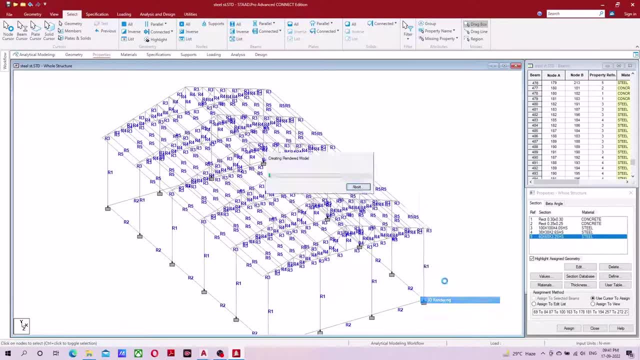 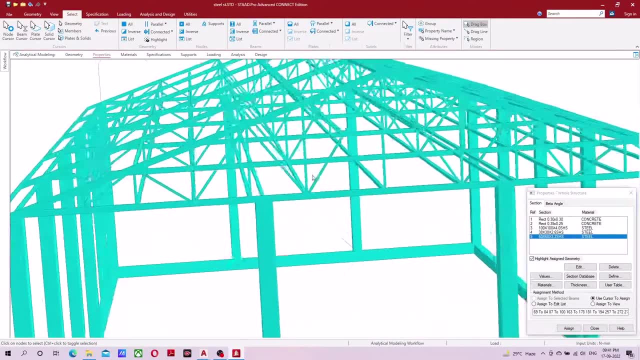 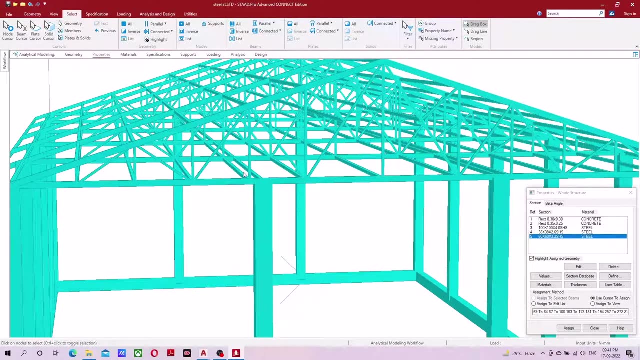 After that assign here. So see, this is your property Here. you will see. If you will see, Then there is a connection above And there is also a connection below. This is the connection below. This is called tie beam And this is called tie member. Tie member is a little more. 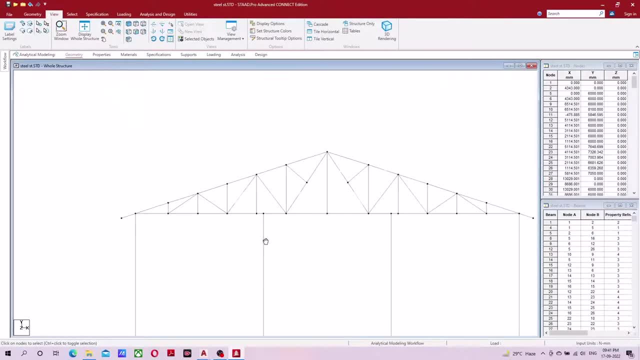 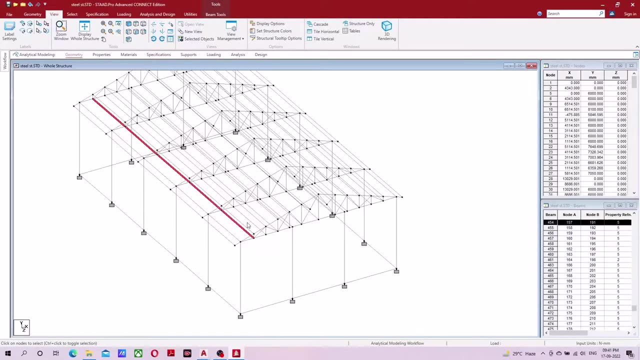 I will reduce it Here. I simply went to front view After going. if I press control, If I drag it to the joint point With the beam cursor In the isometric view, this will be the member selection. I have to delete some members. This is the selection. 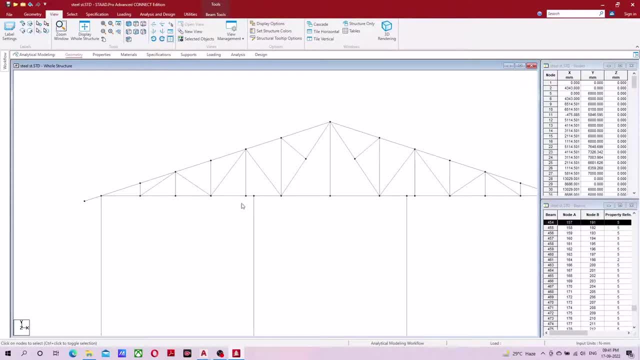 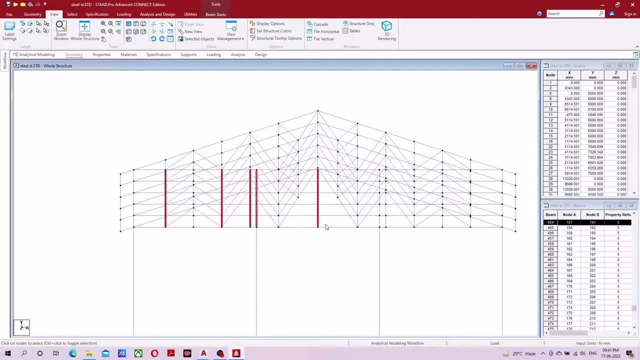 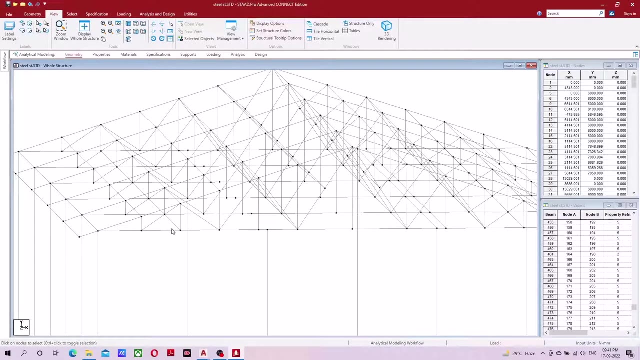 I will delete the first one and the second one, this one and this one. and here now see, here is the selection. I have to delete this. I have to keep one by one. I have to keep one here and delete this. I have to keep this too. 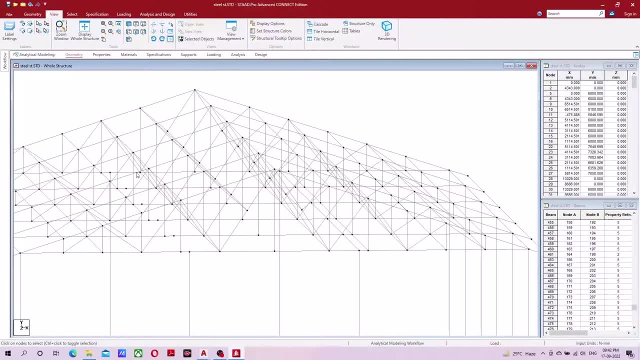 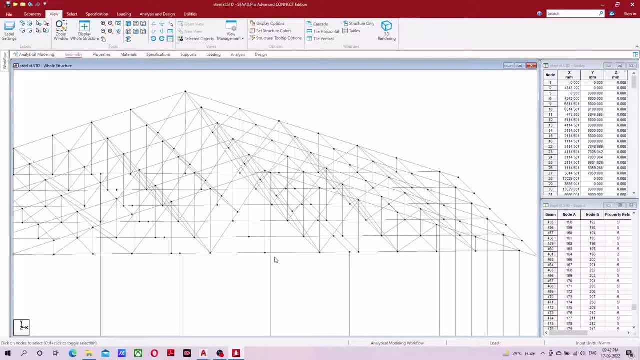 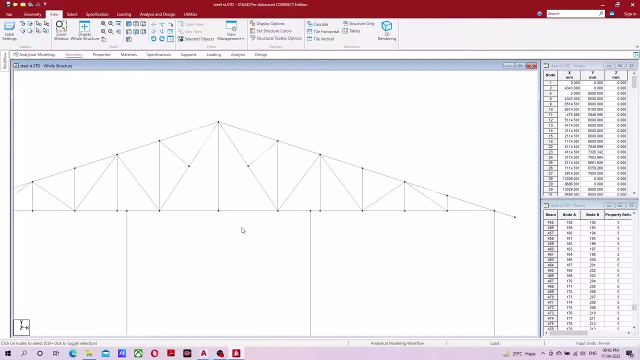 keep some less. This is the purlin part. we are providing the lower part. if you want to put some lighting here, then you can adjust the lighting. here. you can give lighting. that's why I provided it there. By the way, I will delete it in this type too. so the front view is done. after going to the front view. I have to delete this one. I have to keep this one. I have to delete this one. I have to keep this one. I have to delete this one. 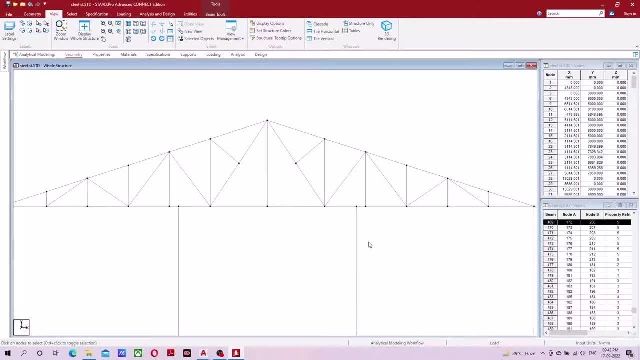 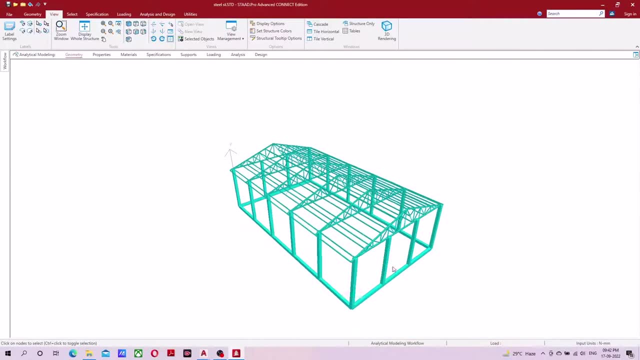 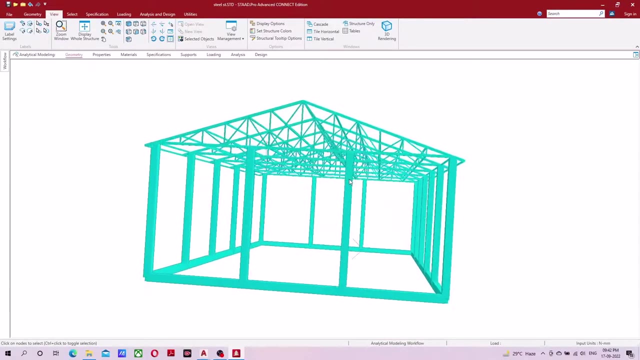 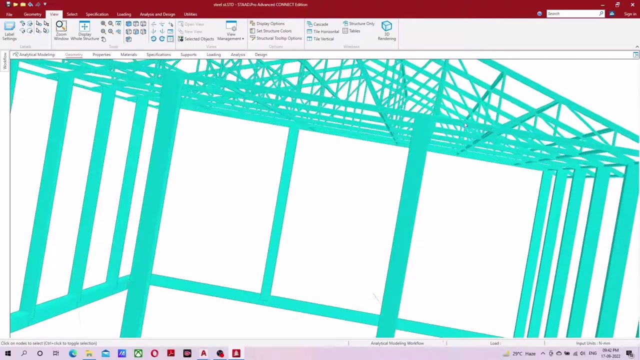 I have selected the right one. ok, delete. yes, right click rendering. let me check a little that, whether it has been properly done or not. see this: if you see the lower member, then there is no member in every point except one. like: if you see, then this is the first one, there is no second. there is no join in the second. there is a third. there is no join here. there is no join here. see, like this: here I have provided one by leaving one, 1 here. 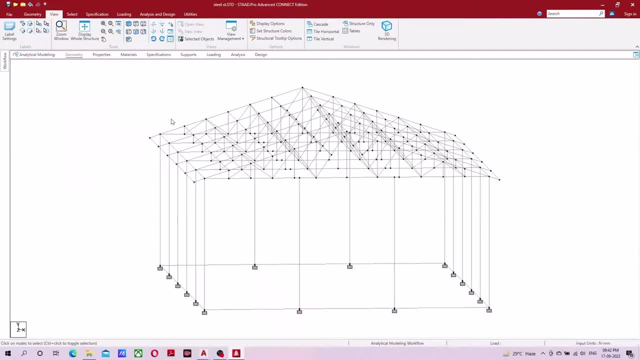 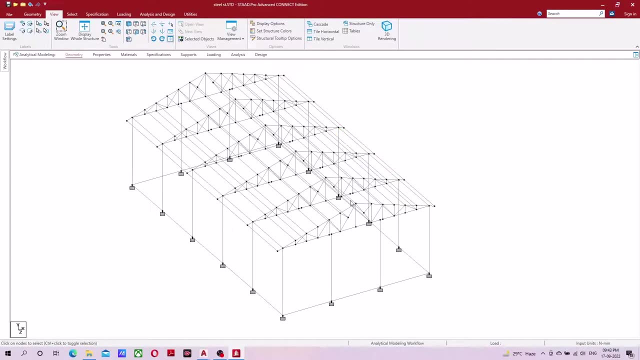 ok, you can do something like this here. see, this is done after this. see, this whole member and property is fully completed here. there will be a seat on it, so I will not provide the seat, I will provide the load of it. 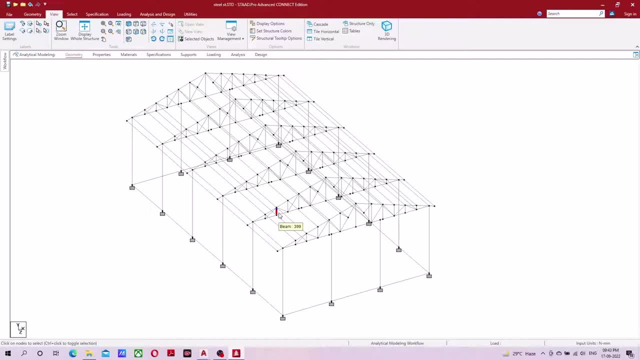 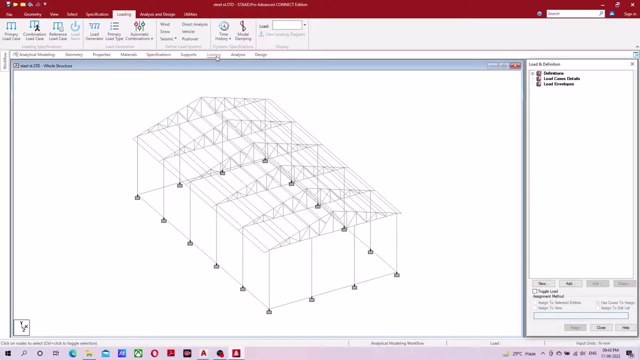 after this is completed, here you will provide loading on it. to provide loading here, go to loading. after going to loading: after going to loading here, you click the plus symbol of this definition. after that, first we will provide the seismic load. then 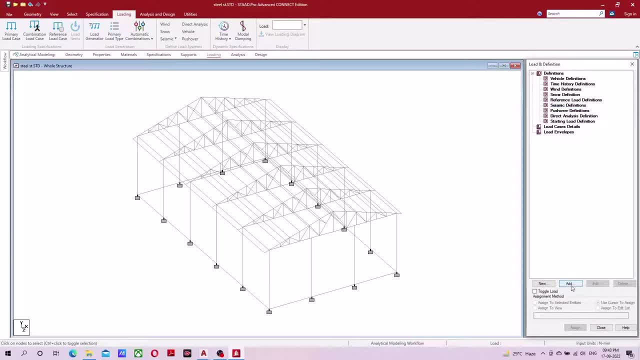 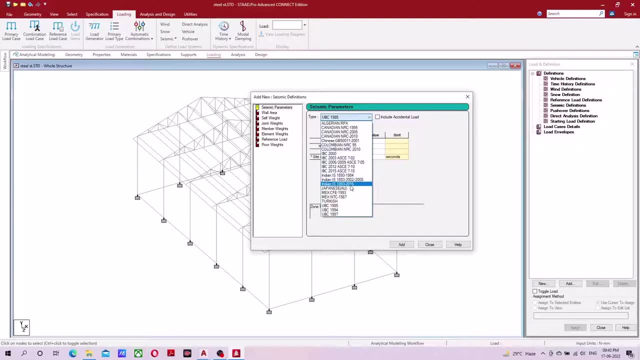 go to seismic definition. after that, simply add it. after that, the type where you will type according to the is code of India, which is IS 1993- 2016. click on it after that. after generating here, here you can choose either city or you can click the zonecomes. 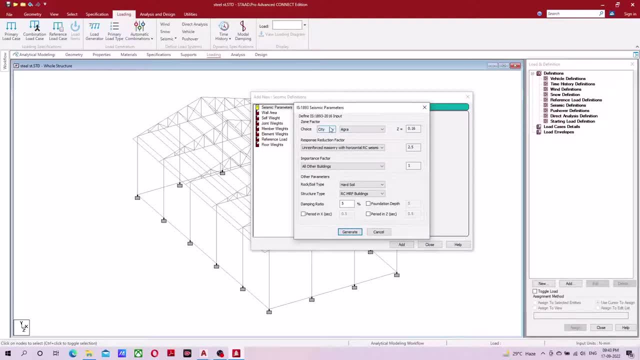 you are place in which Zone. so here you very simply click over the zone. where is basically? in our country there is four zone: 2, 3, 4 & 5. but here you can heaven the befitting me. four shows, two news, four topped only house. room, not the flows welding. then click here for further control. here you will get close under it. you can see the seashore were the contacts and place of the facility. Кор, please take care. if you can join once again for complete $ collection, here you will get back. 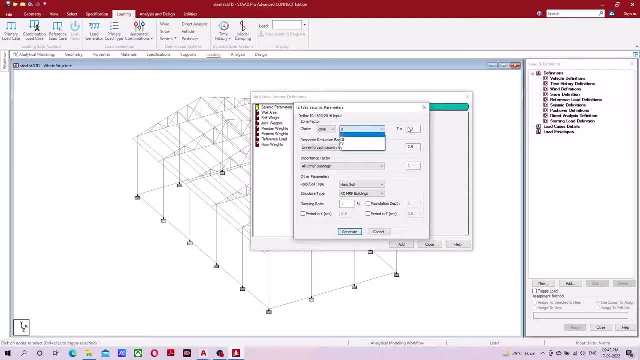 all the part again, and they are some additions. we like to add one and after this one is, and accordingly the value will be changed: 2 will be 0.1, 3 will be 0.16, 4 will be 0.24. 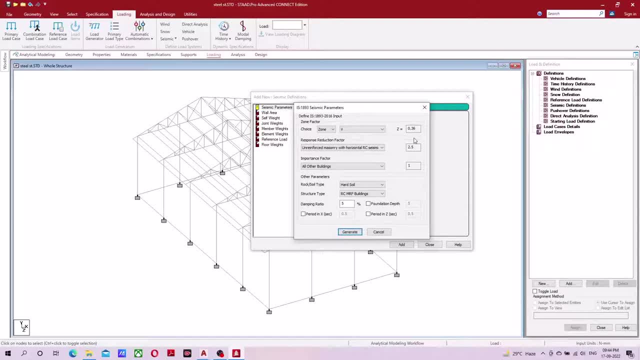 and 5 will be 0.36. if you want complete video on the sesmic load on manual calculation, currently for start pro there is no manual calculation, but if you want deep knowledge on it, manual calculation, then comment for that. I will make a separate video. 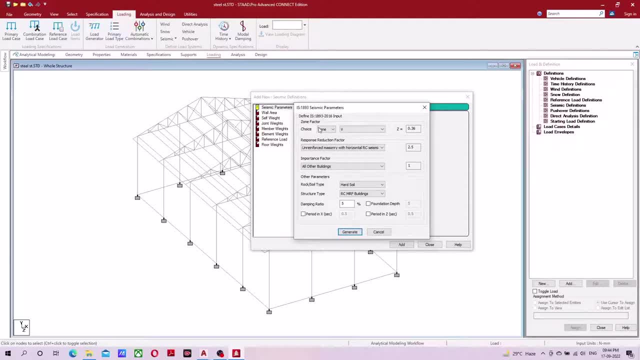 in which I will explain sesmic load completely. so basically, if you know the city, then you can take city. after that, take your city, whatever city you have. if your respected city is not available, then you can take nearest city. so my native place is Bhubaneswar. 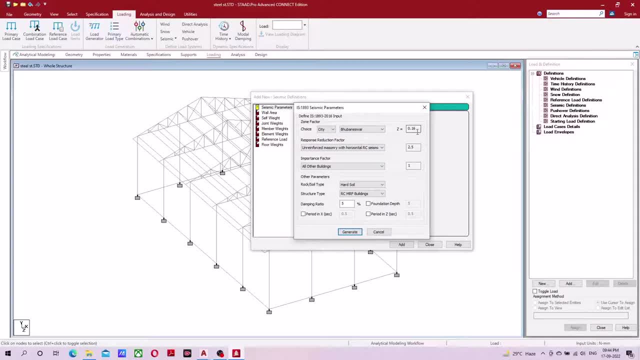 so I take the city, Bhubaneswar, whose zone is 0.16, which is number 3, so I choose it here. after that I will go here. here is variety option. first is steel building with ordinary RC moment and special RC moment. so basically this frame is: 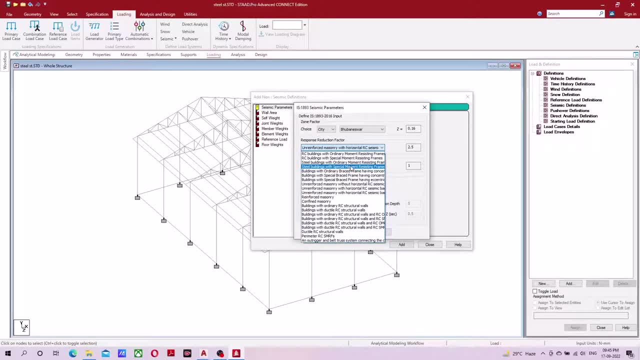 ordinary RC moment of steel. special RC moment is big garment building, 3 floor steel building. you can take special PV type structure. but this is small. go down. so take ordinary RC moment whose number will be 3. factor of safety should be 3, important factor will be: 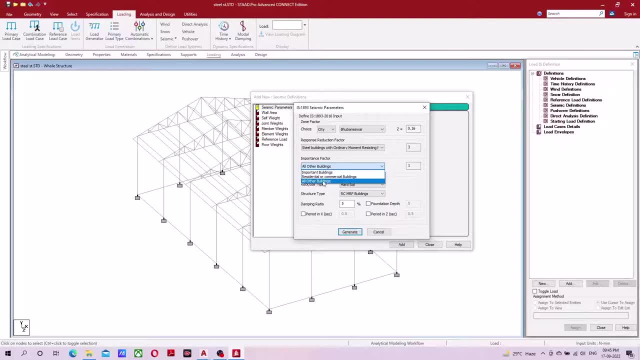 important building, residential and commercial building, all other building. so here I take it on commercial building, because this building is of commercial type. here we will keep some material of go down for commercial purpose. so here I take commercial building. after that: here you will choose soil type. 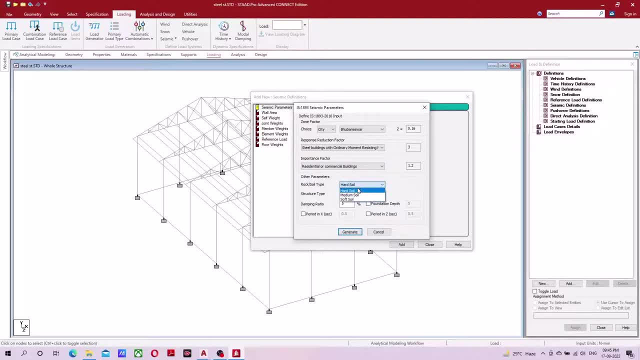 which type is available? this soil data. after testing of soil it comes out which type of soil you have. if you have hard soil, then you can take hard soil, and if you are not testing, then you can visit. after that discuss with client that which type of soil. 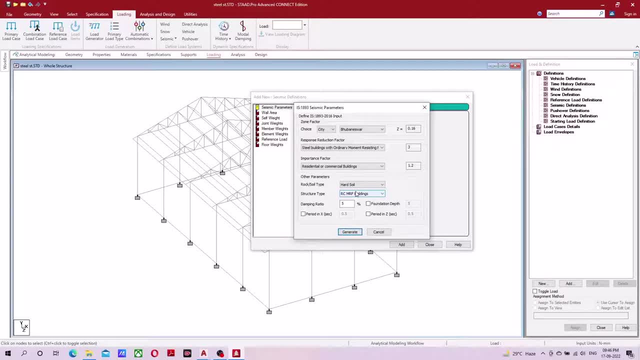 you have. if you have sand clay or black cotton soil, then you can choose soil category. after that building type will be steel frame building, MRF building. then click on building. after that damping ratio will be 5 pxpz value can be calculated, but here we will skip. 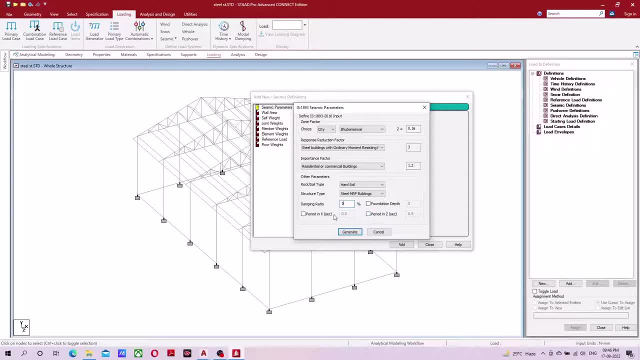 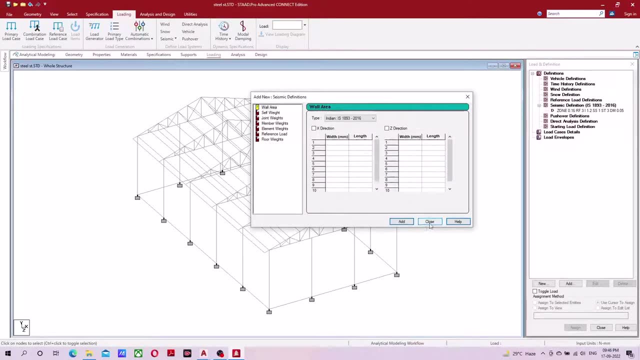 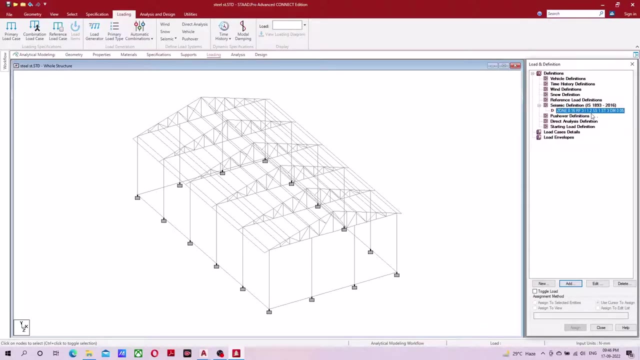 this is not that much important now, but this is provided, but for now we will not provide. after that, simply provide: generate, after that add, after that close. so here I have completed this part. one more thing: I forgot that I had to change my unit in meter kilo newton. 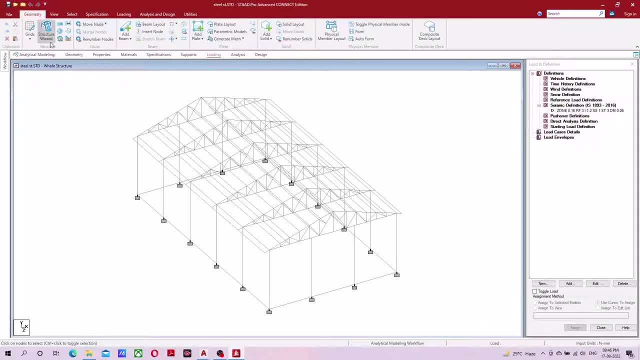 so now I will do: whatever load you will apply, you keep the unit after coming on matrix. keep the unit in meter kilo newton. before applying load, keep the unit in meter kilo newton- model in millimeter. but before providing load, choose unit in meter kilo newton. 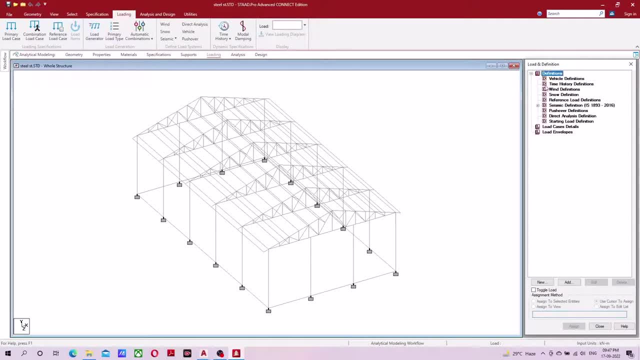 after this I will come on loading page and I will provide its direction. so basically, I will provide seismic load in x and z direction. so what is the detail of load? after coming here, simply click on add option here. the loading type will be: keep it in seismic. 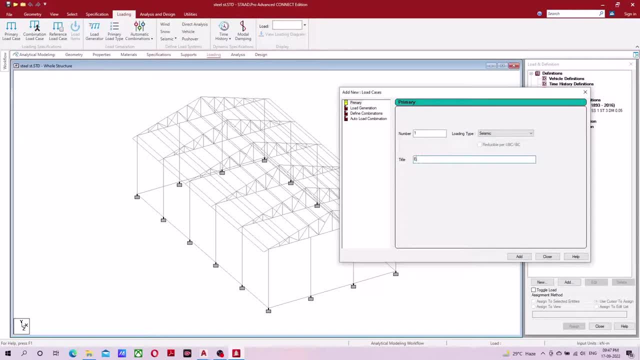 and seismic will be in two direction. like I write here: eqx- eqx means earthquake in x direction. add again. write here: eqz- earthquake in z direction. simply add and close. I will write: do of seismic load and click on add. after adding, click on side, click on seismic load. 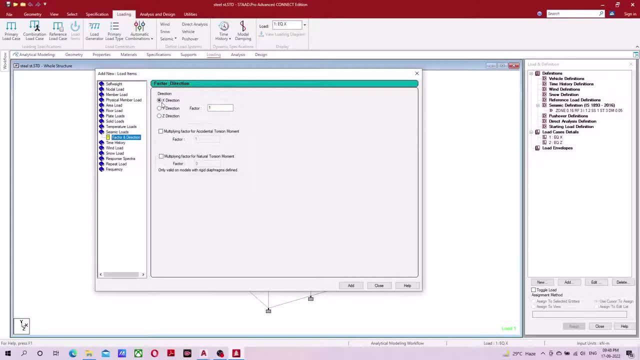 click on seismic load direction will be x and factor will be always 1. no need to change. first one is here. click on second one. now you will select. seismic load direction will be z, factor will be 1. add close. now you will see nothing is visible. 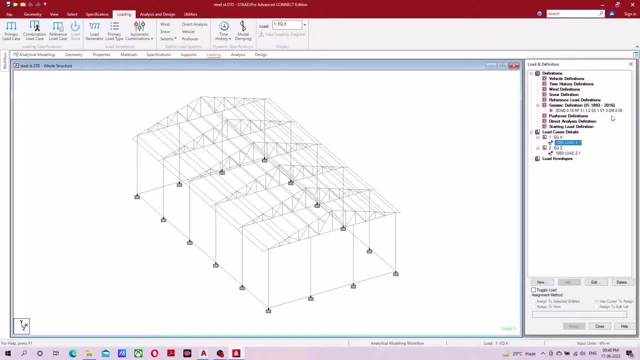 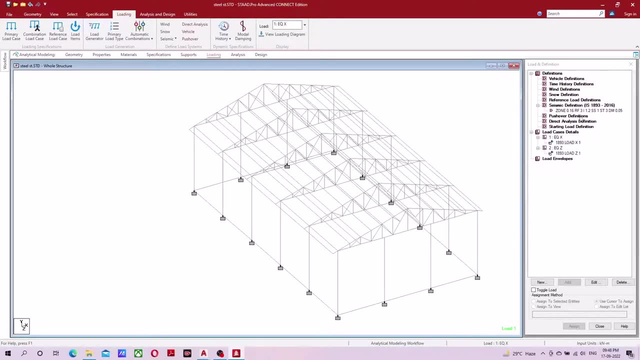 because seismic load process is not complete. we have to provide all load after that you will see. now you will not see. so I have provided seismic load. now I will provide wind load. to provide wind load, go to wind definition. simply add after adding. again add and close. 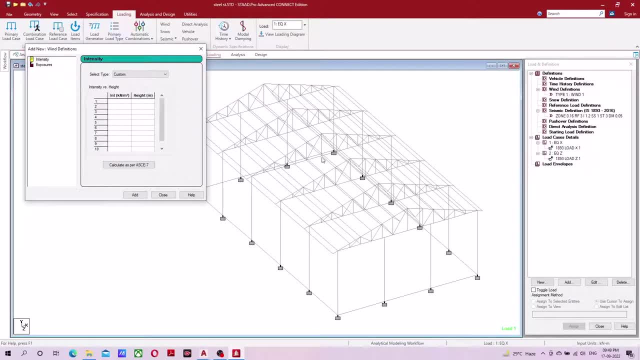 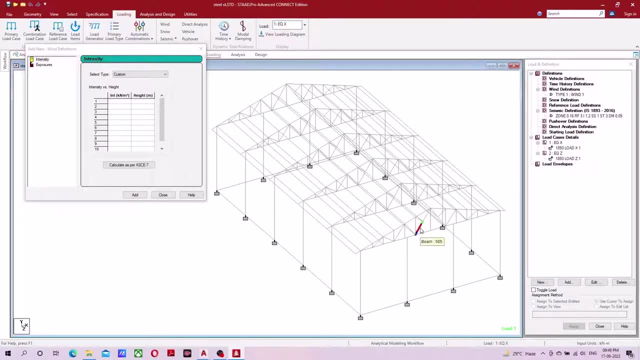 after that, click on wind type 1. after adding wind type 2. now you will see here, you will not see. now you will see here. you will not be able to see. now I have added. I am adding. now I am adding. I am adding now. now I am adding. 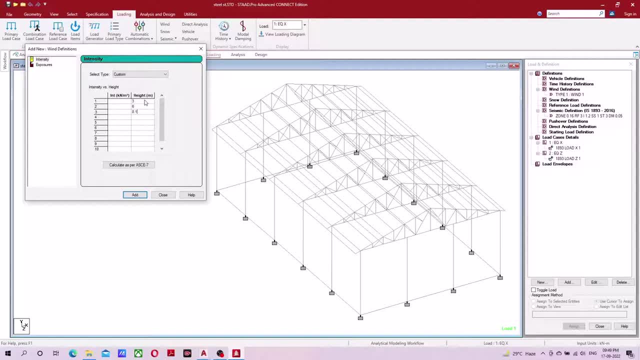 now I am adding now. now I will make a video in which I will upload the complete calculation of the wind load so you can check it out there. for now I take it by assuming, so you can take the assumed value for now, but the original value will be considered according to the calculation and I will upload the calculation soon. so here I take it by assuming 1.1 intensity, 1.2 intensity and 1.3 intensity. I have provided the intensity by assuming here. 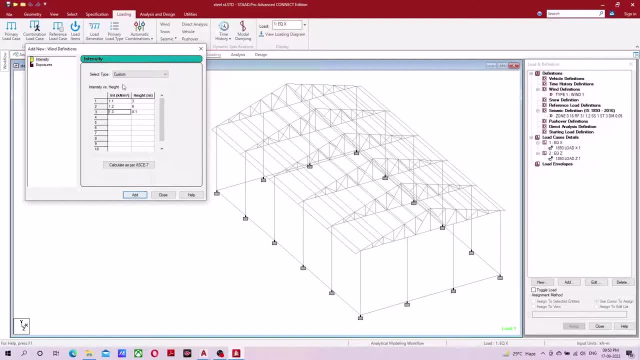 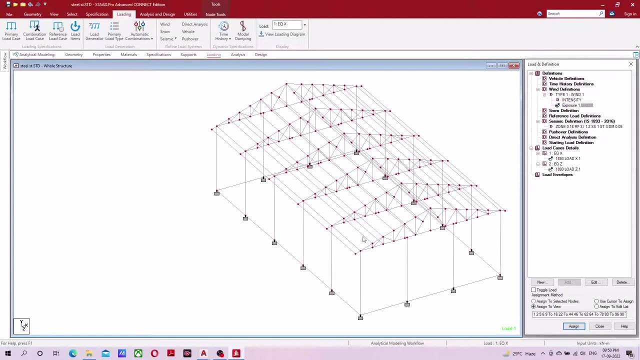 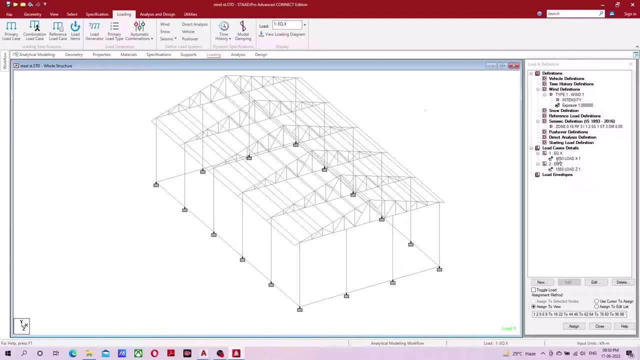 after that, here I will simply not make any change- I will add this factor. I will add this factor by doing 1, then I will close it. after that. see, here there is a question mark. click on it. simply click on assign to view. assign it. click yes. so this seismic load will be applied to all the joint points. after that we will provide the same direction here. we will provide its four directions: x plus, x minus, z plus, z minus. we will provide in four directions. 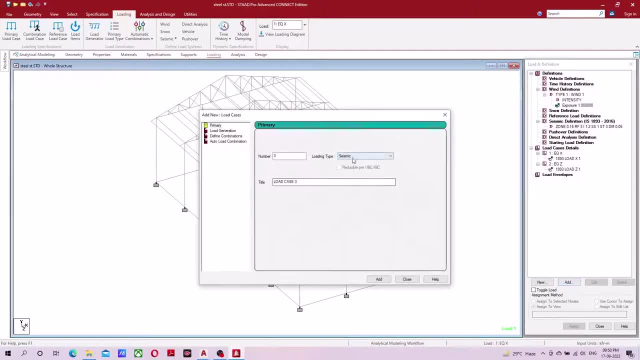 so here the load case is in the middle. after adding here, the loading type will be: we will keep the winter here. we will keep the wind x plus. similarly, similarly, after adding here, your wind will come x minus, after that your wind will come z plus, after that your wind will come z minus. 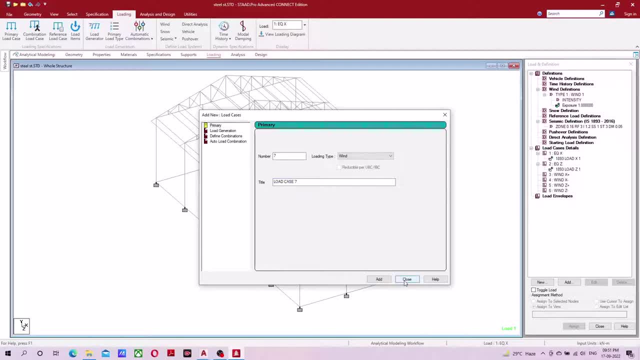 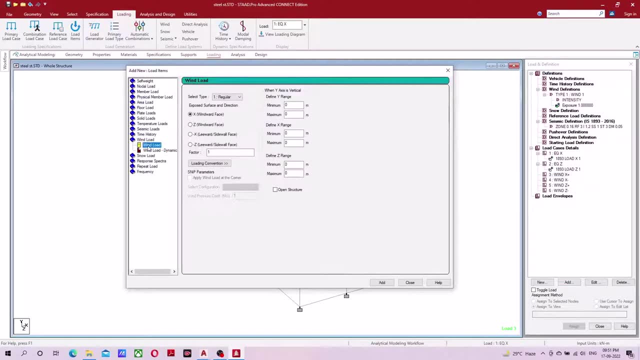 after adding the second kraup here, I will simply add and then I will close it. after that I will click on the first option and add it. after adding here, you click on the winter page. You will find a window and a window is coming. 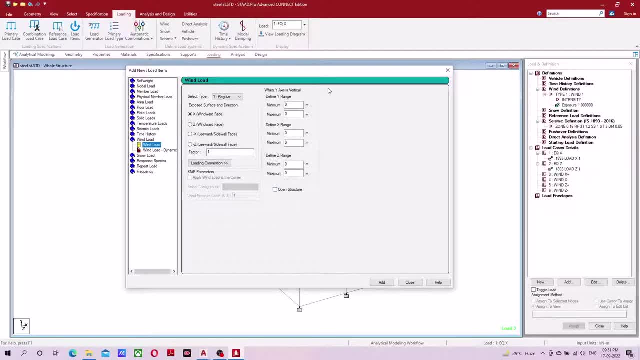 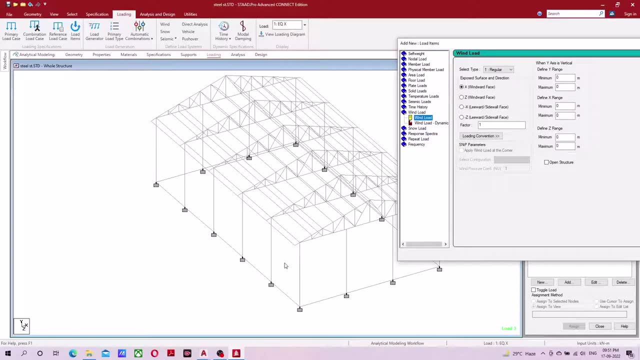 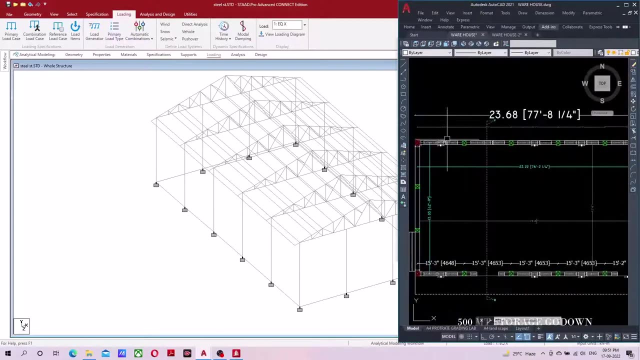 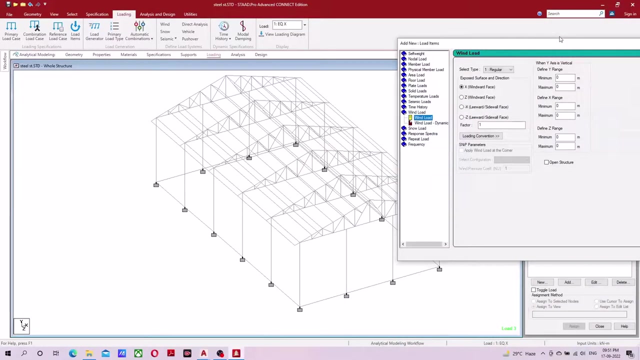 up below, etc. If your frame is complete, then click on open structure. But my structure here is a brick wall. on the outer side This is completely covered by a brick wall. Here is a door provided. That's why I don't keep it in the open structure. 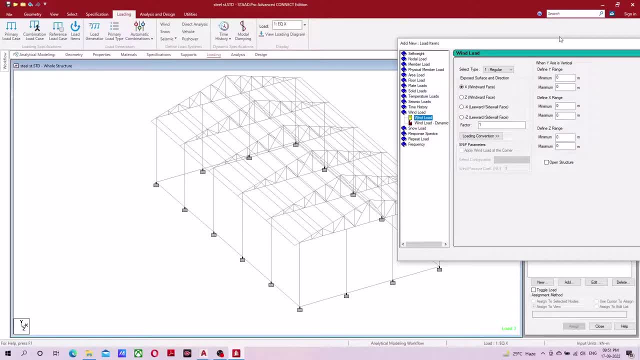 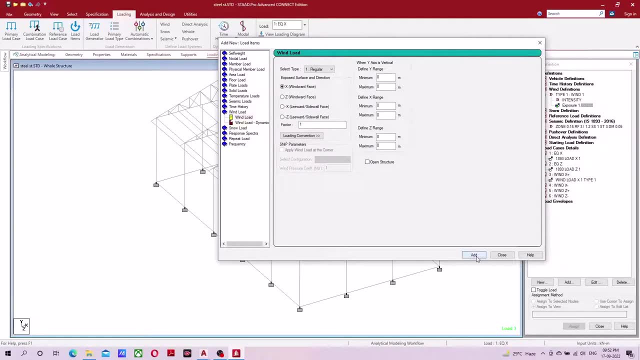 I will keep it in the closed structure. So if you don't have a brick wall, keep it open. I didn't keep it open here. I added it directly here. This is the first one added. After that I will select the second one. After that I will click on the wind load. 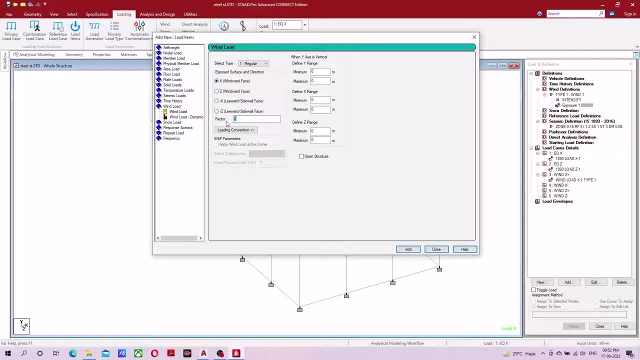 After that I took x again And I will take the factor as minus 1, Because I am taking x minus here. Don't take x minus here. The usage of x minus and z minus is different, So it is not necessary here. Do x and do the factor as minus 1. 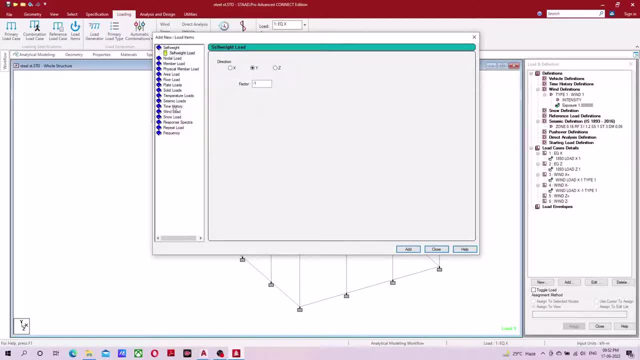 Simply add Wind z plus. click on the wind load. Take it in the z direction. Factor will be 1,. add Wind z minus. click on the wind load Here on the z direction. After that the factor will be minus 1 Here. do minus 1 After that. add and then close. 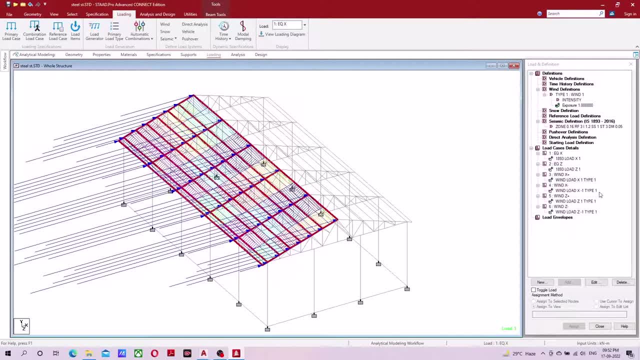 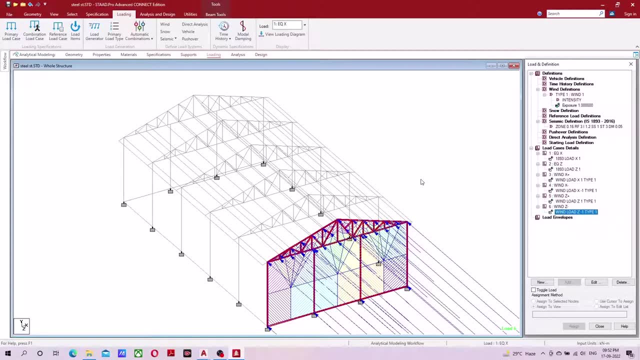 Now, if you select it, It will be applied in the individual direction: X plus, x minus, z plus and z minus. Here my wind load has been applied in four directions. After that we will apply dead load on it. To apply dead load Here, I will click on the load case detail. 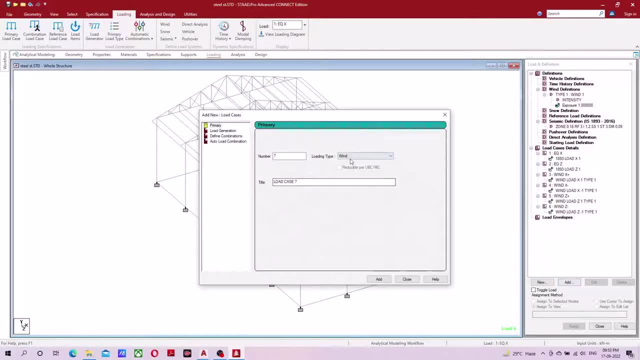 After that I will simply add here. After that, here the loading type will be: I will take this dead. So here you click on dead. After clicking on dead, Here in the title write dead load. After that simply add it. After that, close Here. I will not apply any live load. 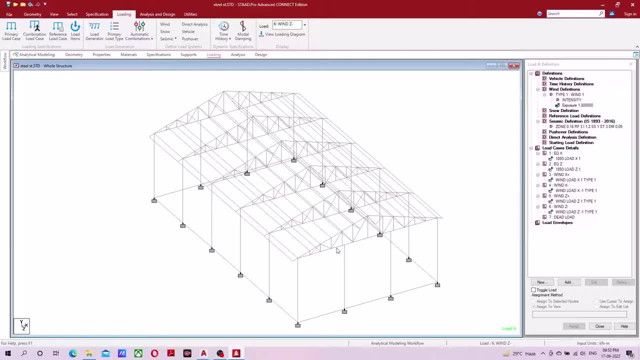 Because there is no live load here, Because your flooring is below, There is no floor here. So sometimes we will go up for maintenance. But for that we are factor of safety, For that no extra live load is necessary here. So after selecting the dead load, We will simply add it. 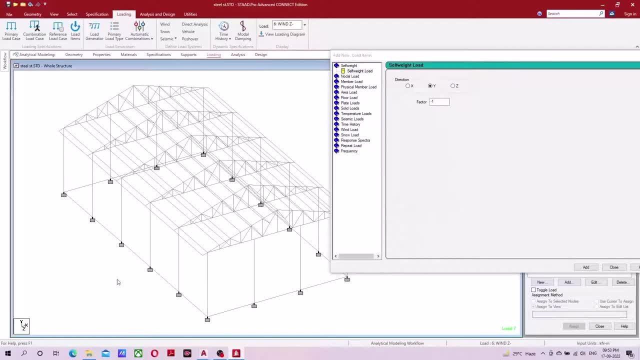 After adding Here, the dead load will come first: Self-wet load. Self-wet means This load of total structure. This load is your individual member. It will calculate and apply all the weight here. So here I will select self-wet, After that I will simply add here: 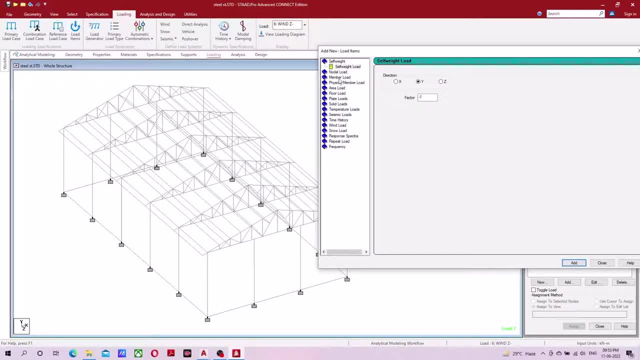 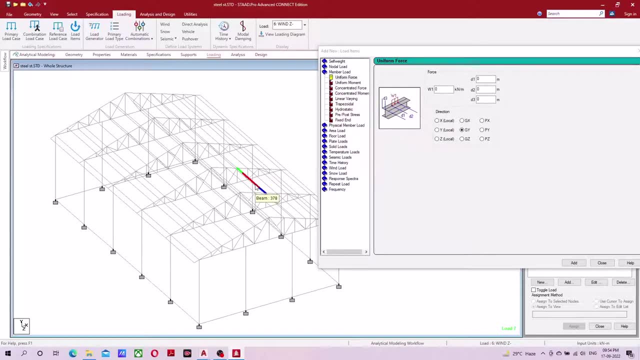 After adding Here, I will take the next member load. I will apply this member load only on perlin. I will apply it on perlin because What happens on perlin? There is a seat, There is a seat of GIS, There is a seat of ACP. So the weight of the seat: 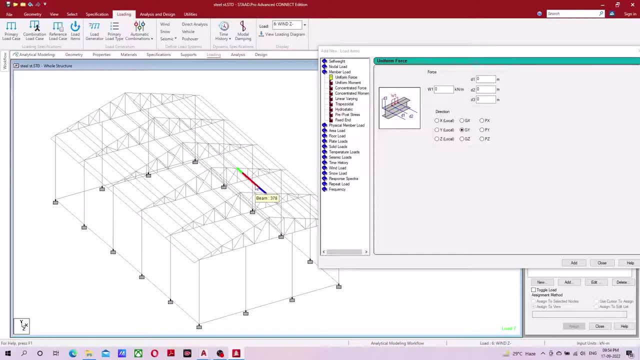 And sometimes for maintenance, We go up, There is a rainfall, So by combining all these loads, Uniform force. here I am applying minus 0.1 kN per meter, Including all loads Like self-wet of steel seat, Rainfall And snowfall If there is snowfall. 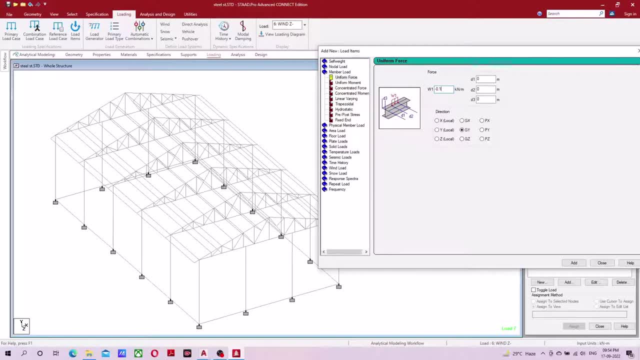 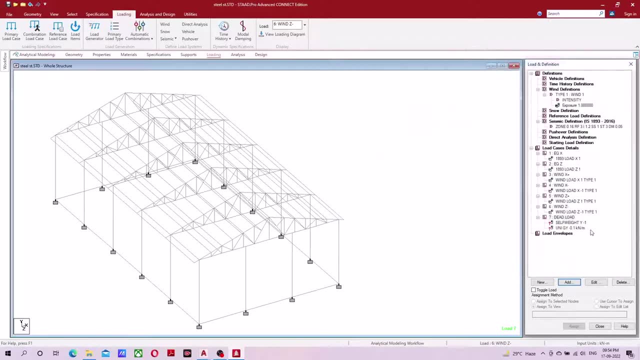 So here there is snowfall, So ignore it. So for all this Here, I will apply this 0.1 In member load. I simply want nothing else here. Add and close. Now I have to assign these two. Here is the question mark. If you assign, it will go away. 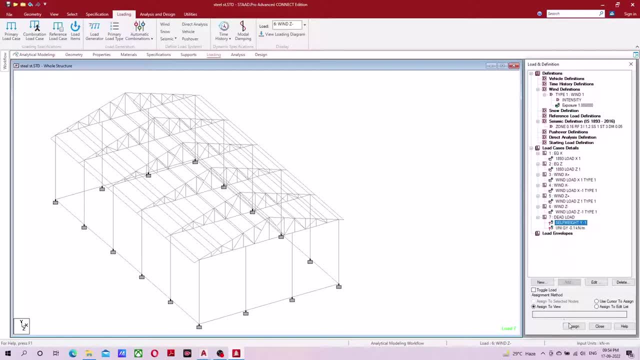 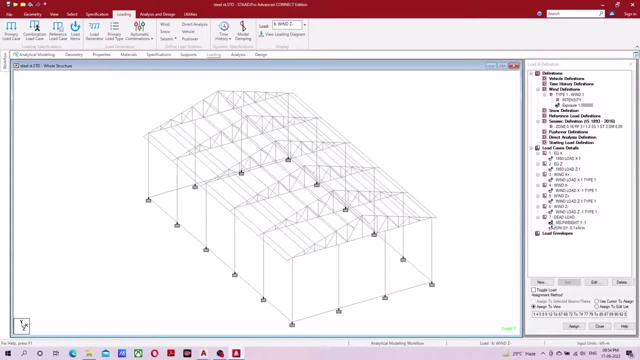 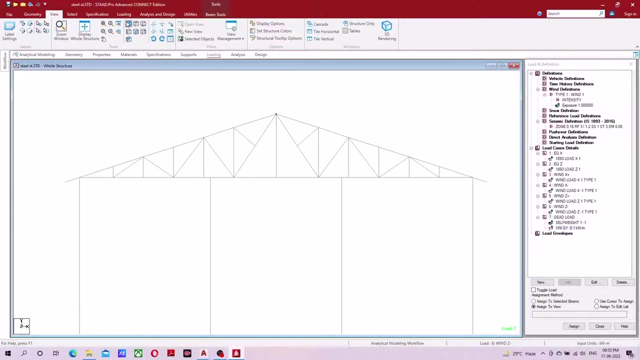 After selecting this self-wet Assign to view Assign. yes, Your total structure is applied. That's why it's highlighted here. Look here: Your question mark is removed. After selecting the second, I will select it on perlin. How will I select on perlin? simply, here I go to the front view. after going to the front view, if I press control and drag it like this, then, see here, this member will be your selection. so go to the front view here, press control and drag all the joint points like this and select the first one. also like this, only upper part, lower part. we will not apply. like this, press control and select it from the beam cursor, not node cursor. select it from the beam cursor. see, this selection is done. 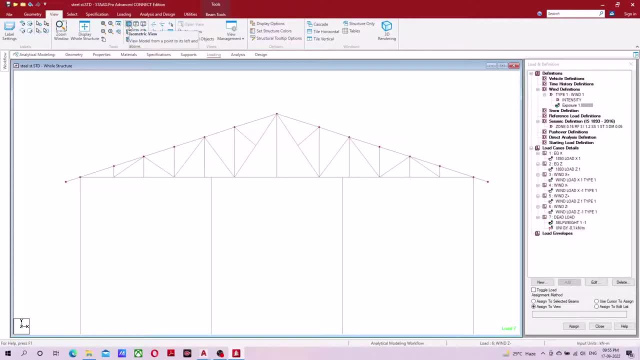 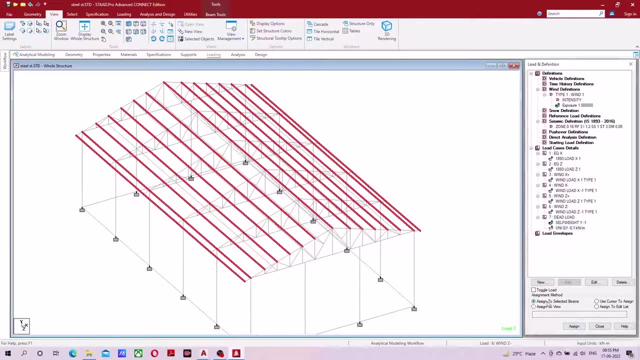 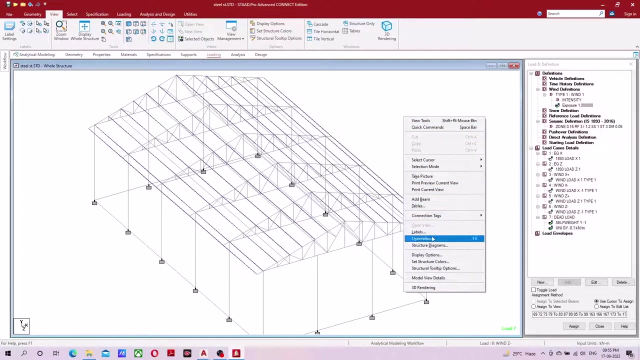 check a little on the isometric view. select it with control press. check on the isometric view. see this: the selection is done properly. after that, here you do assign to selected beam, do not do view. if you do view, then selection will be done in total. assign to selected beam, assign. yes, so see, this you have done, but it is not looking good to see it right. click after that. click on the level here. so click on light. click on your level here. after clicking on the level side it here, click on scale. 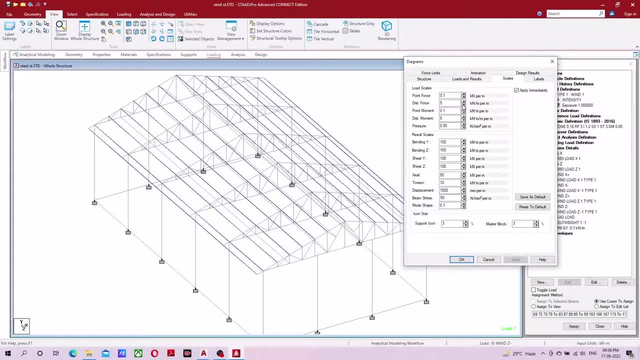 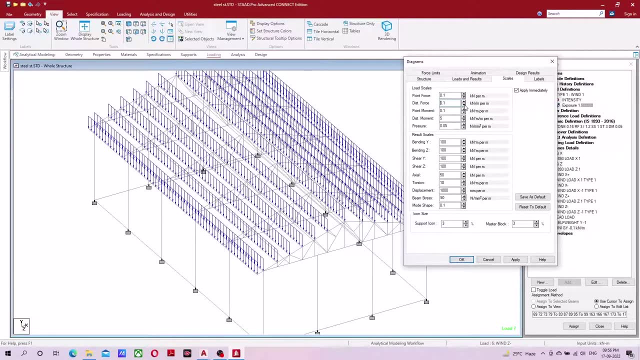 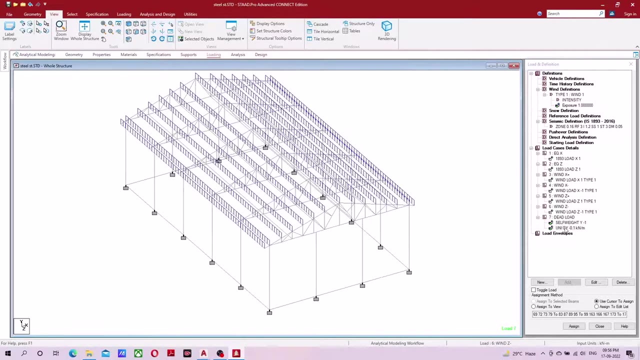 click apply. immediately reduce the distance force. if you reduce it, then you can see this animation, if it is visible. if it is not visible, then you can see it with this process as much as you want after that. ok, see, your application is done. see, I have applied all the load. 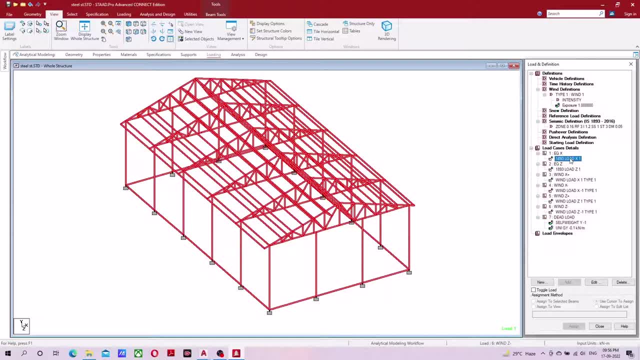 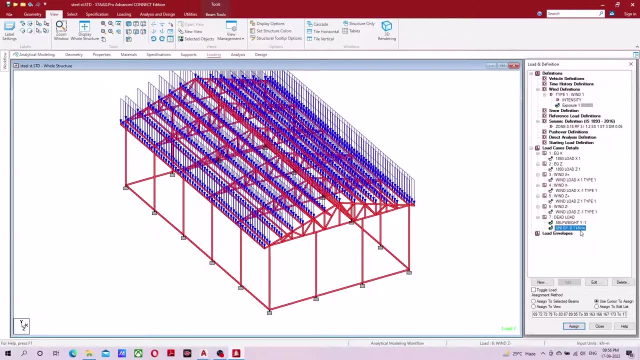 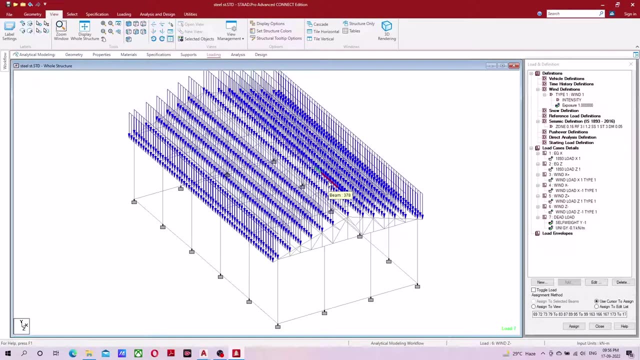 no need of live load. because there is no requirement of live load, I have assigned it in 0.1, including maintenance. after this, we will do load combination, factor of safety. we will provide factor of safety load combination. this is very important for this. you go to load case. 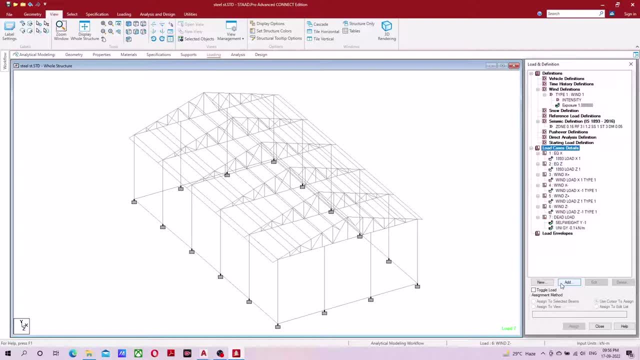 I will not go here and there, I will not explain it much. this video will be very lengthy. for this, I will go in a simple way. you can design it in a simple way. if you want full description, if you want full detailing, then comment it and also make a video on it. 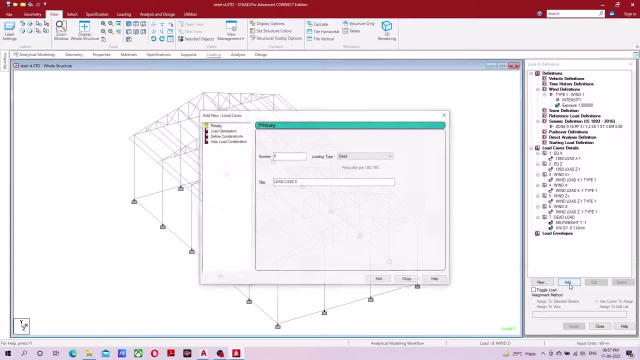 after clicking on load case, simply add. after adding, two types of load combination can be: 1 is define combination, 1 is auto load combination. I always prefer define combination, so you can define load according to you. after going to load combination, first select on dead load, after that click on fast option. 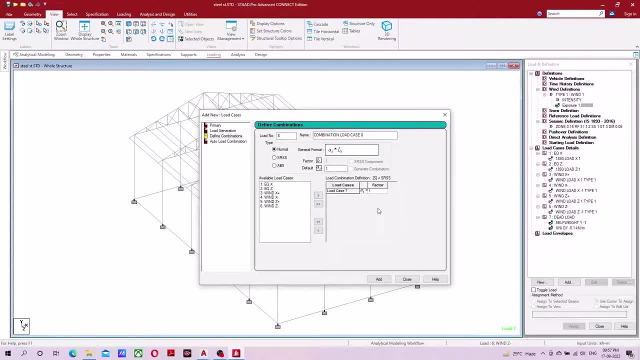 this is my transfer. you provide factor of safety 1. add it again. transfer factor of safety 1.5. add it. this combination I am providing according to IS code. according to IS code IS 875, part 5. in 875, part 5. this is your mention. 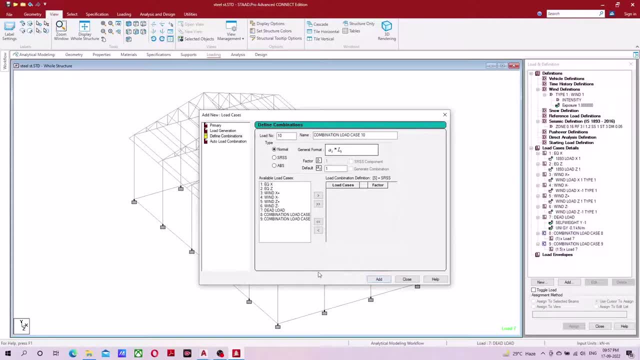 follow it according to that I am providing. after that second combination, select the first sesmic press control. click on dead every time. you don't want 1.2 here on default, press 1.2. after that, first one dead load transfer 1.2. 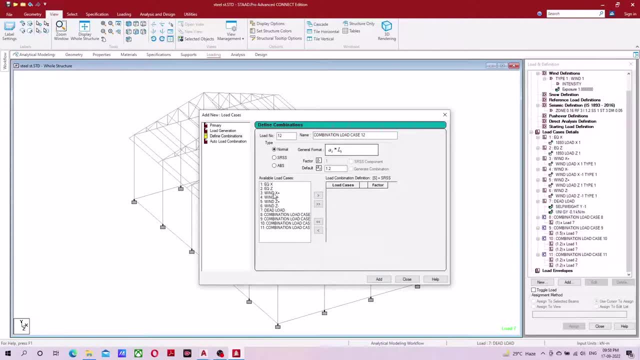 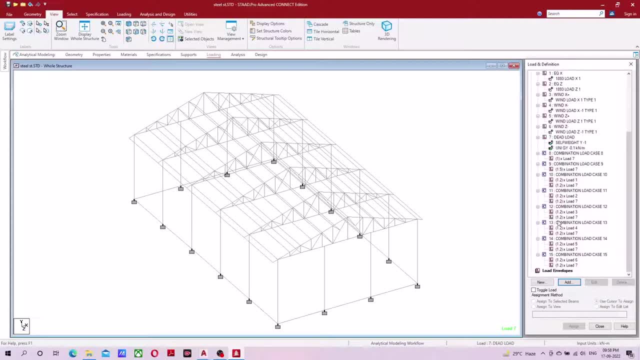 the more 1.2, the more 1.2. factor of safety. factor of safety is equal to working load divided by ultimate load. working load and ultimate load ratio is factor of safety here. convert working load to ultimate load. ultimate load equal to working load multiplied by. 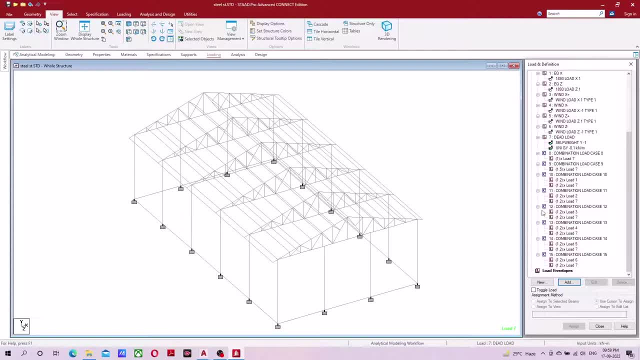 multiplied by factor of safety. so we did that here. so after that, my process is complete. after that, what will you do? oh no, it is not complete. after that, if you have provided sesame, then you have to follow one step. it can be a little difficult, so see it carefully. 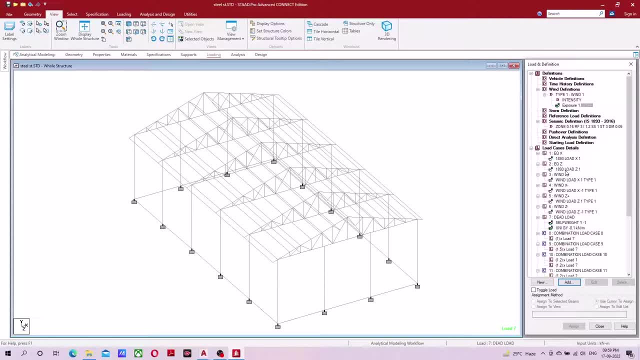 if you have any problem, then rewind it and see it again and again. then you will know this step. it can be a little difficult, so you can easily do it. follow it exactly like this. what you have to do, you have to go to utilities. after going to utilities, click on command file. 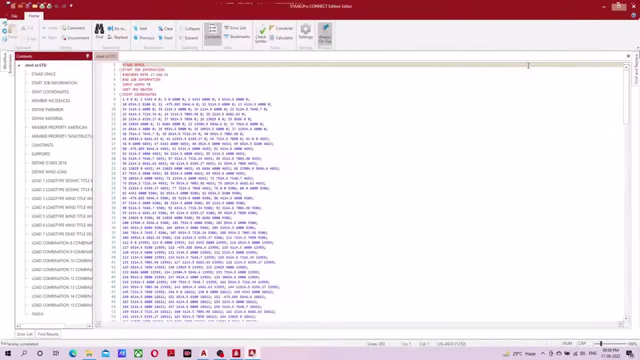 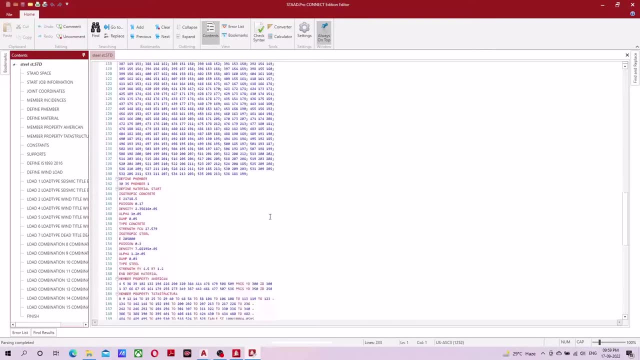 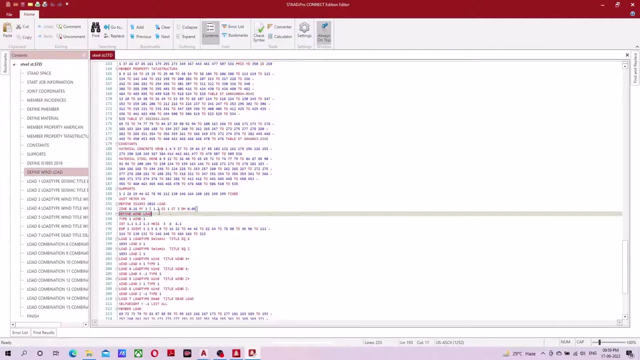 simply save. after that this command file page will open. after that you come down here. you have to search something. after coming down, you have to search one line, which line I show you here. see this line carefully. you have to follow it. see this line zone, note it down. 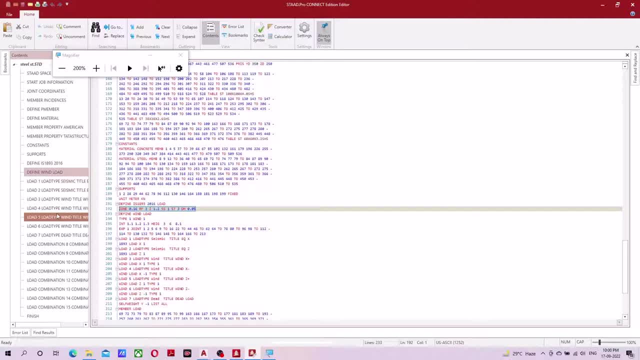 this line zone 0.16, RF3 I. so this may be different, but here the first letter will be written as zone 0.16 may be. if your zone is 0.1, then 0.1, 0.36, 0.24. 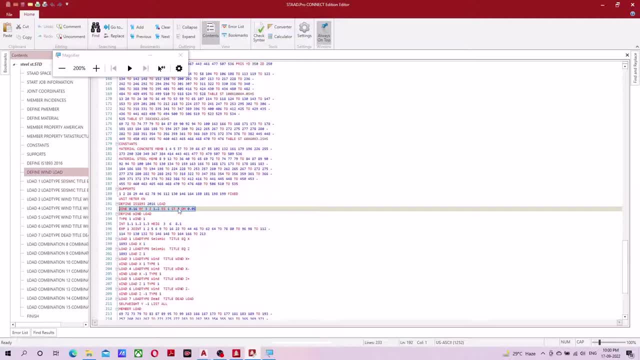 can be changed here, but here with zone, this line should come after coming: this much press enter. press enter because I have to copy something and paste. so I will copy something and paste and here if you come up, then here is an ad option if you click on it. 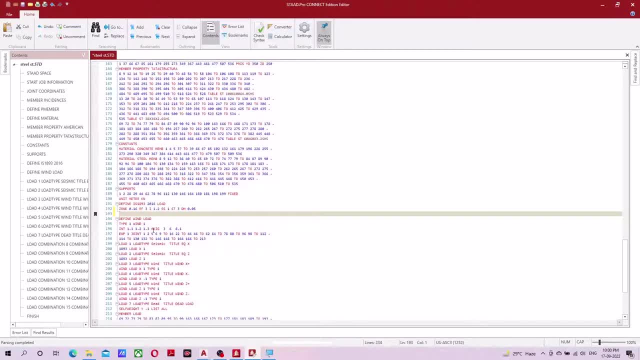 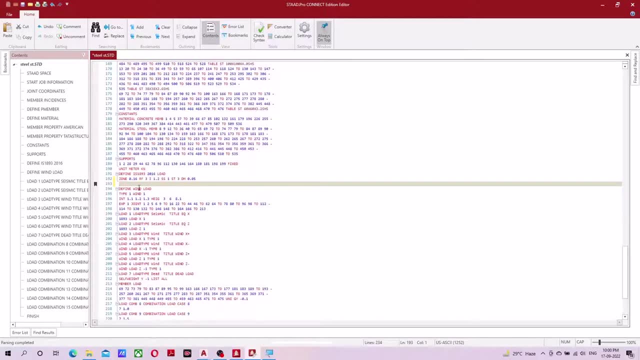 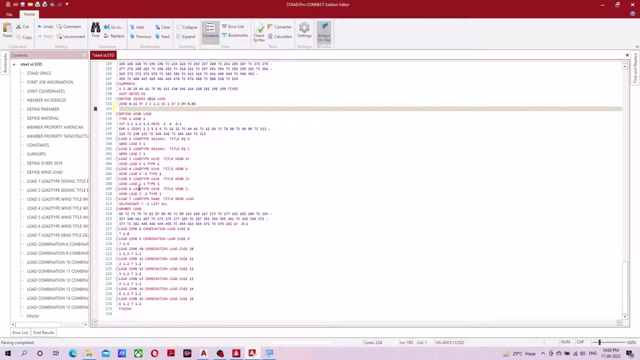 then a mark will come here, so you will be anywhere. you will be anywhere. then you will come to know that I got this line. I have to paste here to know who to paste. you come down a little, come down a little more. here you have this dead load. 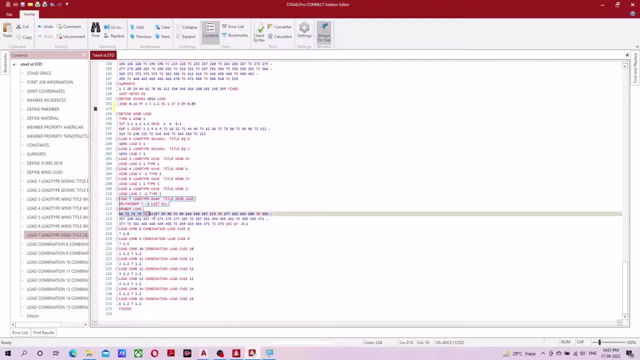 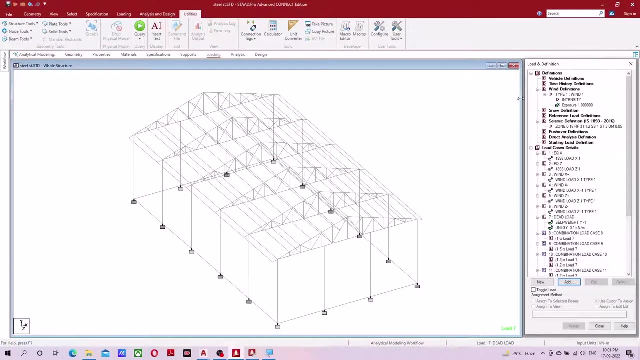 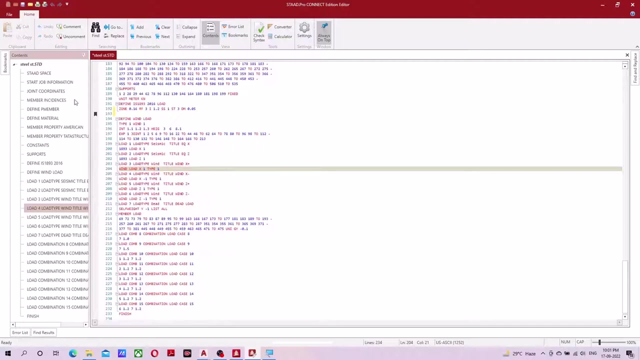 dead load. see here, dead load. how much was the dead load? here was my. what load after wind load, what load did I provide? load number 7. ok, if it is confusing, then here you have to minimize after minimizing. see here, see here, here it is written: load number 7. 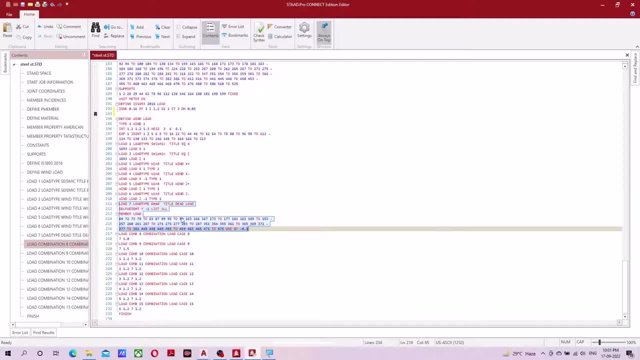 which is my dead load. this is my dead load. below my start was combined load, combination load. so this load has to be copied. from where to copy, leaving the line above dead load which is below start, from self weight up to its ending. you have to select it. 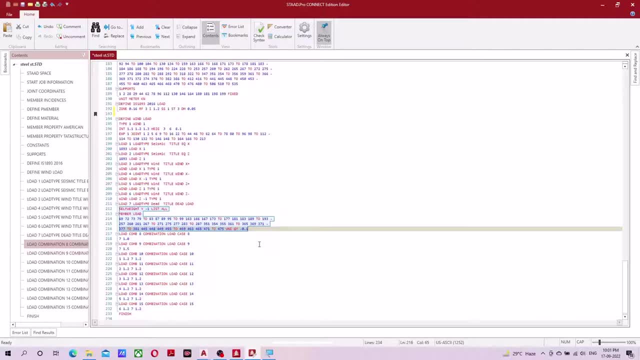 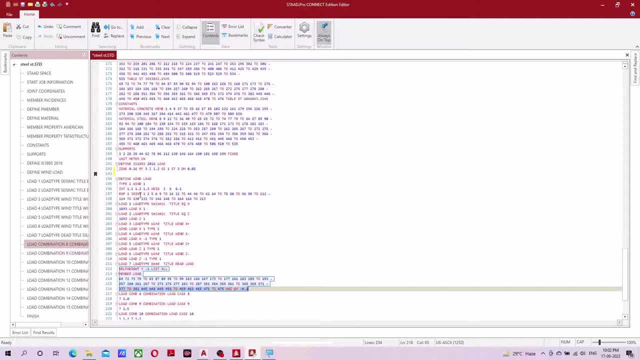 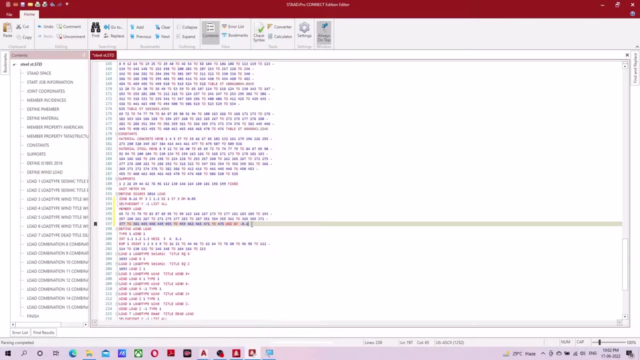 I will upload it in this video. I do not include it in this video, so simply select it. copy it to ctrl c. after ctrl c, where I had a bookmark, by clicking here I will do ctrl v. ctrl v will be pasted. so from here to here, 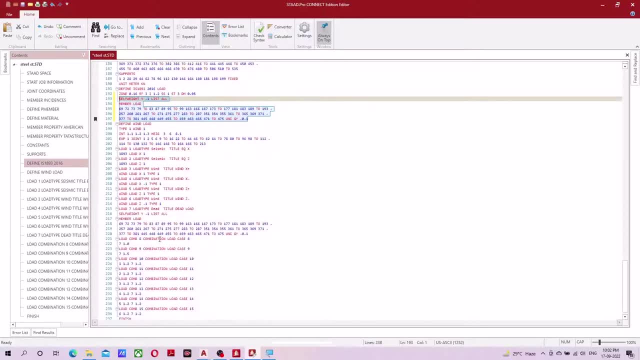 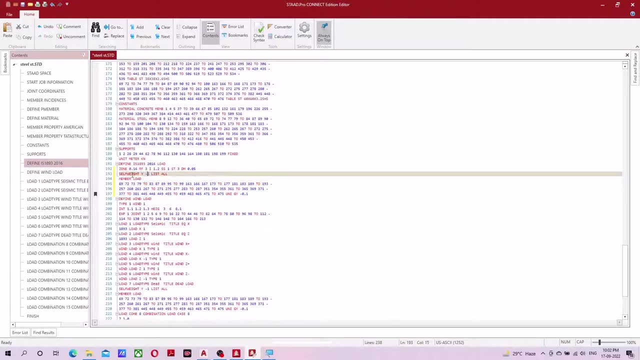 it is pasted: see carefully. original is also there, but here I have a duplicate created. this duplicate created after the self weight y and minus 1. this has to be removed from minus and this has to be removed from y. ok, this has to be removed from minus and y. 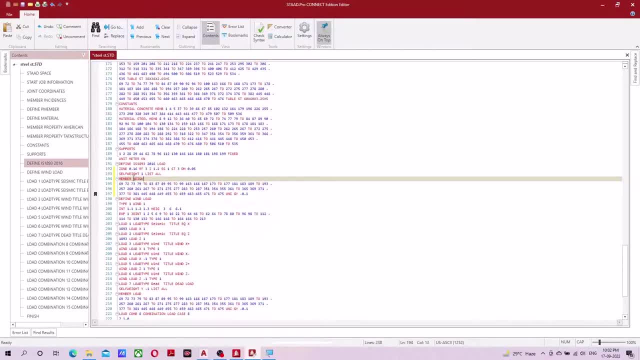 after that this load is written: write this load in capital weight: w, e, i, g, h, t. write weight. after writing weight, come here this last written: unigy01. this minus symbol has to be removed and this g y has to be removed, simply after unigy01. 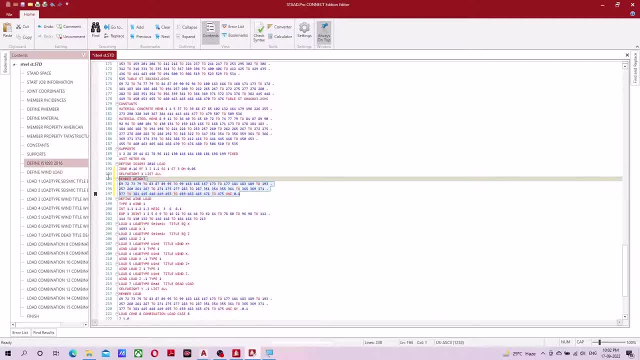 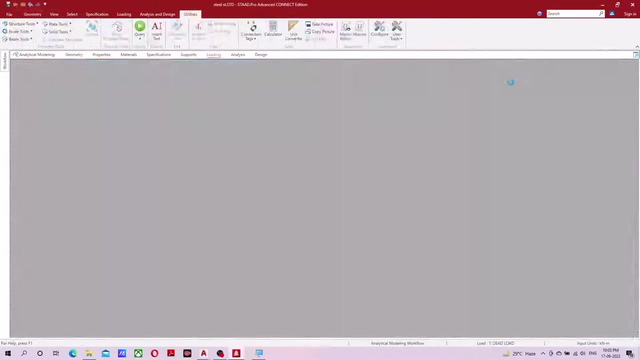 this number has to be removed. so this much you have to modify here: after self weight: remove y-1. here member load write weight. after unigy01: remove g, y and minus. after this, simply here click the save option and press ctrl s. after this, close it. 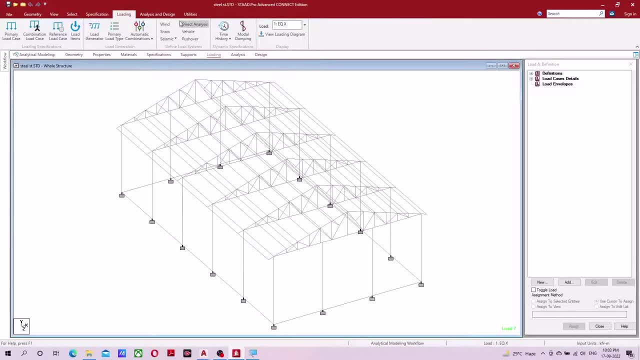 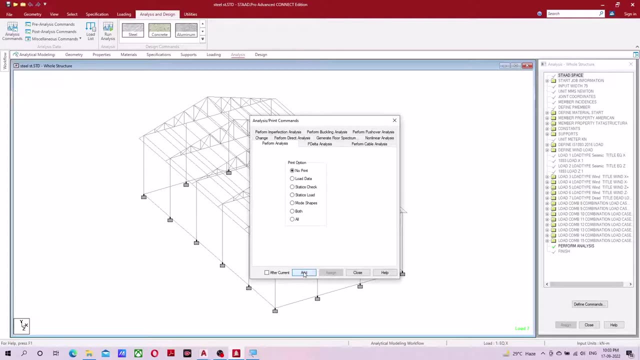 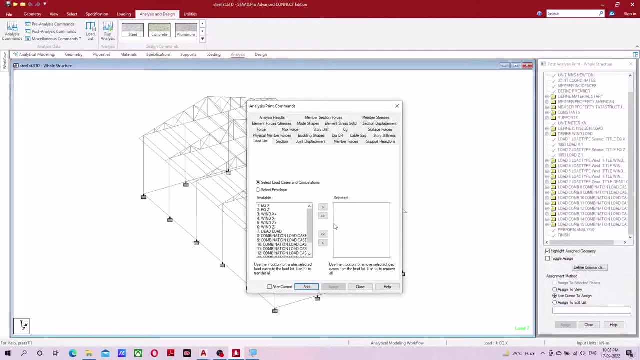 now what we will do simply here: go to analysis and design option. select analysis command. after that add and simply close it. after that post analysis command. after that define command. after that transfer this load by the help of this second option. after that add it. after that select support direction. 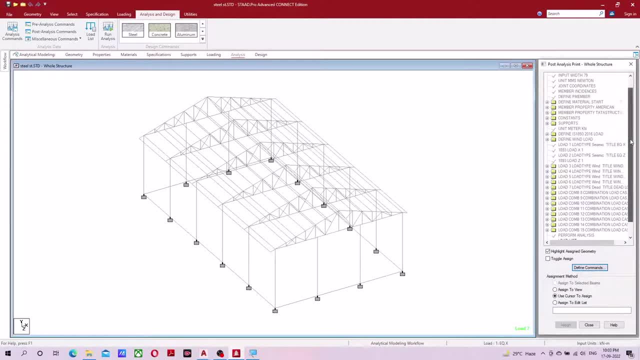 add and close. after that, scroll down. there is a question mark on support direction. simply select it and assign to view. assign: yes, so this much step is completed. after that, click on run analysis. save it. see here, there should not be any error. one warning will come. ignore it. 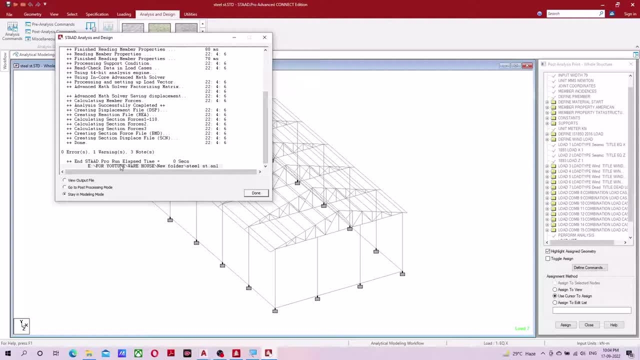 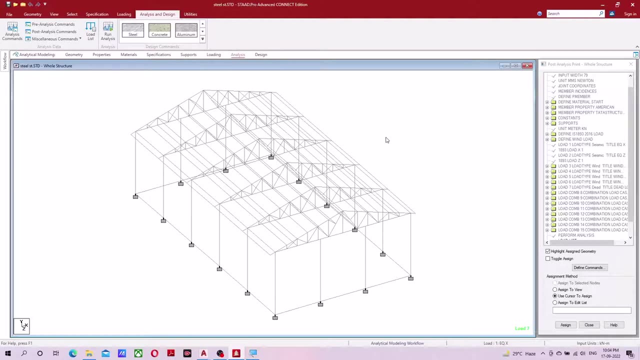 except that there should not be any error. two or three warning will come, but there should not be any error, one warning, default will come. so this much is done here. after that, that means my load is complete. load process is complete, if any member, if I have to calculate. 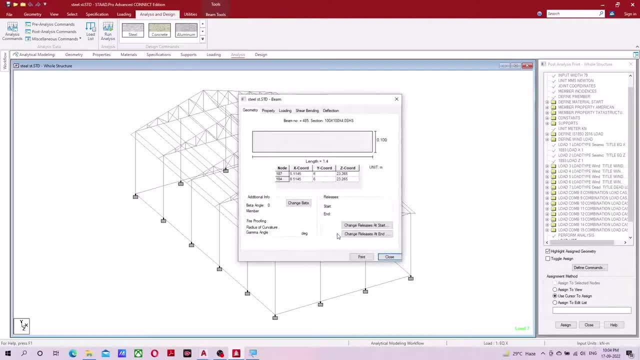 pending moment: shear force. then simply double click on it. here you can check deflection. you can check shear bending for this you will check different video, but here you can check on any member. double click on it here. shear bending: shear force for different load and its bending moment. 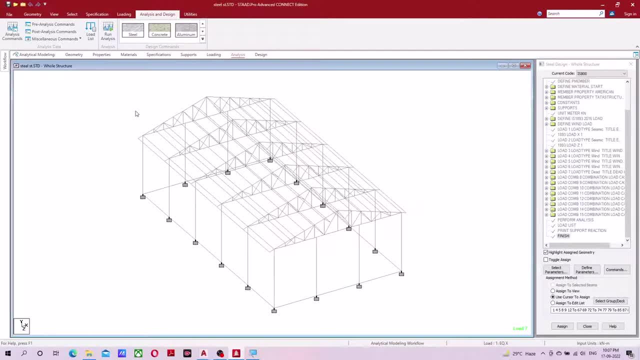 I can check here. after that we will follow the last step. what is my last step here is design. after coming to analysis and design page, click on steel. I have to design steel. click on steel. after clicking on steel, choose current core is 800. this is my last step of steel design. 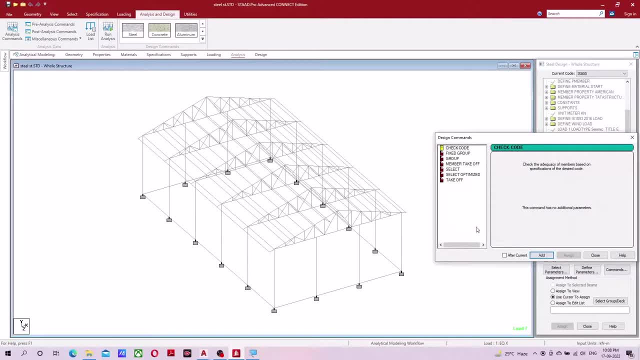 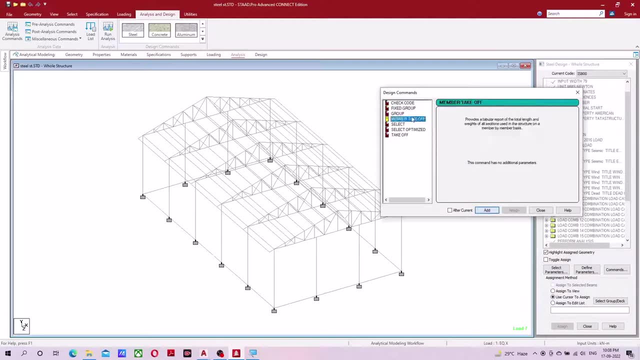 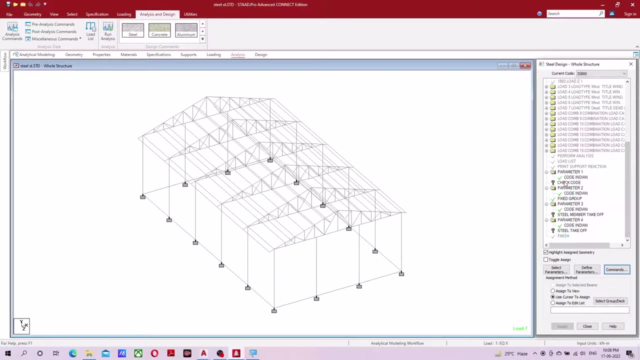 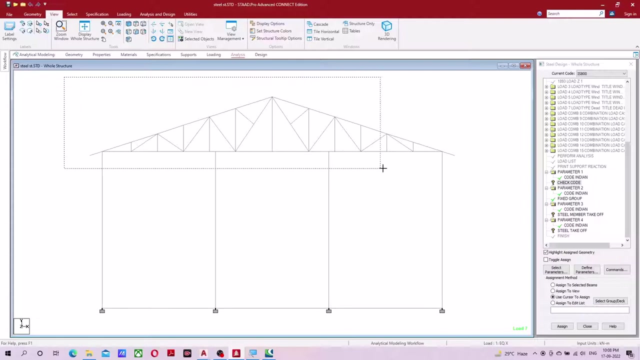 after that, click on command option. after clicking on command option, first of all, check code. add fix group, add member takeoff, add takeoff, add this much you have to add. after that, come down here. you will see question mark. after selecting it, go to front view. here is your steel member. 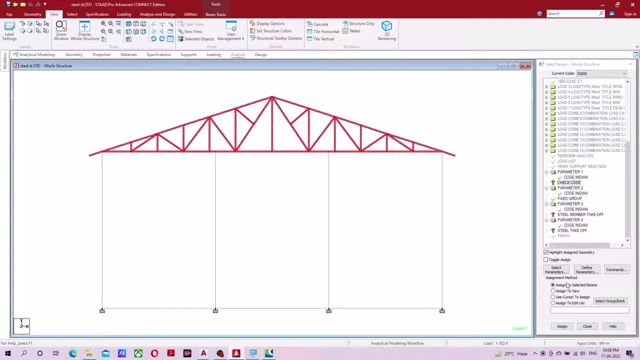 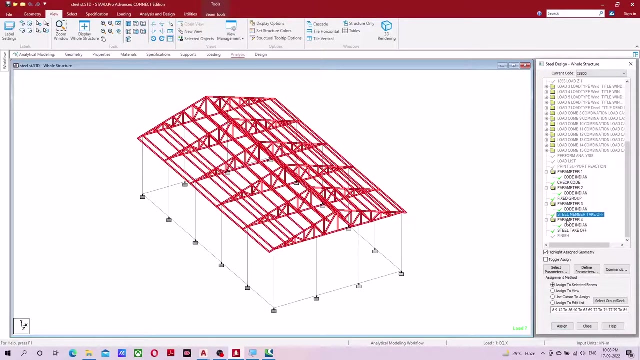 select it like this: this is my steel member. rest are of RCC. after selection like this: select it like this. select it like this: assign yes. next one: select, then assign yes. like this: I choose it. see this. whatever it was see here. this is my highlight, this is my selection. 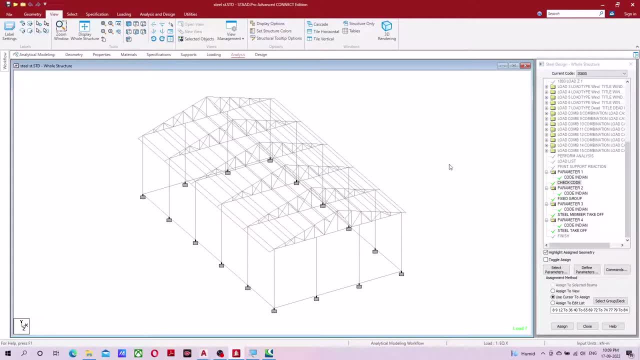 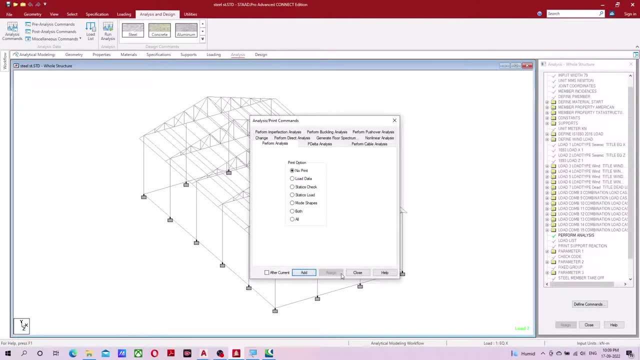 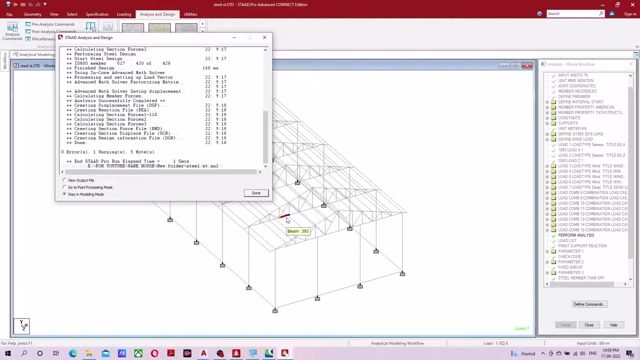 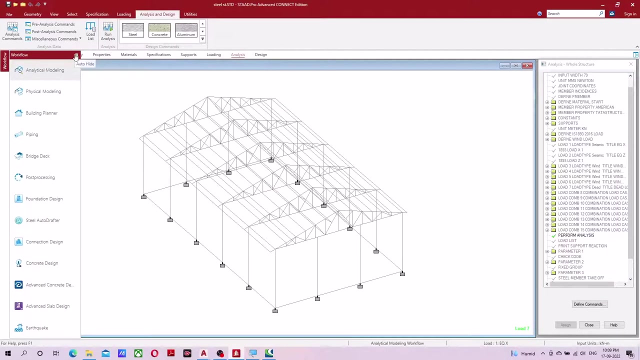 this is my highlight. after this, after coming to analysis and design, again click on analysis command, add and close. after that, run analysis. save it. now our steel design process is complete. how to check the result? after that done it, click on workflow. click on it. go to post processing. 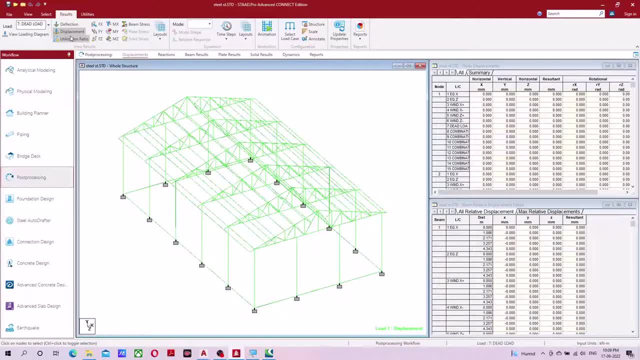 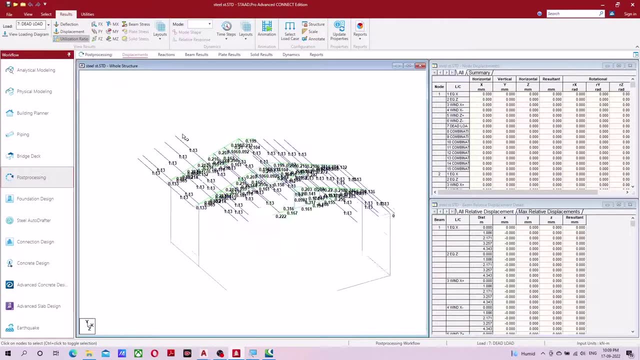 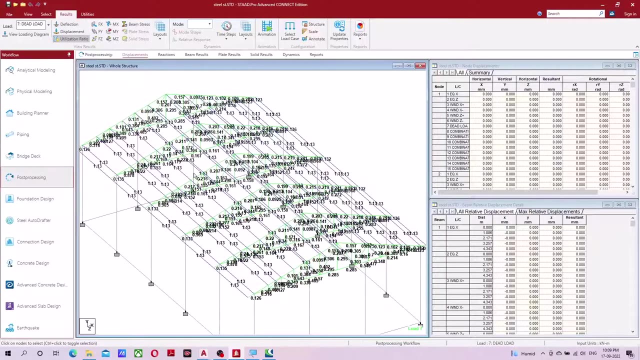 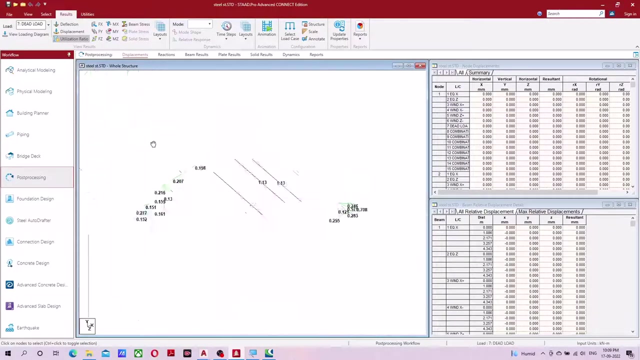 after that, simply ok after ok. uncheck the displacement unchecked. click on utilization ratio. after clicking here. basically this is the upper part, ignore the lower part. here basically three colors show. first color is red. if it was red then it would have failed completely. here no red color is showing. 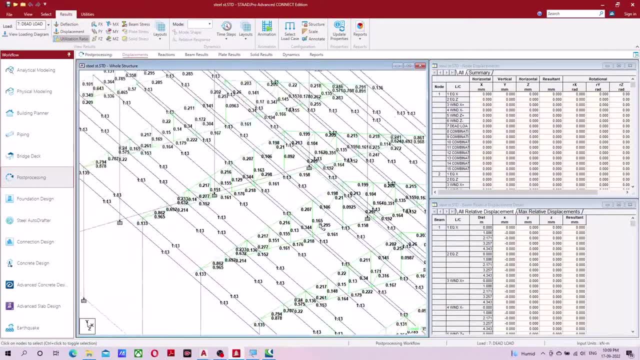 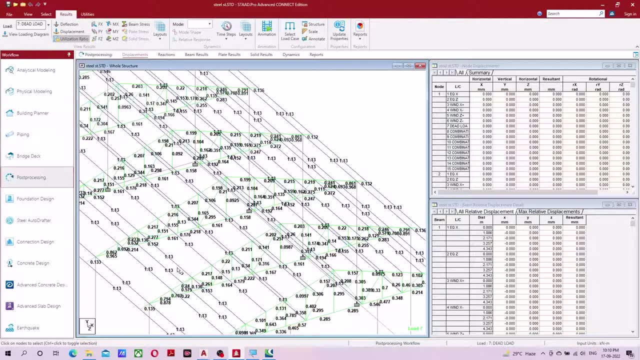 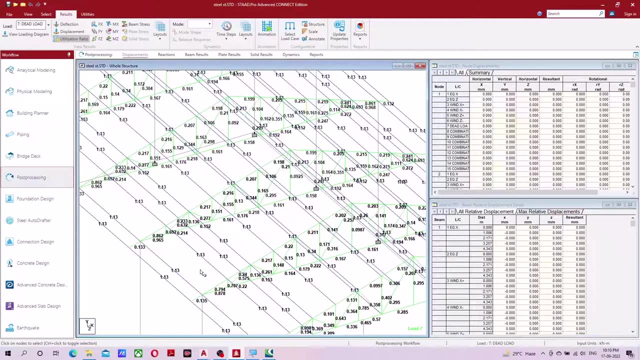 so my structure is not completely failed. see here. so red color is not showing. second color is blue. what is blue color? it is approximately failed. it should be below 1. it should be below 1. below 1 means 100% pass. see here: 1.13. 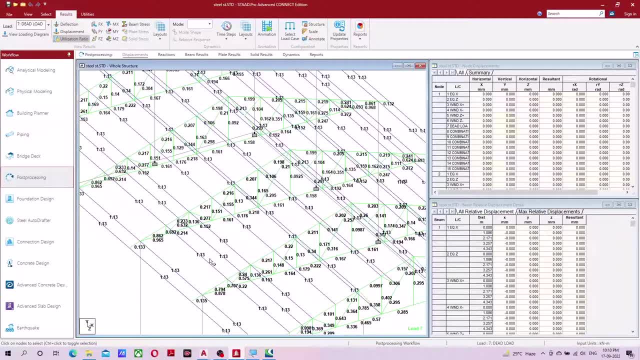 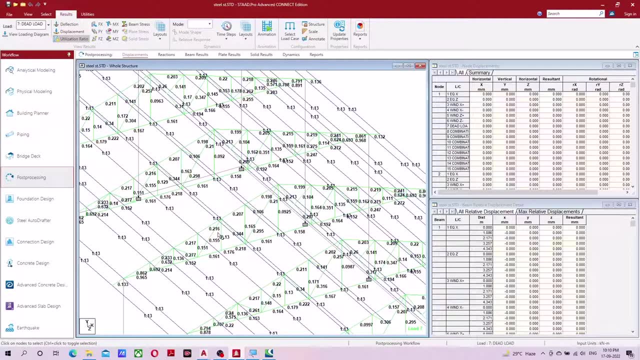 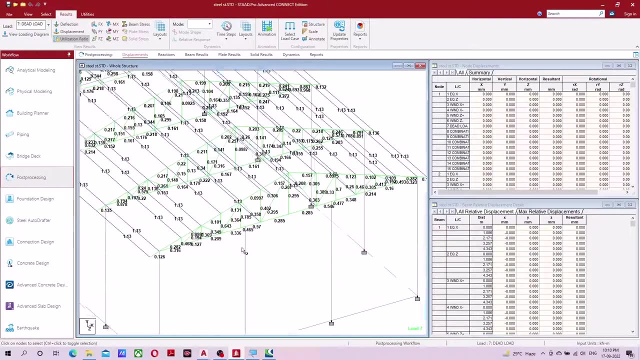 means it is almost pass. it is still failed, but after increasing a little it will pass. next color is green. green color is always below 1. means it is 100% pass. means it is 100% pass. here three colors show. we will check the ratio. 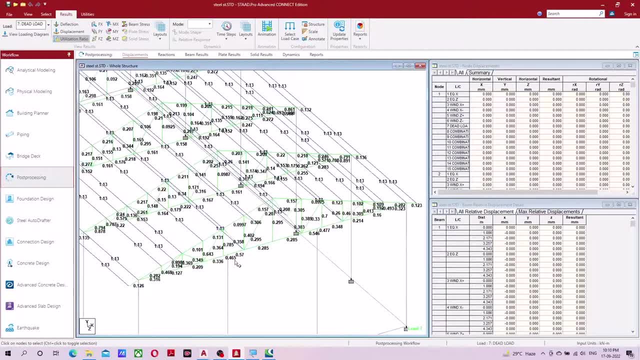 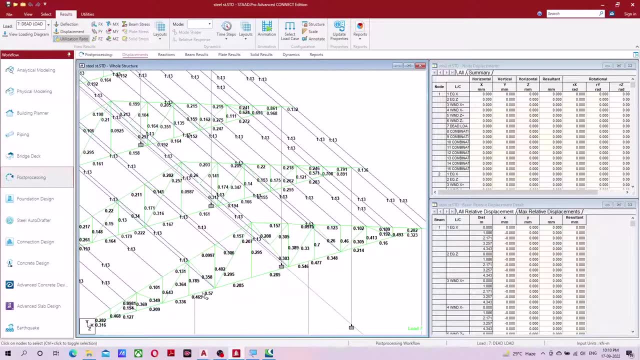 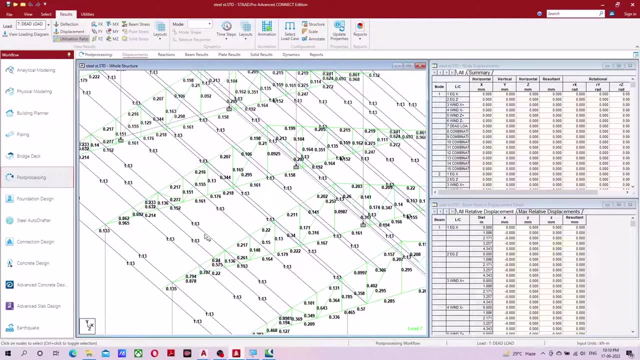 ratio should be below 1 here. the ractor and tie member and the secondary member, all these are passed. sorry, ractor and tie, beam and secondary member are passed. I have to increase the porlin and tie member property to pass. so what I will do, simply again come to property. 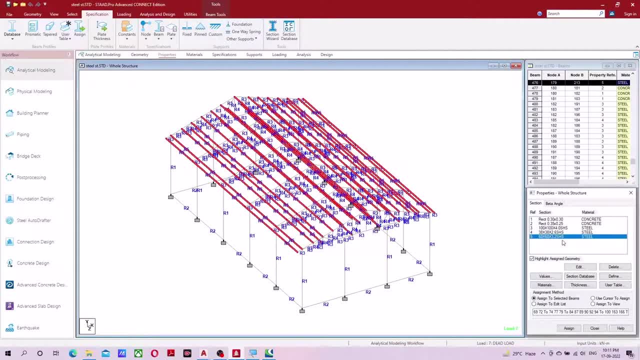 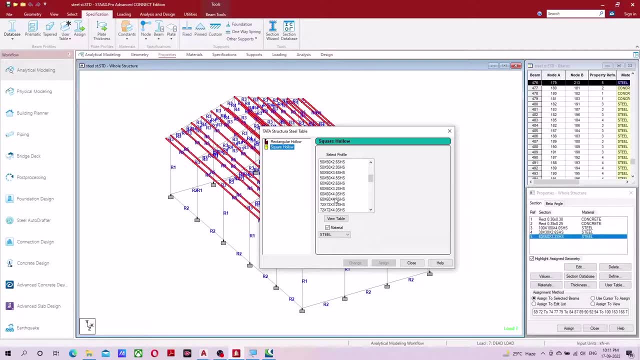 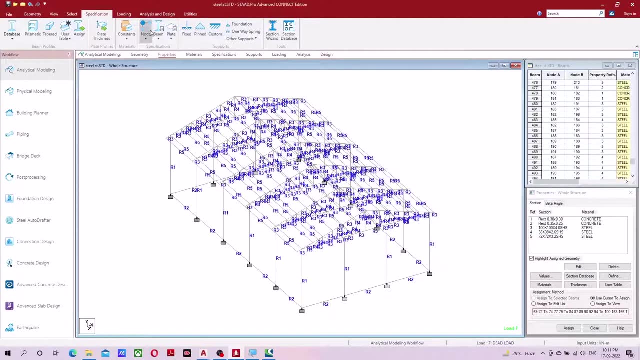 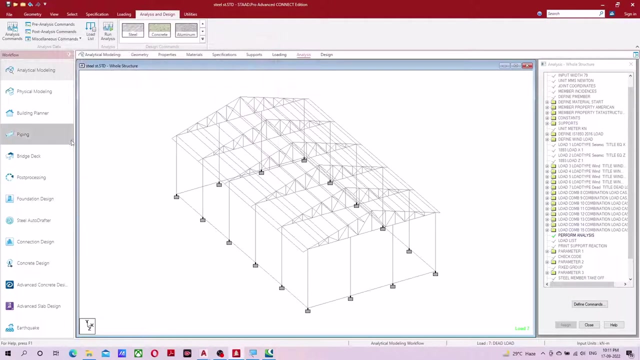 the property. I took this one: 6060, 3.2. this one is failing. I will edit this. I will increase this 60 to 72 to 3.2. add after this: run on run analysis: simply run. if you do not run, then the result will not show. 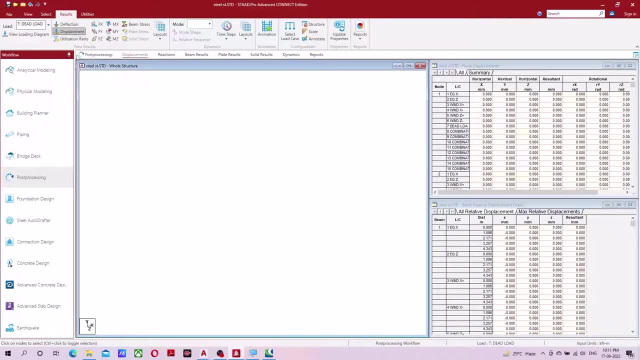 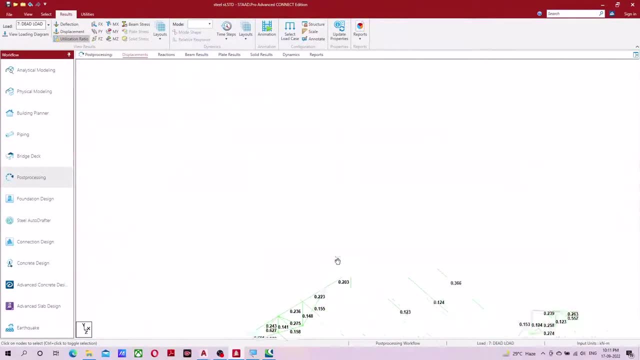 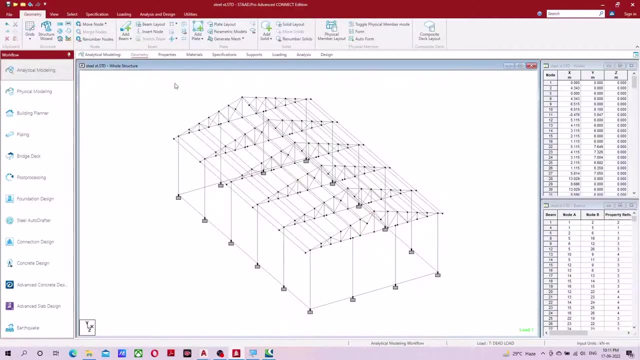 after completion, again come to post processing. ok, you have to remove displacement. after that click utilization. you have to pass this. if it is not passing, then you have to increase again, again, increase, suppose. if I fail something like the first one I provided, I will reduce this 100 to 104. 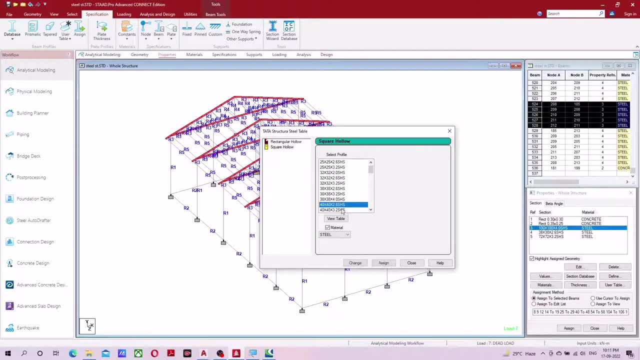 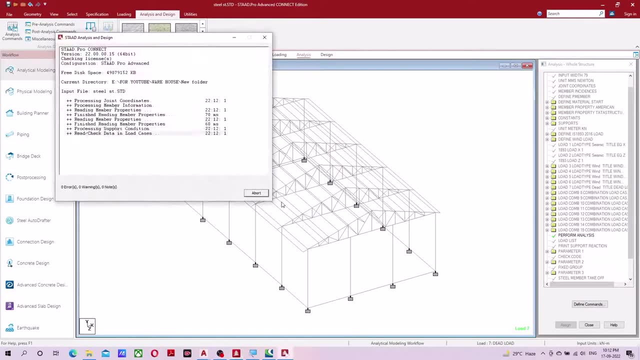 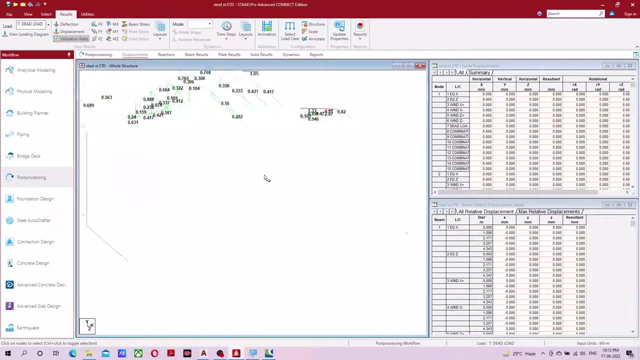 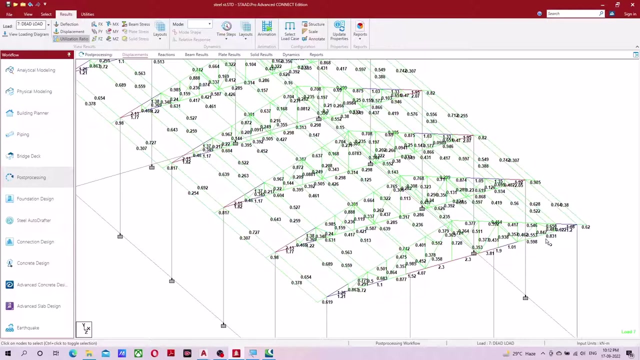 so that it will fail. this is 50 and this is 42.6. I will fail and show: I have assigned this now check. ok, see this. when it fails, something like this shows: see, this is on red color. the ratio is 2.3. this whole member failed. 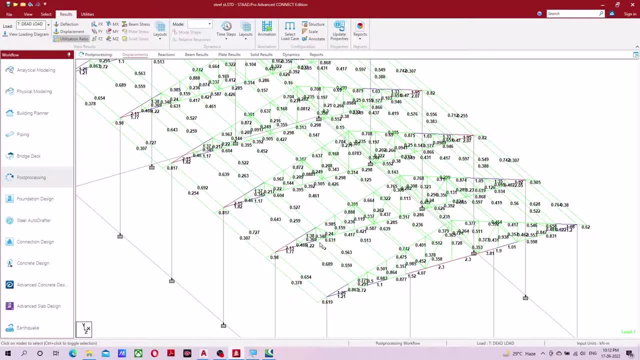 the upper member also failed. that means I have to increase the total. it is not like I will take it separately, so how will it join? this means this is failing. you have to change the complete member. if this is failing, then you have to change the complete member. 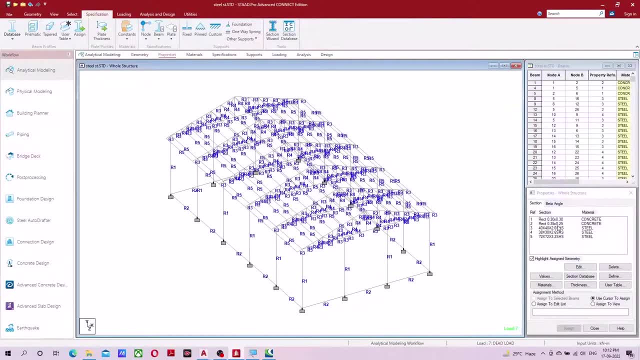 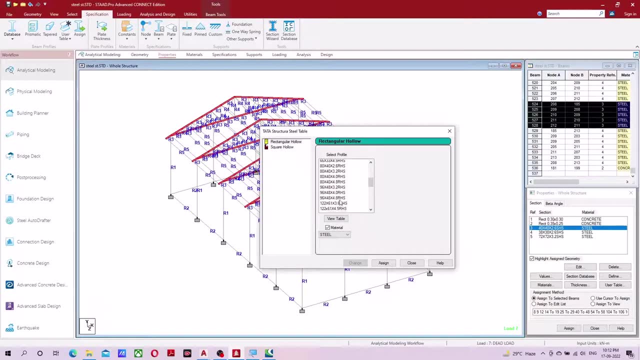 like this is failing more on red color. so whatever it was that was correct that I did 70 to 72. sorry, 40 to 40. I keep it 100 to 104. that is correct. this is only to show you what was where it went: 100 to 104. 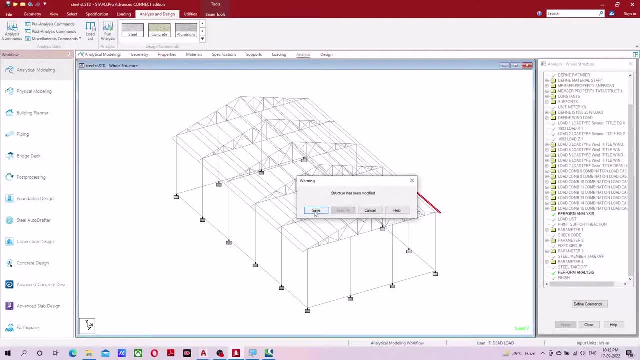 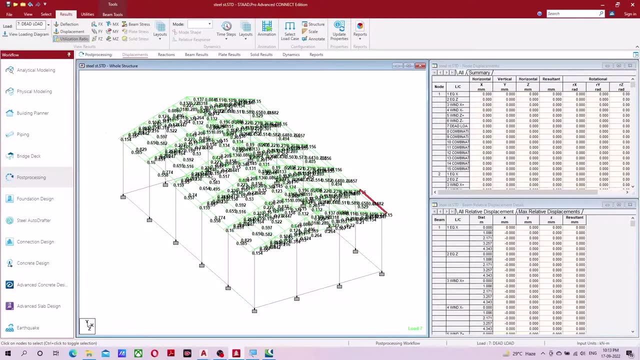 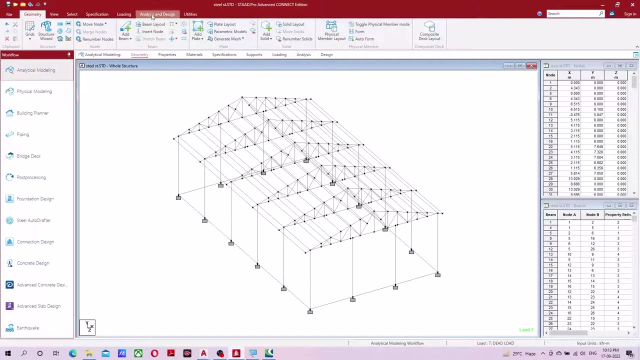 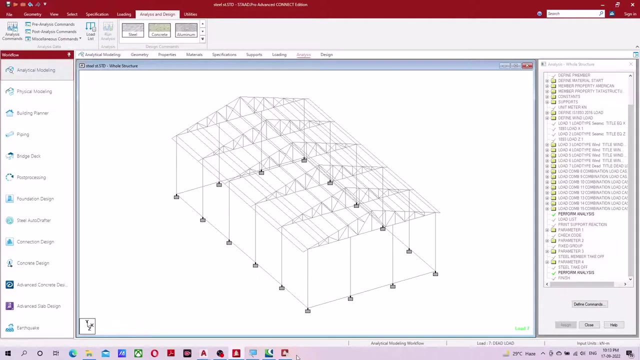 change. yes, after that again run. I will see it is correct or not. ok, post processing. ok, see here. my here is correct. all members pass here and you can check here here. you run after running. here will come an option view output file. done it after done, come down here. 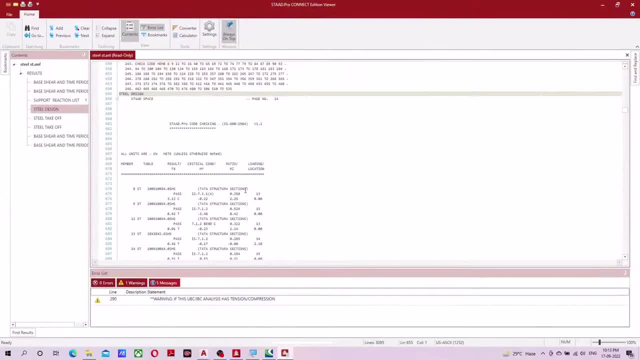 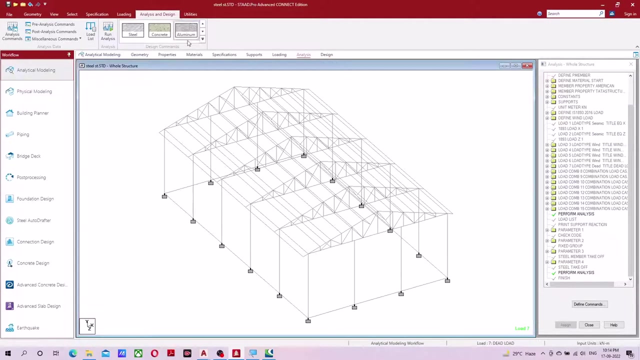 here you turn off the warning. here you will write: still design. double click on it. after double clicking you can see all of the pass here: pass, pass, pass, pass. I will design the columnar beam of RCC. I will go to the concrete. I will keep the design code as IS456. 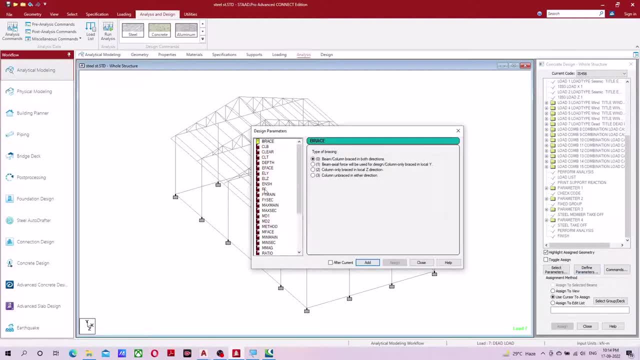 After selecting the design parameter. I will take FC in meter. I will take it as 25000. I will simply add the concrete of M25 grade. I will take FOMN as 500. I will add this much parameter. I will add more parameters in the complete tutorial. 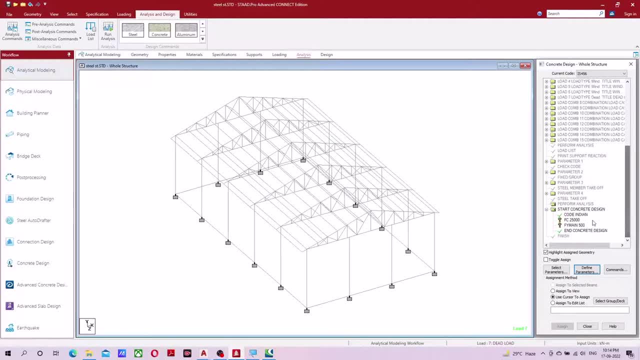 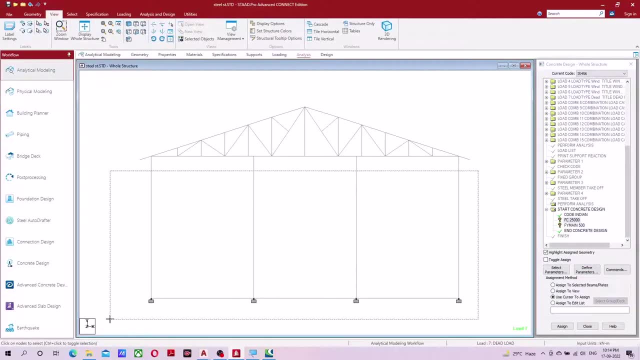 That's all for now. You have to assign this member. The first one is in the front view. Select the member of RCC. Assign to selected beam. Select the second one. Assign yes. After that, come to the command option. Select the design beam and add. Select the design column and add. 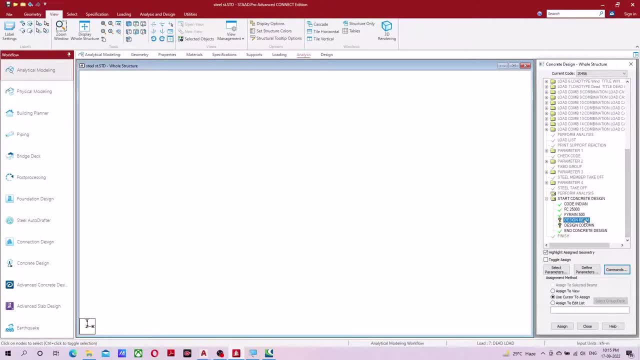 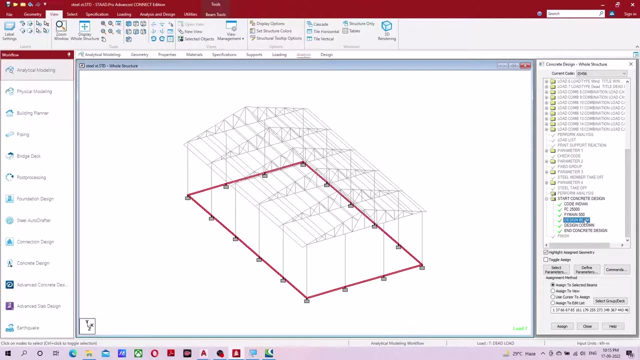 After that close. Then come down Where to assign the design beam: Select the plane beam below. Assign to selected beam, Assign yes. Where to assign the column: Select on the column. After that assign yes. So here I have designed the RCC. If you want to check, You can check design beam, design column. 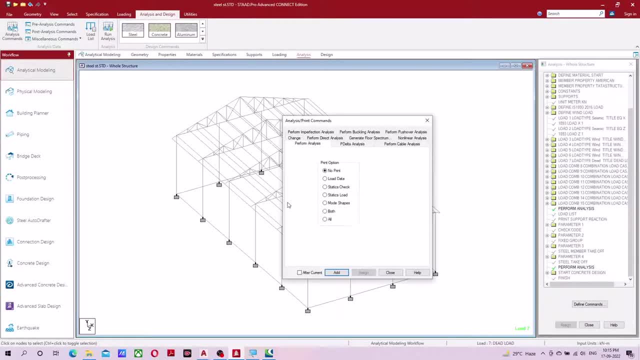 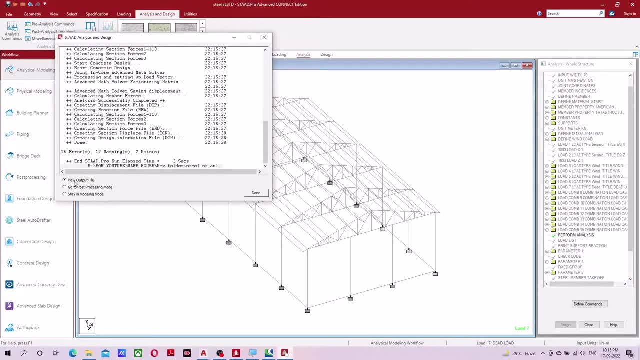 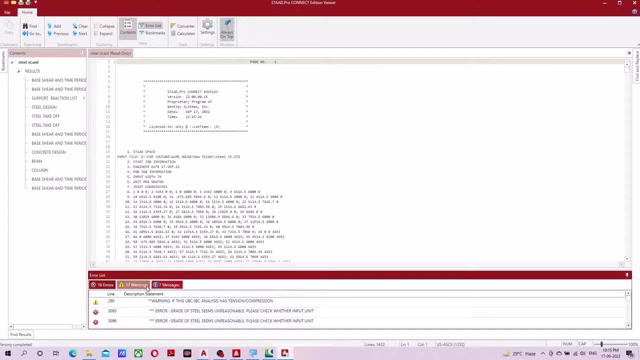 Again. you analysis command, After that add, After that close, After that we will run it again. So here I can check the RCC Here in view output. Here some error is happening. Let's see the error. View output done. The grade of concrete seems unreasonable. Here the grade of concrete is a little wrong. 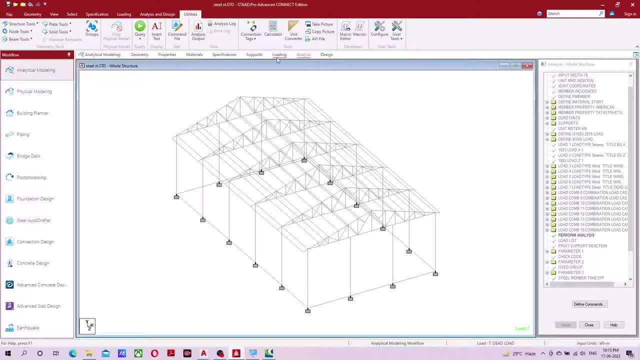 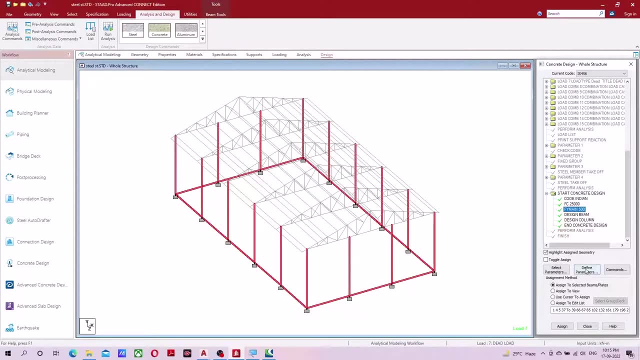 Let me see this. I will see this Here. I came to design Concrete Here what I provided. This 500 was taken Because it is in meter. This 500 was taken. This should be 500,000, 1,2,3 And 30: 0 should have been put here. 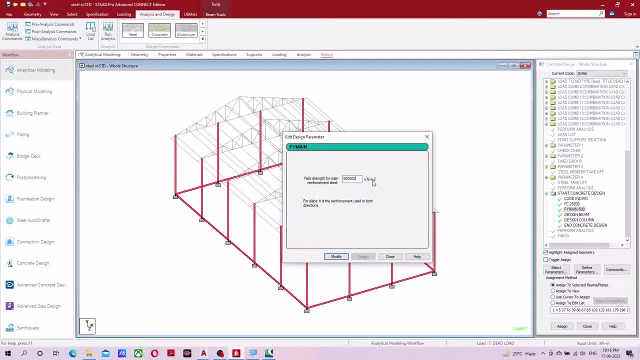 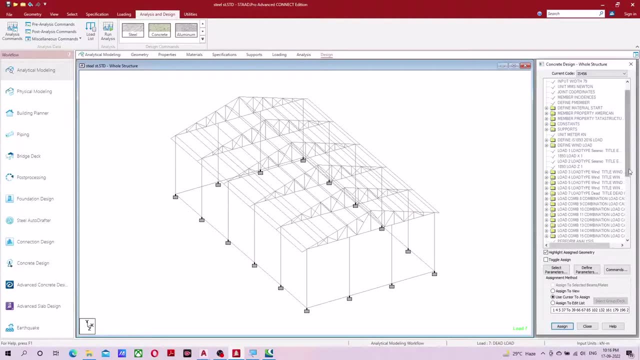 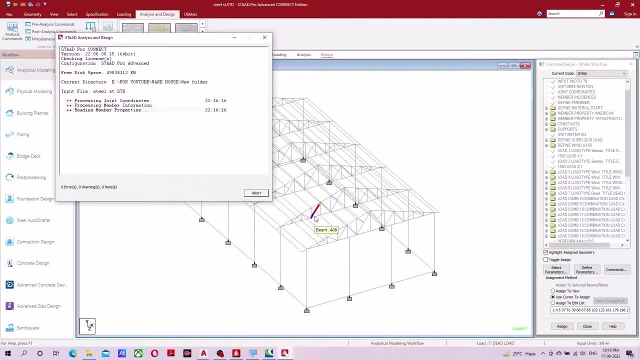 Because it is in kNm2, If it is in mm, If it is in Nm, Then it is 500, So I modified it. Ok, modify this 500,000, Run it after that. Now you check this, I will upload another video In which you can check the error. 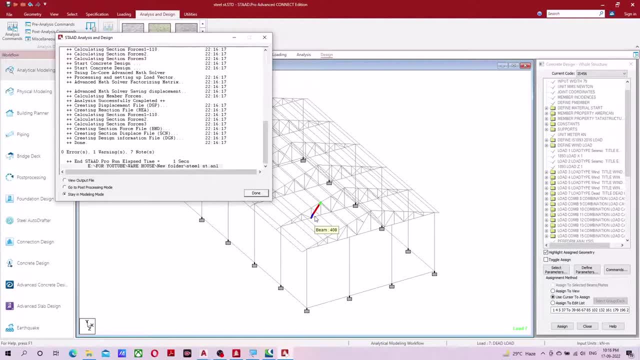 How error is created, How to solve error. I will upload video for this further. That's why I'm saying: Please subscribe this channel, subscribe to my channel so that in the future I will upload a lot of different videos like this which you can see. it completely start pro 3ds max, rafit, lumion, all software. 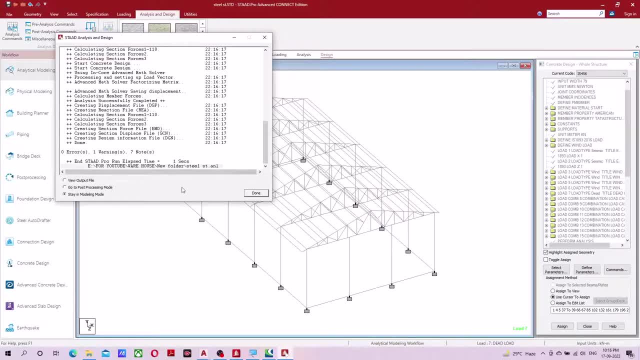 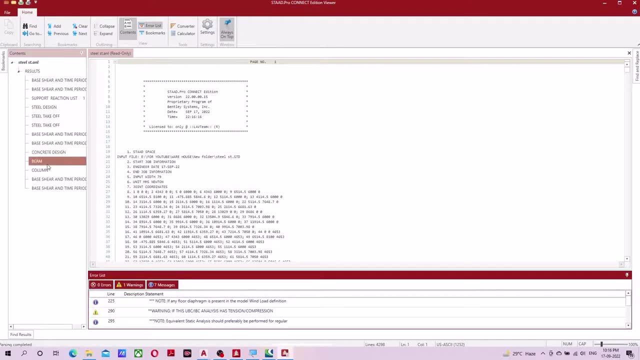 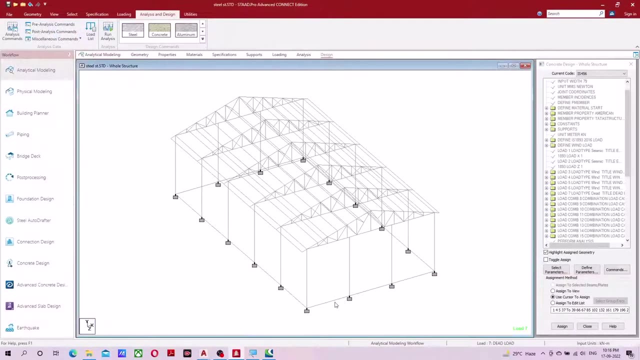 easily you can learn. so here it is view output. after that I done here, after done here: simply you double click on the beam. my result of the beam is showing here. double click on the column here. the column result is showing here. you can double click here. double click here: concrete design. this is the result of the beam. 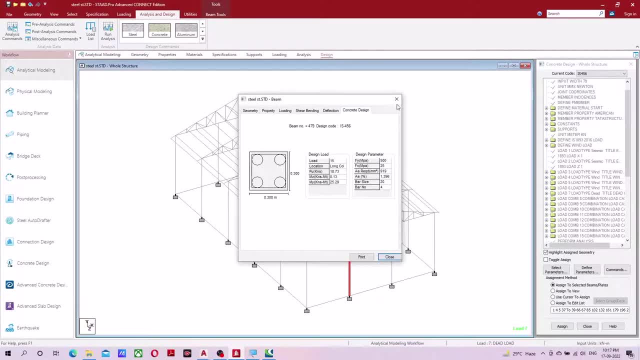 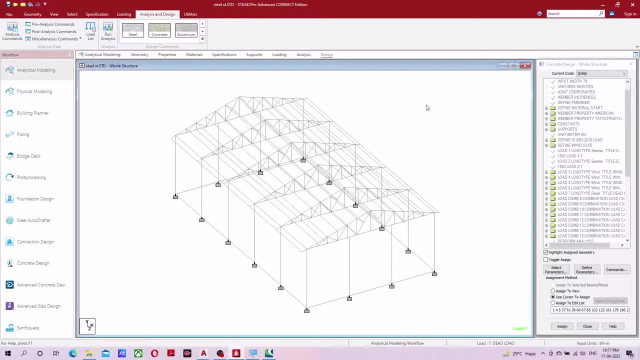 double click on the column here: concrete design: here my column is showing this column one and this column one. see here the result of the column. so like this you can design it completely. so this my design is done for now. pause the video for a while. after, pause, I completely. 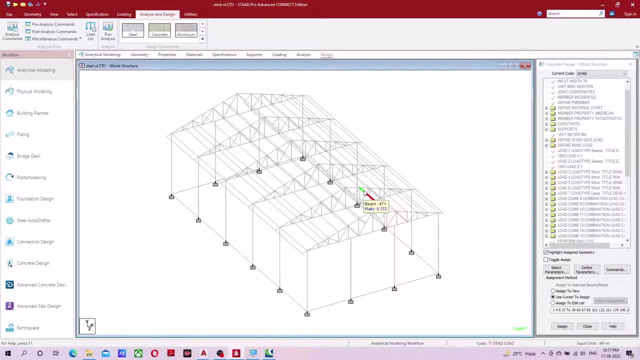 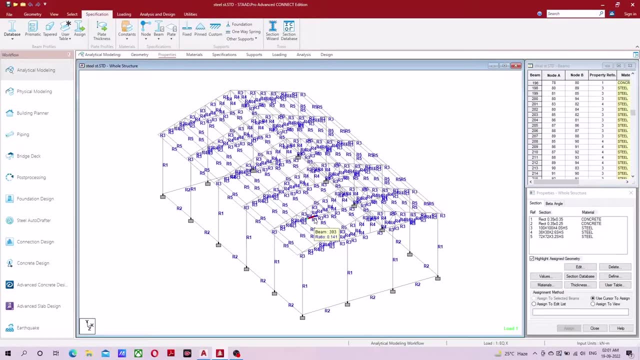 I draw it, because if I draw it online then I will take a lot of time, and after drawing it I will explain it a little. after that we will continue further. so after one day, one day, my drawing has been completed. so this drawing, according to the design, 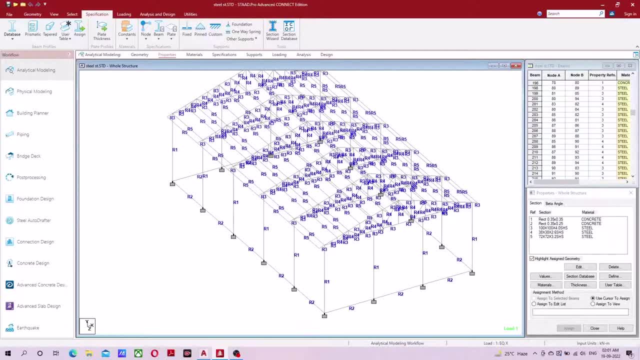 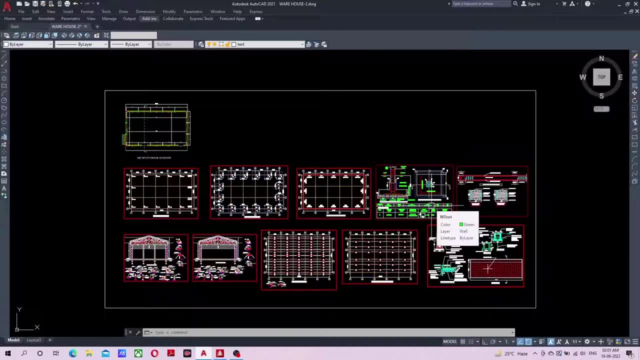 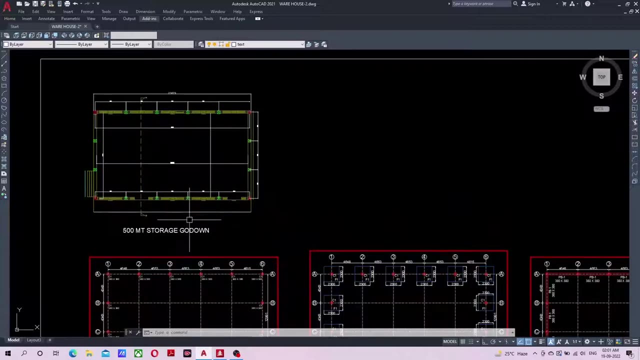 I have completed it according to the design. if we look at the drawing, then I have completed my drawing and, according to the design, I took 5 to 6 hours to complete it, which I am explaining. this is my plan. according to the plan, I have provided column position. 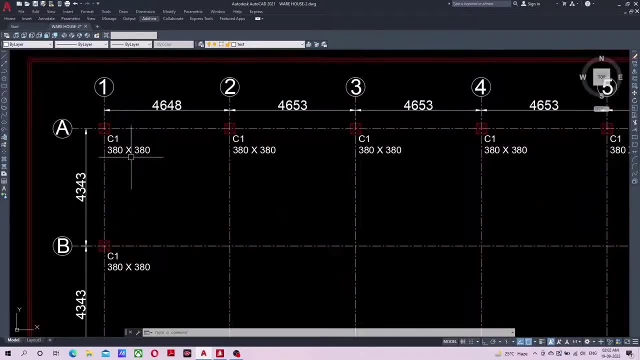 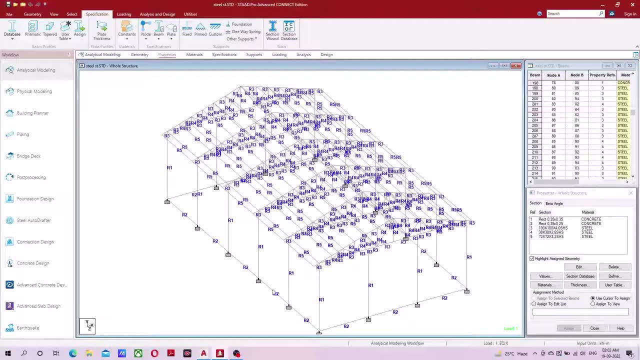 column layout plan. so the column was RCC column and the column I have given here is 380 by 380, but here exactly the pass is there. if I look at the column, then the column of 350 by 350 is passed here, but here I have provided. 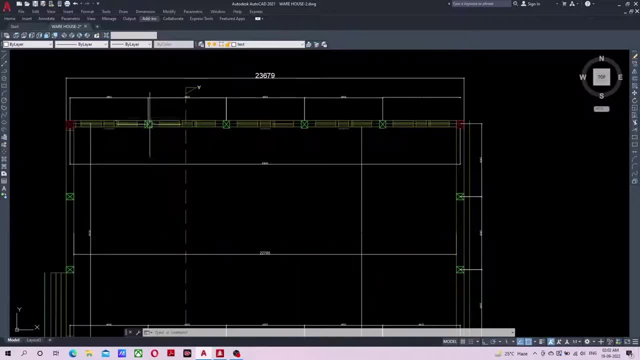 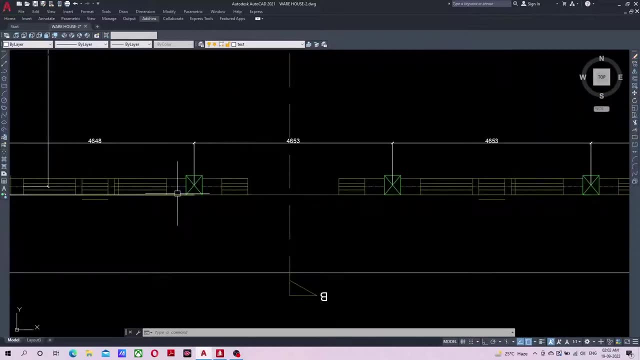 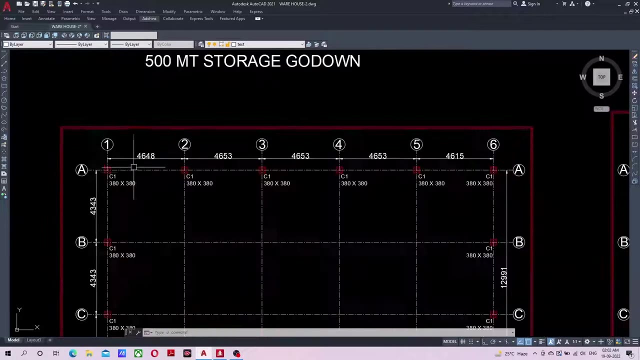 380. why 380? because the wall thickness is 380 mm. the thickness of the wall is 380 mm, so according to this, the thickness of the wall is the same as the size of the column. so that's why I have provided 380 mm column. 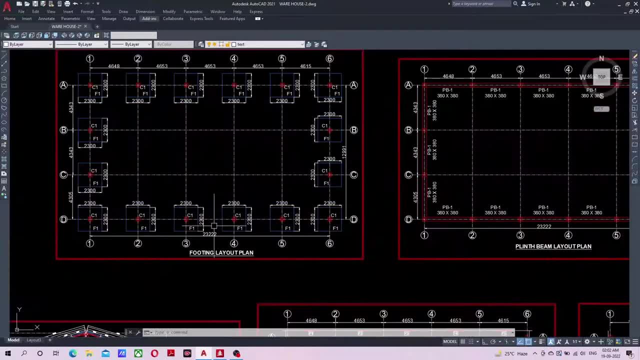 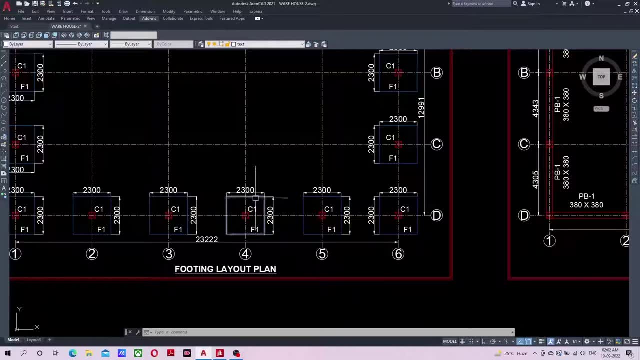 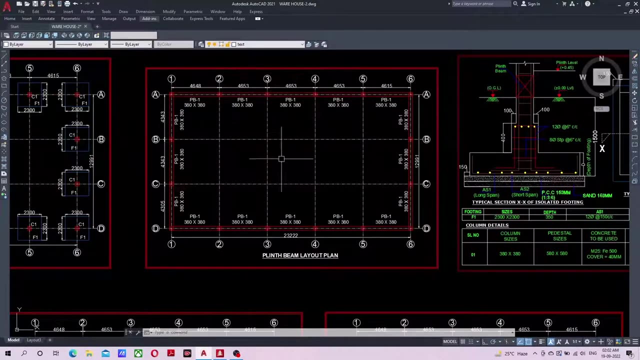 so here my column position is done. after that my footing size. I will upload the footing in the next video to calculate the footing. so the footing pass here is all around footing. after that the clean beam below: if the wall thickness is 380 mm, then the beam size. 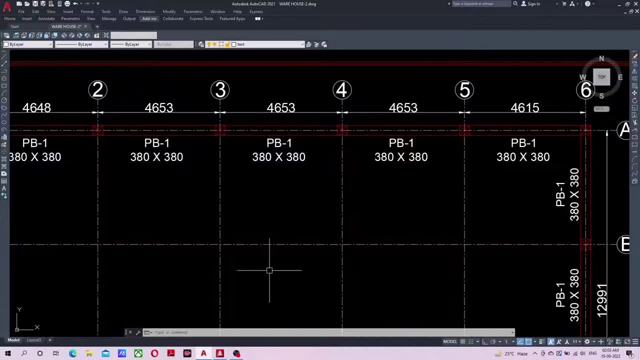 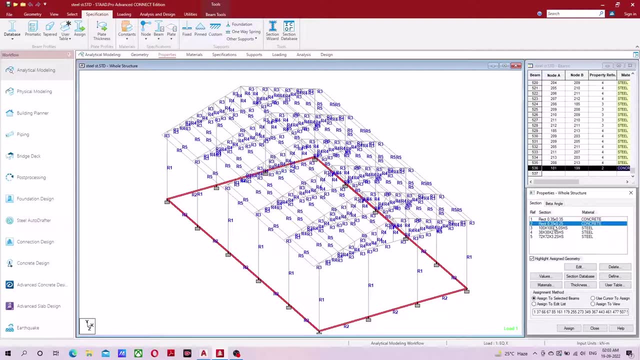 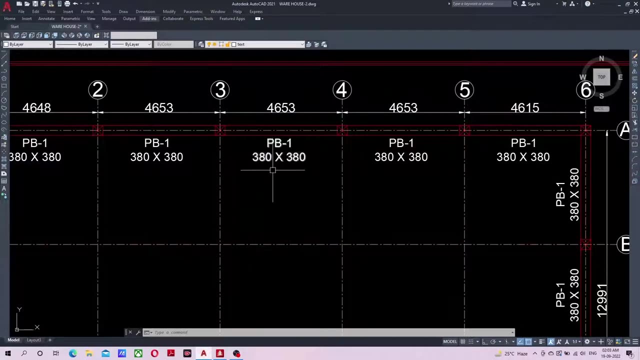 is also 380 mm into 380 mm, but here my pass is there. so, whatever the pass, you can take more, but don't take less. so here exactly pass is there: 350 by 250, but here I have provided according to wall thickness, there is no problem. 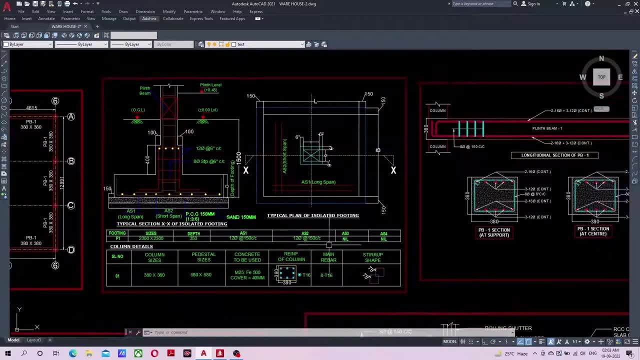 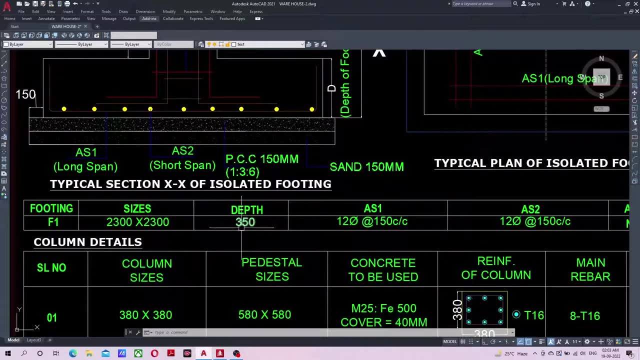 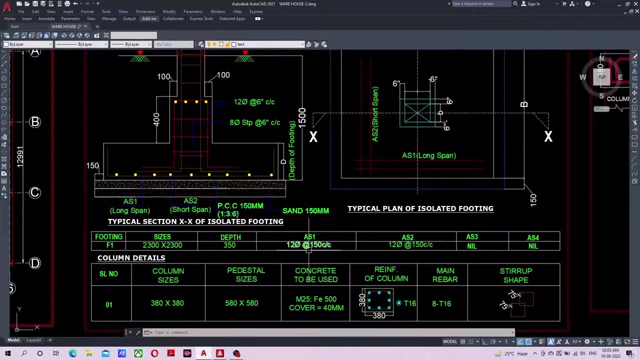 so this is my clean beam. after that, here is the detail of my footing. here, my footing will be the size of my footing- 2300- 2300- and depth, which is 350 mm, and the reinforcement bar will be used here. here the full detail is given. 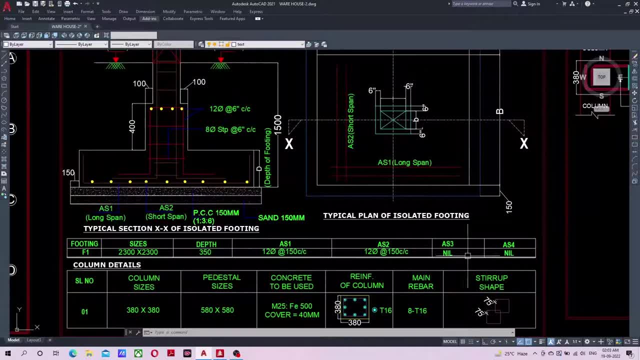 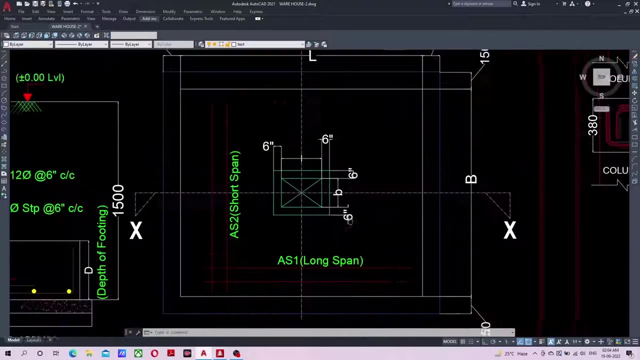 S1, S2. what is given here? S1, S2, S3, S4- there is no reinforcement bar in the top, only on the bottom, on both directions. the reinforcement bar of 12 mm- 150 mm will be provided here according to this, provided this is on inches. 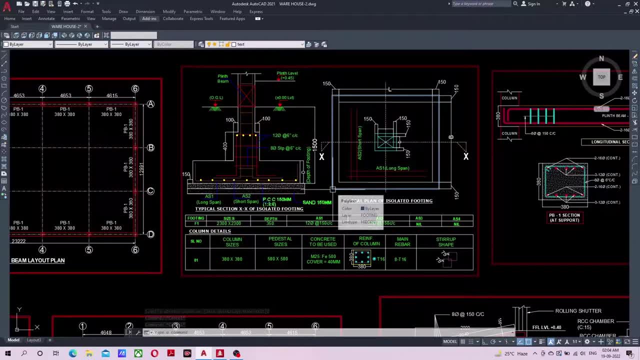 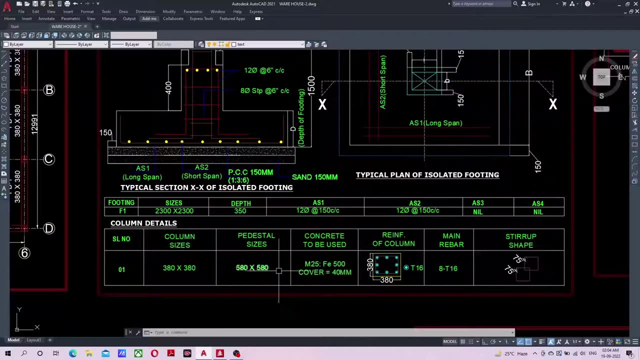 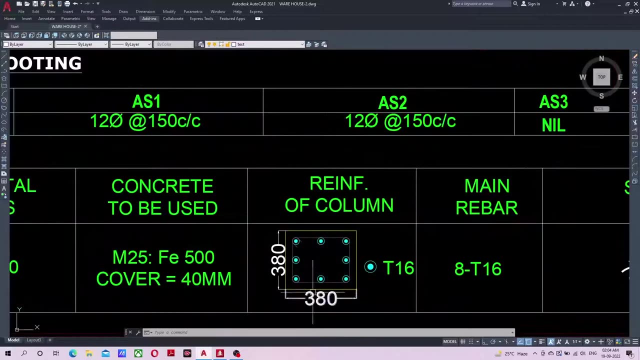 so here the full detail is given here. the full detail is given here. so you see the detail here. here you will get the full, like: here the column, the size of the column, and here the reinforcement will be your total 8 number of reinforcement bar of 16 mm diameter. 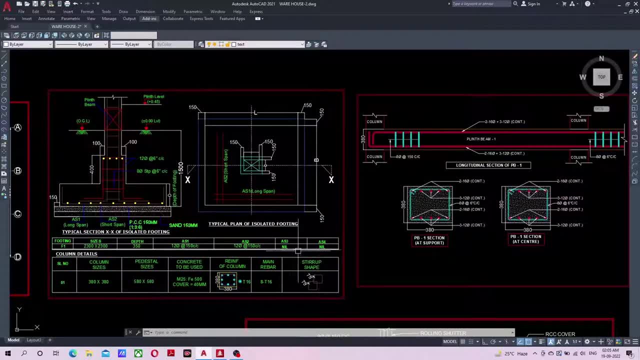 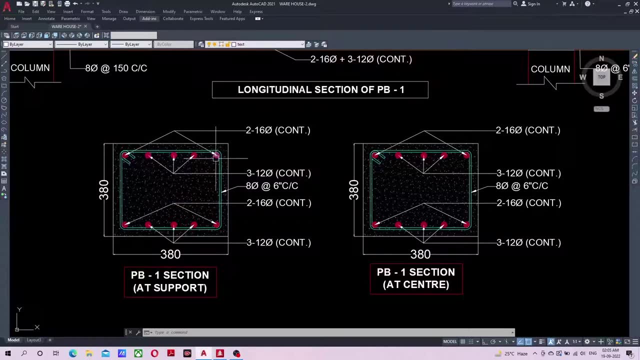 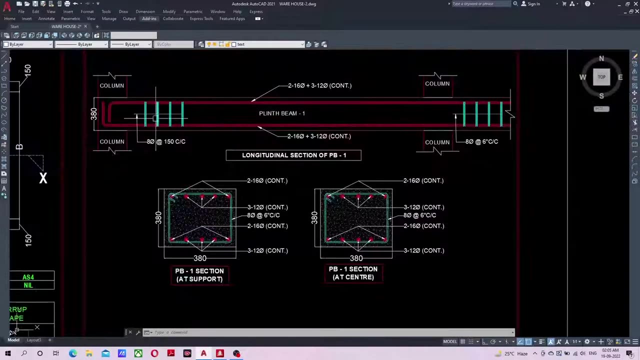 so this is the full detail of your column footing. after that, this is my clean beam. the clean beam will be 3D, in which the reinforcement bar will come in the top 216 and in the bottom 216 and in the middle, 312, 312 will be the continue bar. 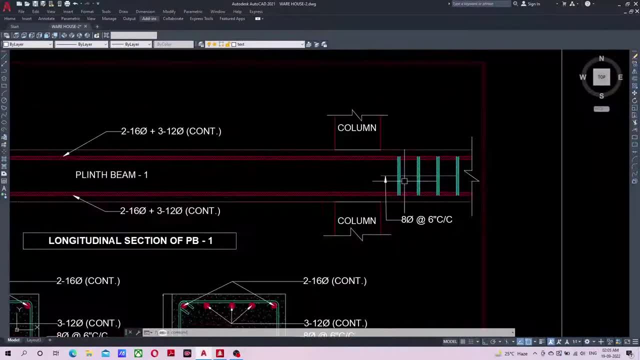 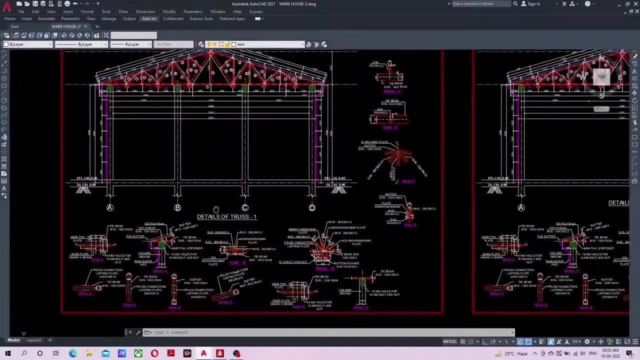 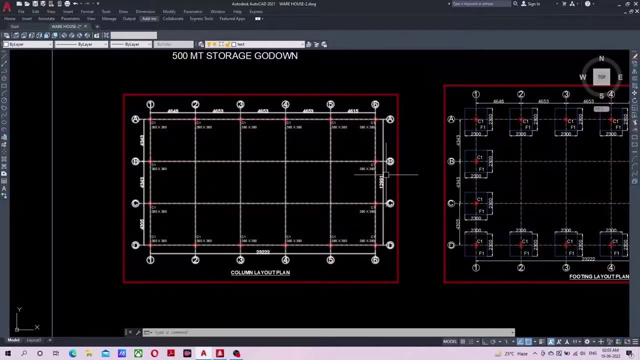 from starting to ending. so this was my reinforcement detailing, according to reinforcement detailing, the casting of the column. after that, here my detail of truss 1. so where is my truss 1? if we see so, this first and last one is my truss 1. 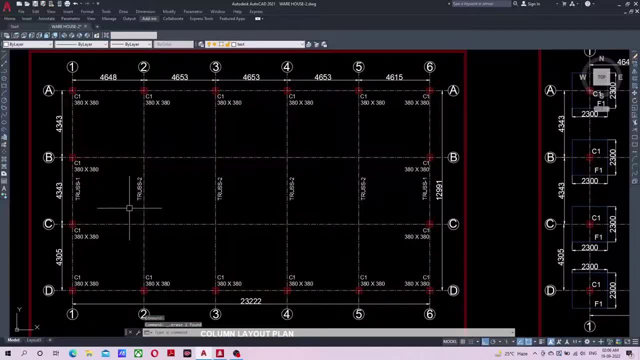 ok, if we see this diagram. so here I have mentioned this: truss 1, truss 1- this first and last one is truss 1 because truss 1 has 4 number of column. after that, in between, we consider this as truss 2. 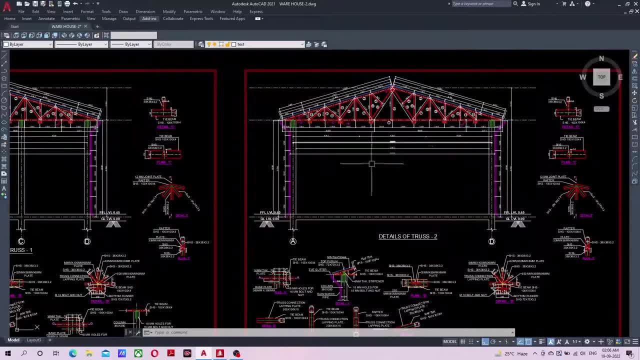 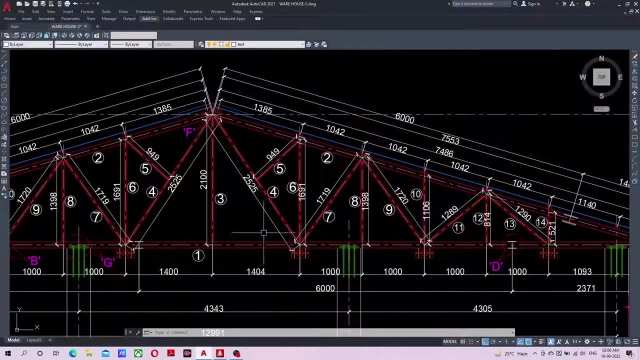 according to this, truss 1 has 4 column and truss 2 will be only 2 column here. so here the full detail of the column footing- sorry, the steel section, the full detail of it. has been explained that what will be the dimension, what will be the dimension? 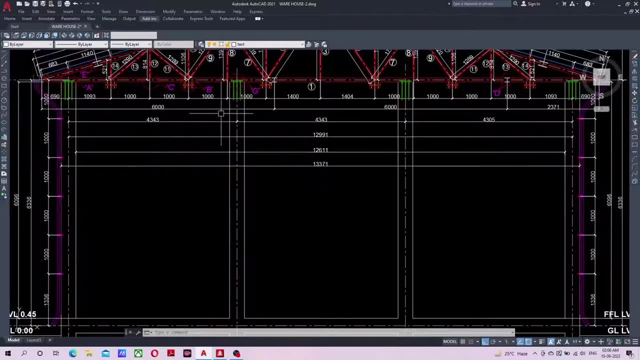 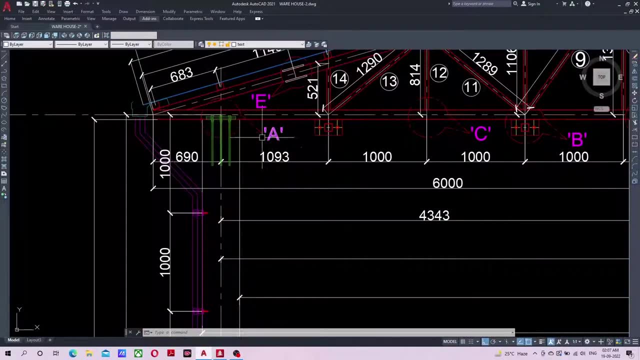 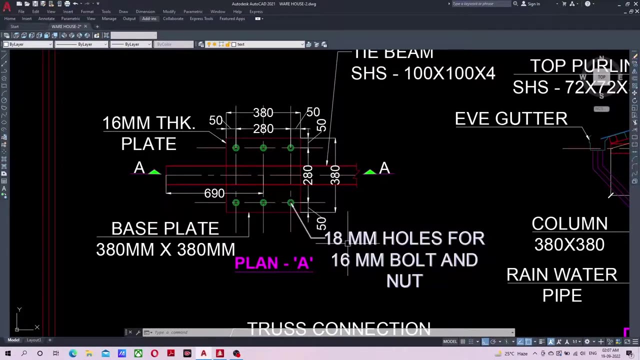 this whole thing is mentioned one by one. after that, the dimension is also mentioned. after that, the section will be like the first one. I say this in this part: what is your section? section of this? so the detail of this will be given here. how many mm will be the knot bolt?